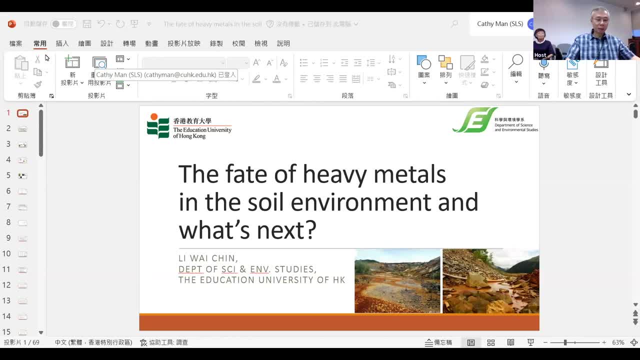 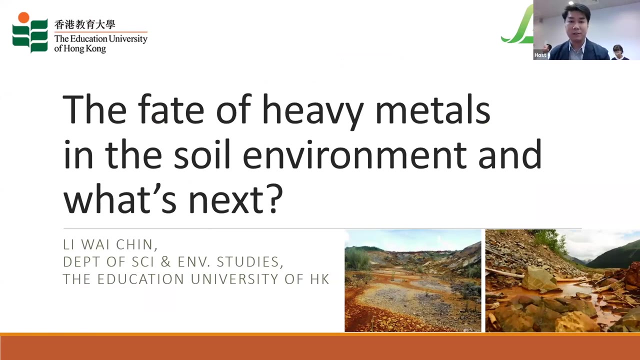 plant growth-promoting myelobacteria, biochar, foods and anatomical properties, etc. regarding the natural performance and heavy metal uptake in contaminated soils. So, without further ado, let's welcome Dr Li to the floor. Okay, Hello everyone, both physically and also in the internet. First of all, thank you so much. 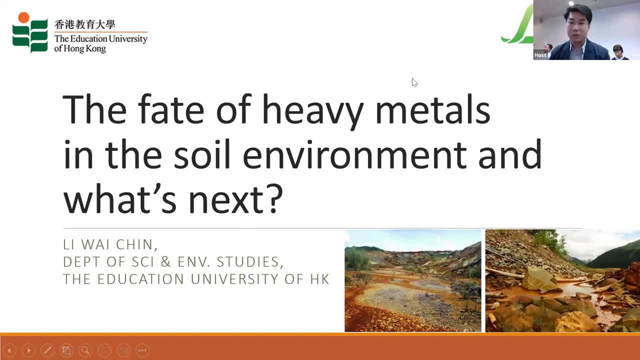 Professor Lam for your kind introduction. okay, And as this is from actual Hong Kong, let me introduce a little bit. Actual Hong Kong now is not just for training teachers, because we also offer supplementary programs. For example, my department, Department of Science and Heavy Metal Studies, we also offer a Bachelor of Science. 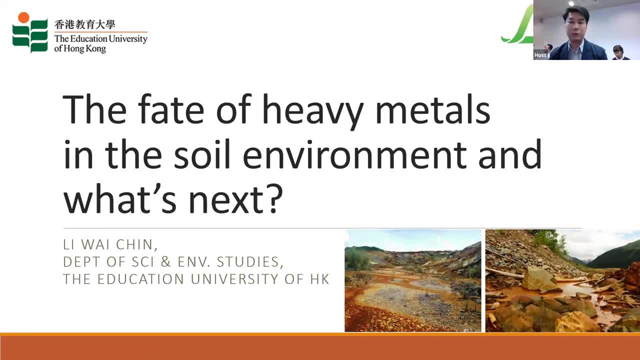 program in Integrated Heavy Metal Studies, Integrated Heavy Metal Management, And we also focus on sustainability and also some STEM education. Here is some background of the place that I'm working And now let's take a look. okay, As you can see the title. 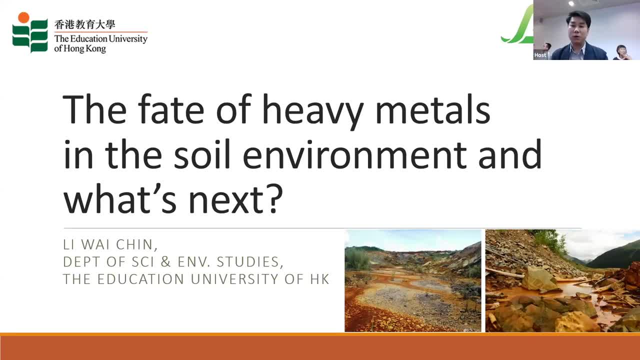 we focus on the thing of heavy metal, As you may all know that in our environment we have so many kinds of pollutants. There are, of course, organic one, non-organic one. okay, And now I will only focus on heavy metal and see how this is actually working: running, operating, uptaking, whatever. 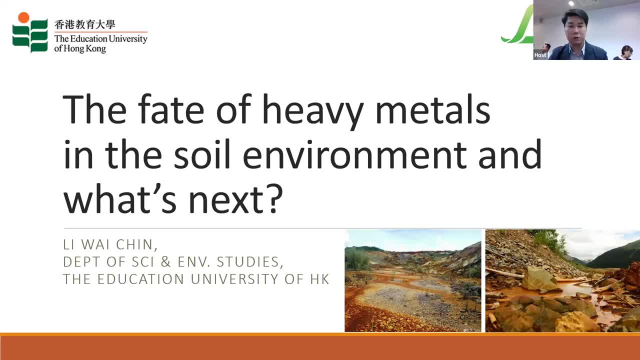 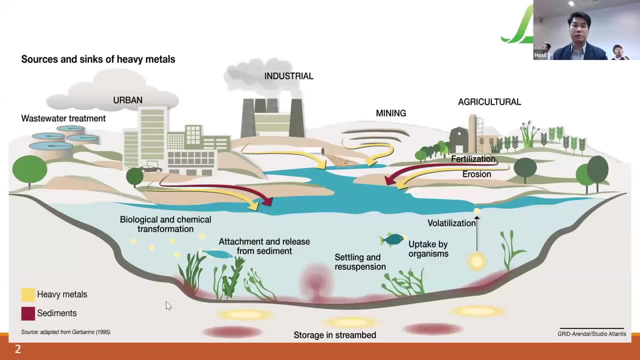 in the soil environment And let's also think about how could we handle that kind of pollutants backdives in the environment. Okay, as I mentioned, there are different sources of pollution, just like in the soil environment. There are different sources of pollution, just like in the soil. 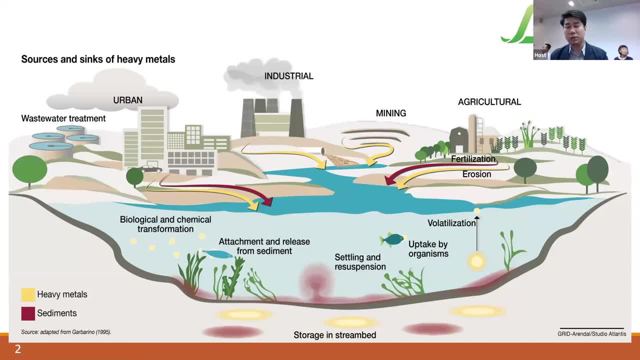 environment. There are different sources of pollution, just like in the soil environment, As you may aware that some kinds of low-quality fertilizer actually contains quite a lot of pollutants of heavy metal, And, for my part, my research mainly focuses on mining activities. 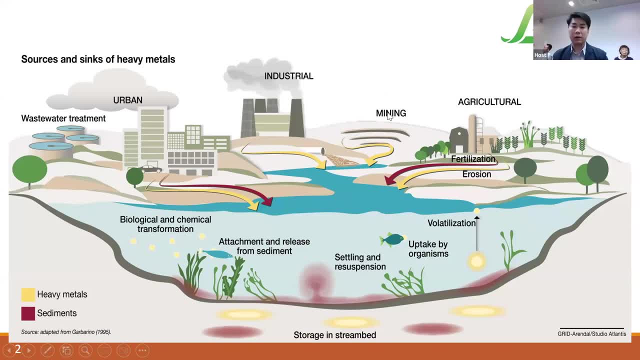 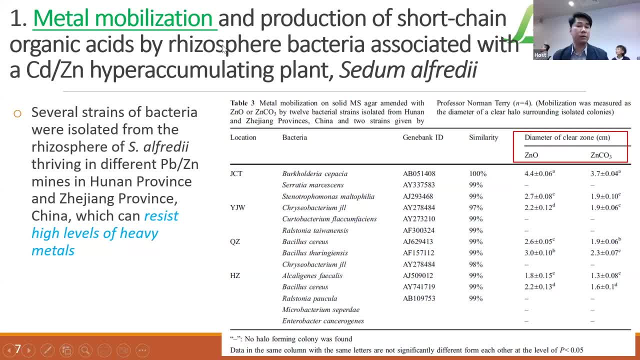 know. there are different sources of pollution, As you may know. there are different sources of pollution, As you may. the rhizospheric bacteria, the same. these are something nice, okay, not bad guys, because they're living with the plant and of course they might have some mutualistic activities. so i try to 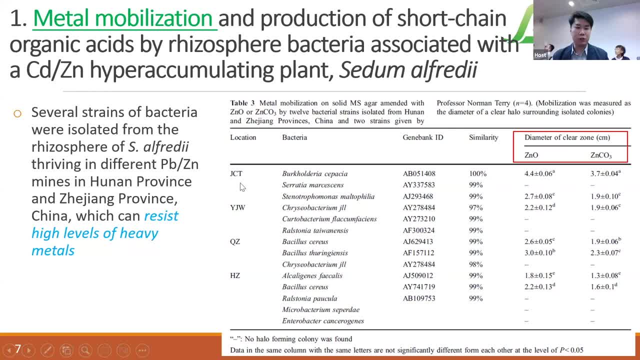 visit different farm, uh in hunan, in zhejiang province, and then we isolated different bacteria. okay, and let's see, okay, we try to inoculate the bacteria with- okay, just on the agar plate, for example, with the zinc oxide, zinc carbonate. if you know something about chemistry, you will be aware. 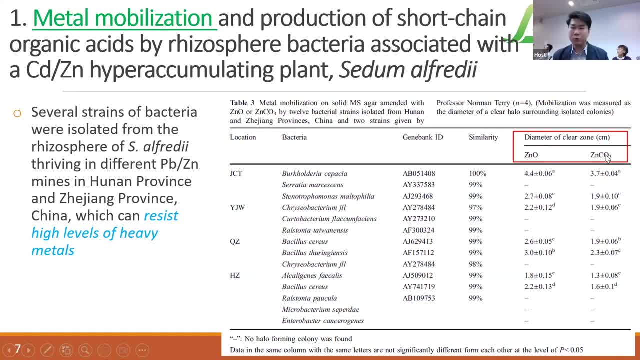 that this kind of oxide carbonate. they are fully soluble. this mean not soluble. when we put this zinc oxide, zinc carbonate in the agar plate, they did not. they did not. they did not dissolve. they somehow use the form as a powder, some white box on the agar plate. and, interestingly, when we 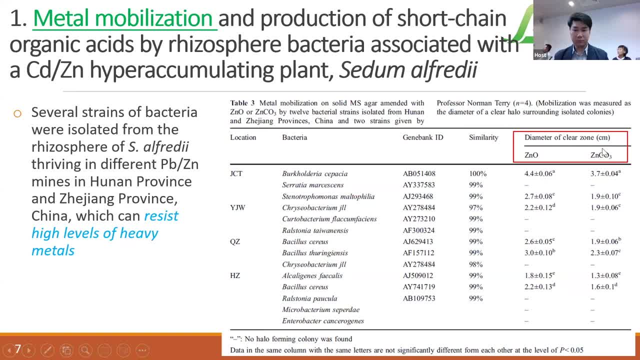 inoculate bacteria with these zinc oxide, zinc carbonate. after a few days we found that some clear zone, some clear zone on the agar plate. somehow this actually means that this kind of zinc oxide, zinc carbonate, they are being dissolved- okay, dissolved and become available. become available. and this give us some insights to see. oh, how come this interesting? 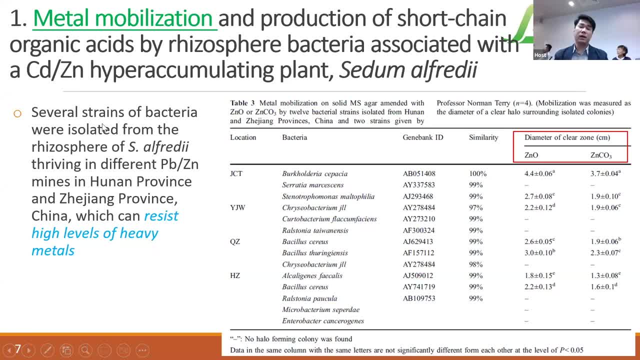 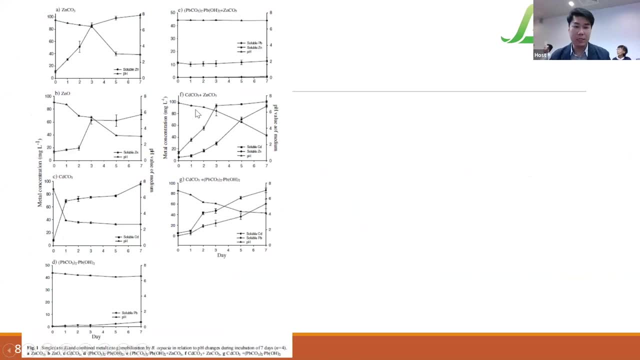 bacteria can work with the hyper accumulator and, of course, eventually found that they this this kind of bacteria. they release organic acids and these organic acids assist the mobilization of the heavy metal. and here shows we tried to inactive the bacteria with different kind of heavy metal, including cadmium. insoluble cadmium forms such as just like the. 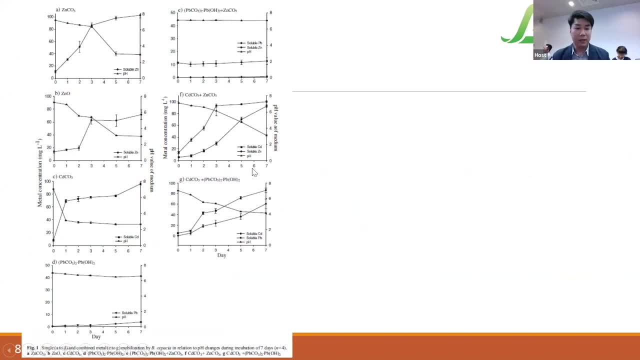 cadmium carbonate, zinc oxide, lead carbonate, that hydroxide, so and so forth, and what we found is most of the heavy metal compound. they are also being mobilized, okay, mobilized. at the same time, we found the ph drop- okay, fish drop- to around three to four. 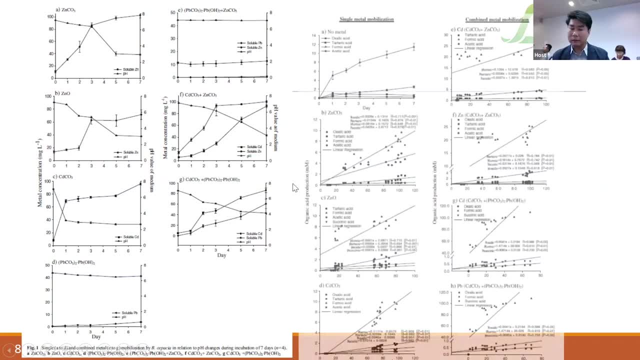 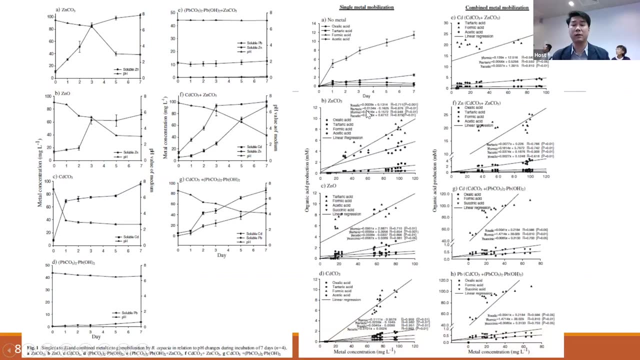 and we take another investigation: why the ph drop? okay, and luckily, we found that, oh, these compounds are the organic acid. okay, organic acid, they are the tetra acid. so in organic, uh, the thoracic acid, forming acid, so and so forth, and this mobilization of the half metal, as well as the organic acid. 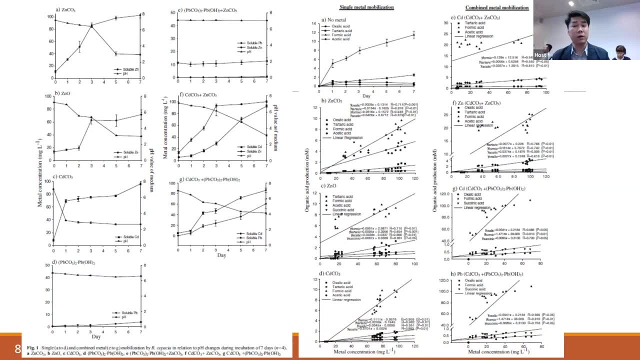 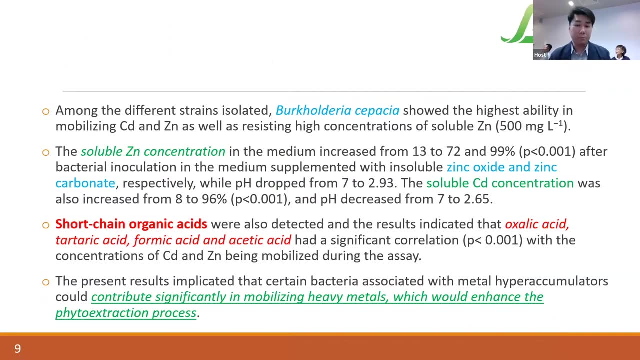 release actually form a very, uh, positive correlations so that we propose that this chain organic acid release, are the bacteria actually doing a conducive effects to the hyper accumulator, so that it could not just protect the plant itself but at the same time it can mobilize the metal and enhance the fire extraction efficiency? 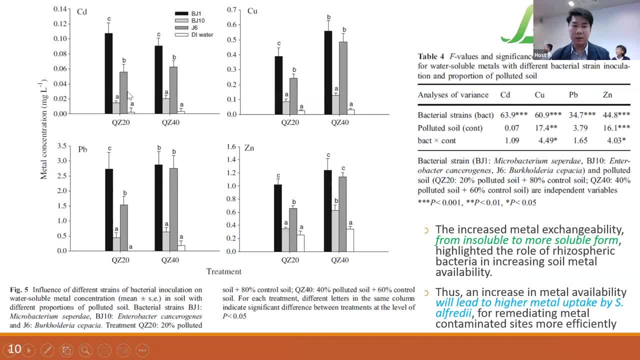 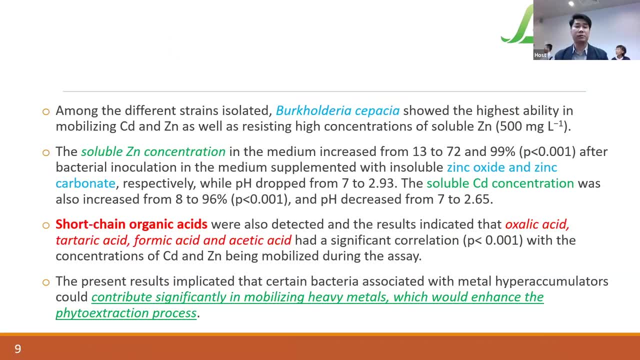 and we also try to inoculate the bacteria in a real soil, because in the previous part we mainly work in a, in a hydroponic solution, because, uh, it is a little bit defective, so to extract the organic acid from the soil conduction. so that this part of the research. 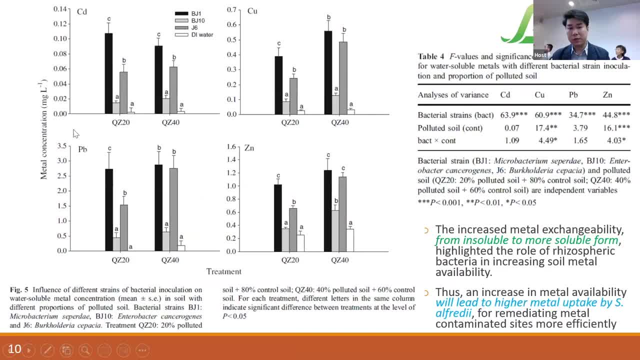 mainly done in a hydroponic solution, but we also try to inoculate the bacteria with the with different types of uh polluted soil- okay, with green concentration as well, and with the two and nova uh analysis we found the major effects, basically, which is caused by the bacterial strain instead of the soil, so it is actually further proof that bacteria is acting. it's 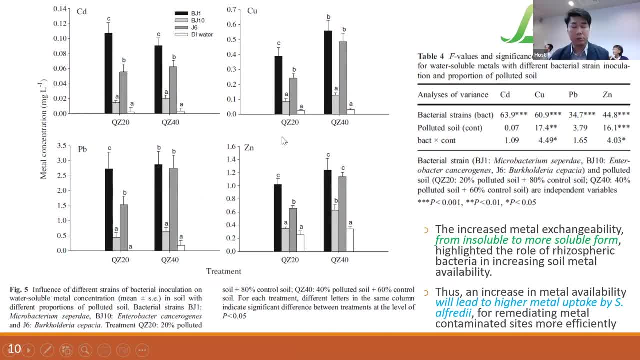 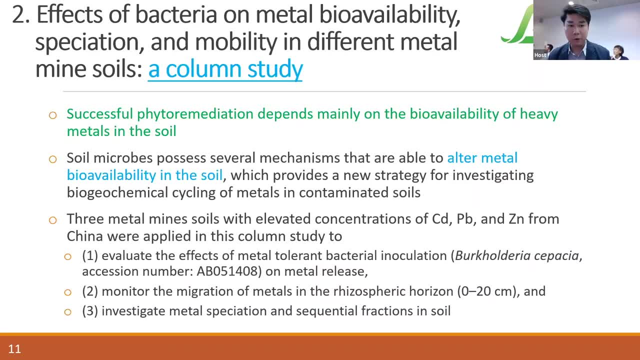 actually working very well in mobilizing the pollutants in the soil and also in the water connections, and of course we didn't stop. we also, uh, tried to inoculate the bacteria in a real soil condition, okay, and then we mimic a soil column as a soil column and, of course, the soil which 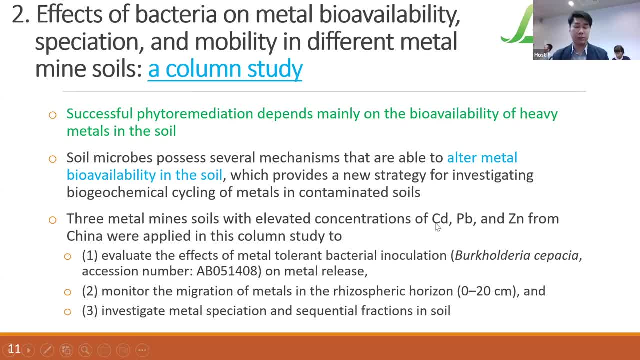 is come from an authentic contaminated soil, okay, which contain cadmium, lead zinc, so and so forth, and we also visited the lab to see if there's any other problems with that. so we've also found that we have a very good mixture of the two and the result is very straight. we found that solubility. 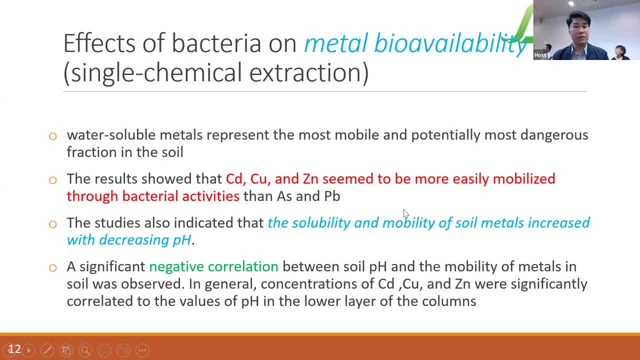 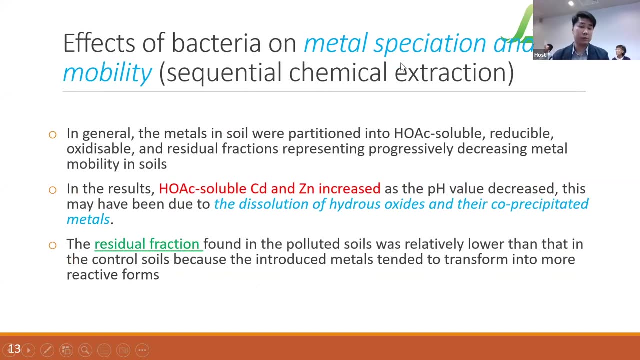 and mobility of these metals increased significantly, as well as with some dh drop a little bit, which is a very nice negative correlation. at the same time, besides the single chemical extraction, we also consider a sequential chemical extraction to see the metal speciation as well as the the composition of the chemical extractions, uh the formation of the chemical. 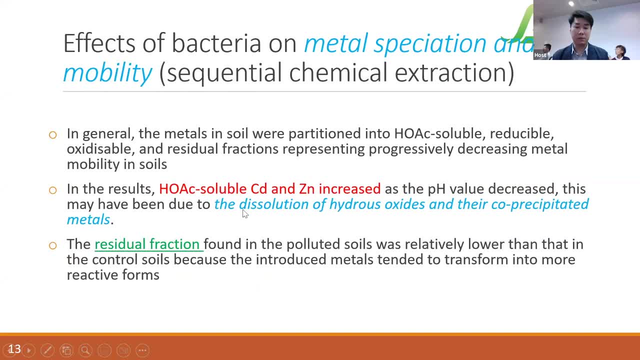 as the mobility and of course, we found that, yeah, the the solution of hydroxide hydroxides and also their precipitated metal also increased as well. and what we found is the residual fraction, okay, which is at a very low okay, not very, it's a relative low okay, away compared to the control. 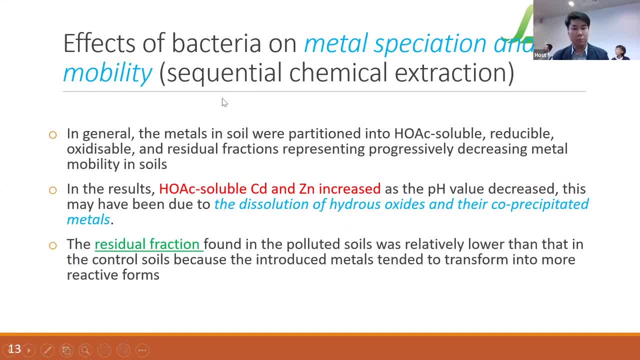 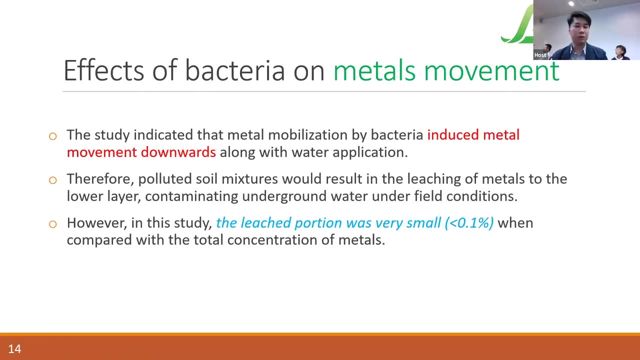 that's mean, uh, the material actually did a good work in mobilizing most of the heavy metal. of course we work on this uh, soil column. the aim is to mobilize and also enhance the fire distraction. but we also worry about it with the bacteria, i mean with the metals goes down. okay, right, we we. 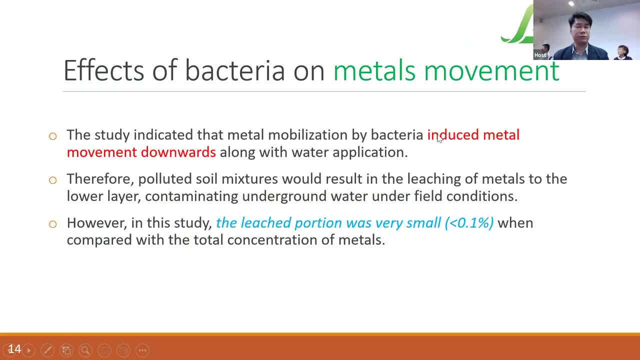 found the. the bacteria somehow mobilized the metal and with the gravity you can see somehow it induced the metal movement downwards. that's mean you may consider it might cause secondary pollution. but actually the leach portion is rather small when we compare to some uh chemical, okay, some leaching chemical just like epa, so and so 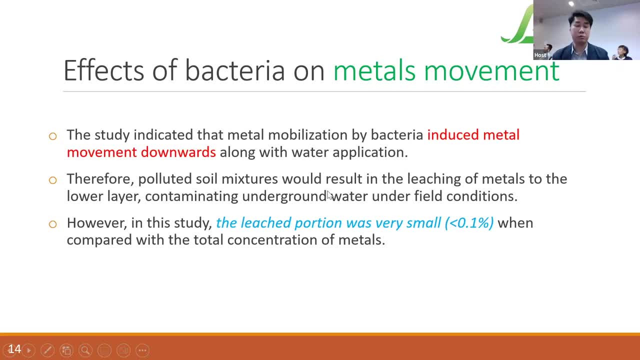 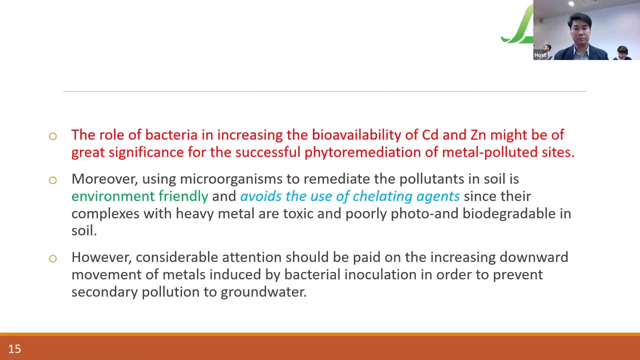 forth the effects is rather somehow under our control. so that's, although it somehow induced metal, uh, induced metal downward movement, but it's actually safe. it's actually safe because, suppose, the plant should have enough time to uptake it before it goes down further. okay, so that, uh, we, we will say that with using this kind of bacteria, 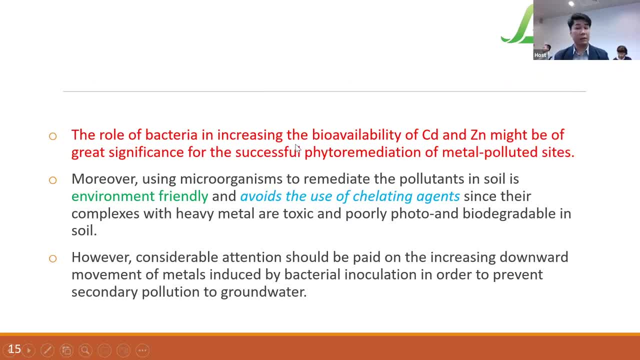 will be a nice solution, okay in cleaning up the pollutant. at the same time, it will not cause any severe secondary pollution to the downwards, just like the underground water river, so and so forth. so we will say: this is implemented for any technique at all days, okay. 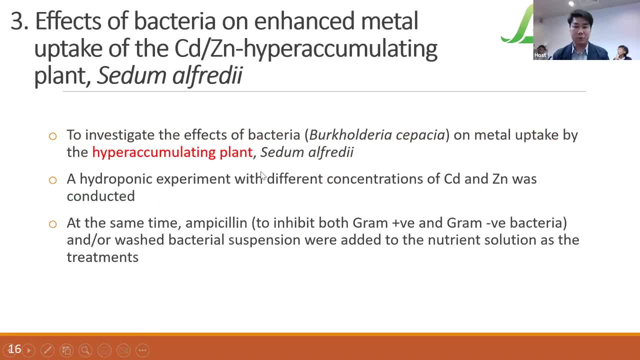 all days and, of course, uh, we will try to inoculate the material: okay with the plan, okay in the real conduction, and to prove the work is actually done by our bacteria. with the whole one of the control. we try to add an emphasis, which is antibiotics, a very strong antibiotics. 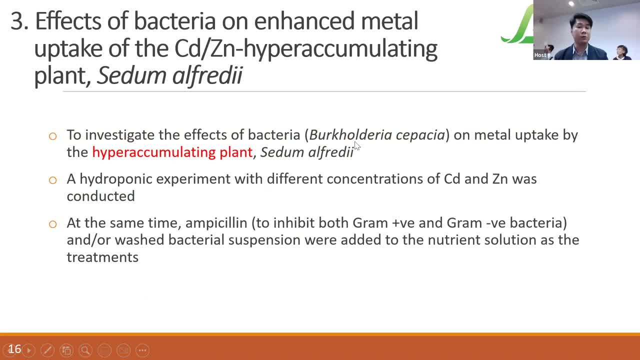 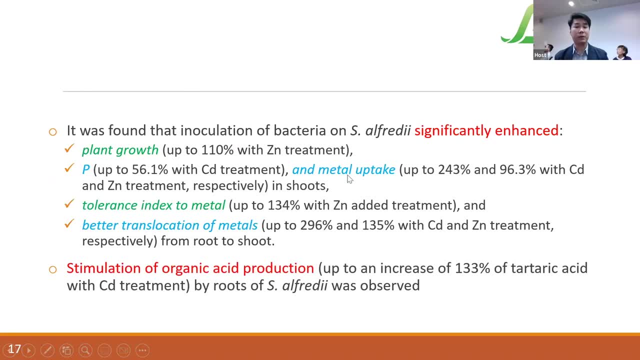 to kill, to inhibit all the bacteria, including ours one, so as to uh, ensure this is a control. and what we found is okay, of course, the metal up increase. at the same time, we found the plant growth also increased, nutrient uptake also increased, as well as the tolerant index of. 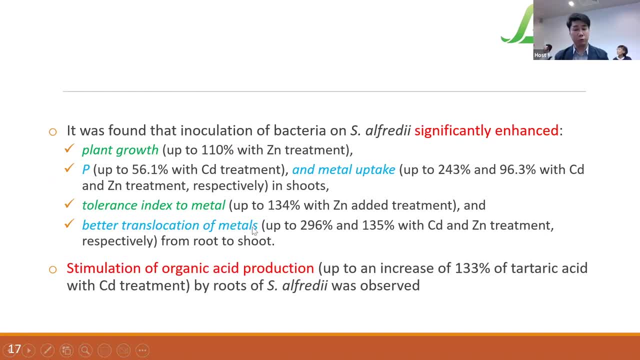 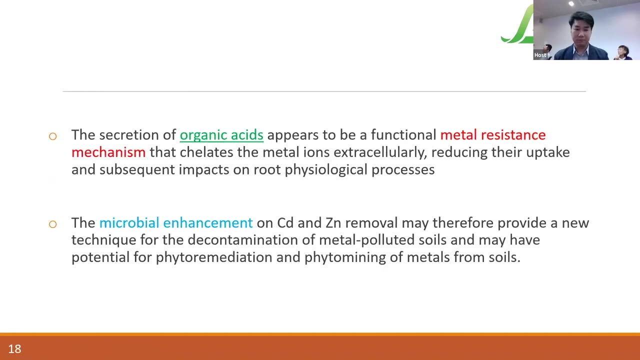 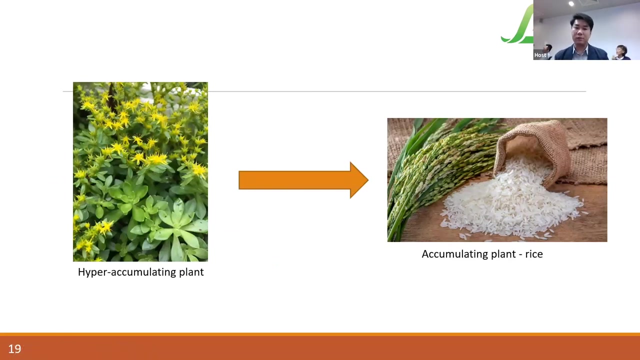 the metal and also transportation of the metal okay, from the root tissue. it is also significant it be improved, okay, by the stimulation of organic acid reductions. so this is a very nice material working very well mutualistically with this hyper accumulating class, okay. so, um, this is just a very quick introduction and, as i mentioned, if we keep using 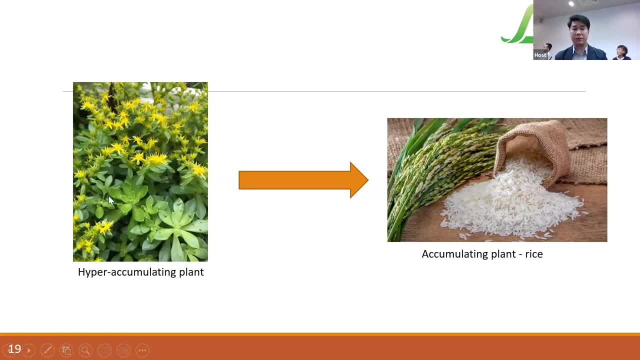 this hyper accumulating plant that the problem is. basically all the activities, farming activities should be stopped. they stopped this for a few years at least, before the soil is ready for farming, for agriculture. but as a farmer, just like a rice farmer, i think they can't wait. they can't wait if they stop all these agricultural practices. i think they cannot. 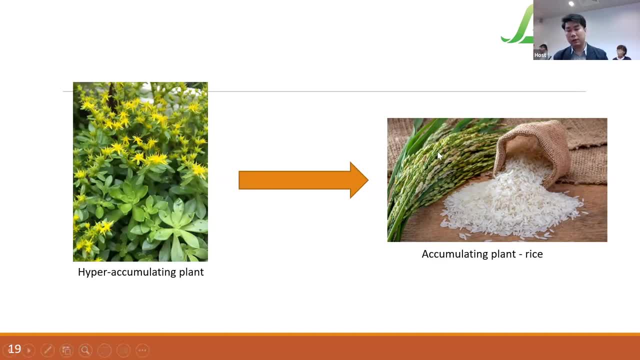 support their well-being. so once i joined it- um, actually hong kong- i tried to use another perspective. okay, how the farmer would think: would they adopt our technology if we, if we are still using the hyper accumulating plants? i would say, if i were, if i were the farmer, i won't adopt it. 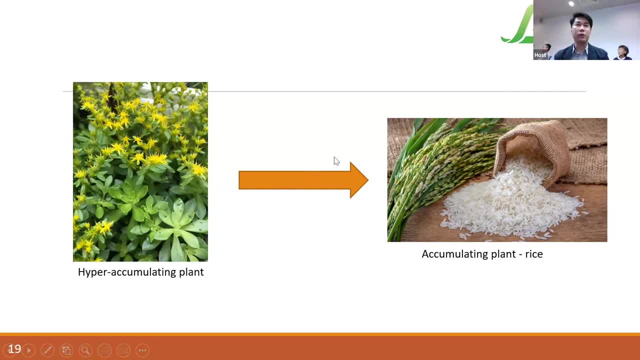 i won't adopt it. so, um, what could we do? okay, let's see in the third, in the, in the latest slide, and before we come to the rise, okay, i think, rise. you guys, we know it very well. okay, as a chinese, we eat rice every day. okay, basically, around half of the population in the world they will eat rice. 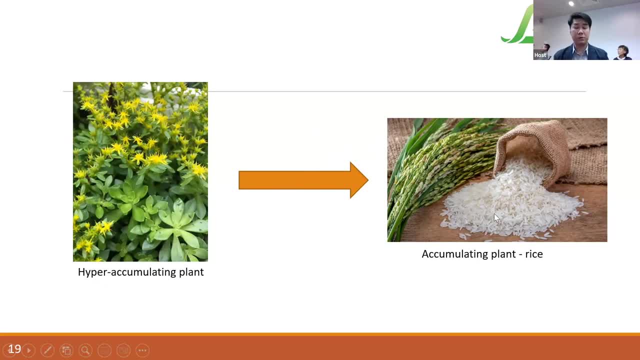 or or related products. okay, every day. so, but i think using the hyper accumulating plant will help. you may not be aware that rice is also a metal accumulating plants. okay, where would this metal be accumulated in the rice? they are not in the roots. no, they are not in the stem. they are also. 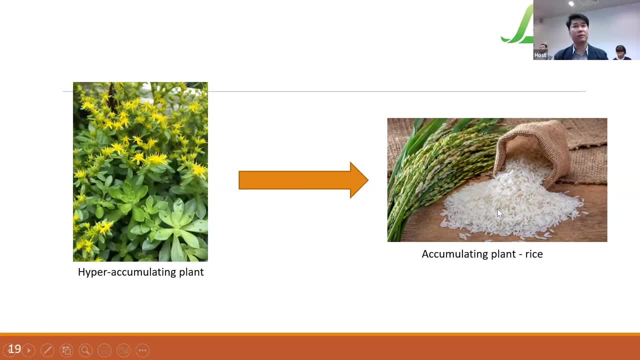 not in the husk, rather in the right screen. okay, in the right screen. so that, oh, this is a problem, is a headache to most of us. but in hong kong, as we found that most of the rice, basically, are imported from thailand, from vietnam, and so far we found these uh products, i would say, pretty nice. it's. 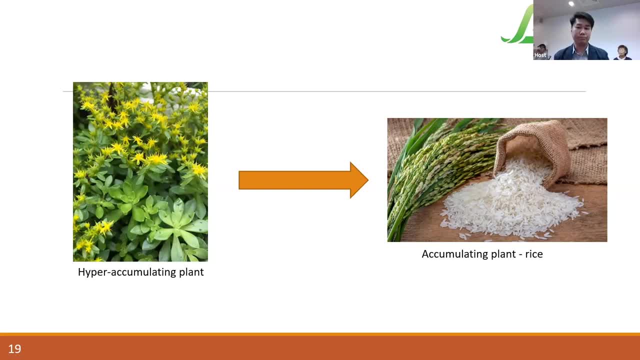 safe. it's safe, but unfortunately we found some rice product which is import in china. i don't know the source, but in the newspaper you can find that talking about um 40, 40 of the rice product from the market. okay in hong kong, okay in hong kong, if, of course, if they mention that the right. 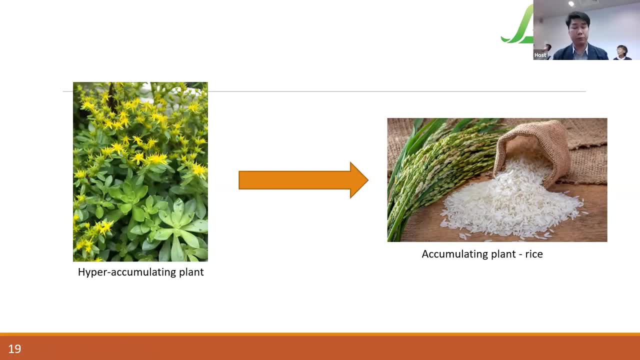 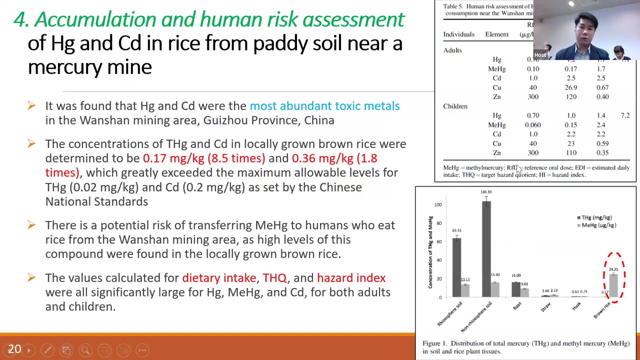 in china, 40 of them are polluted, 40 is a very high number- by cadmium, by lead, so and so forth. so there's somehow we have to pay attention. how can we solve this problem? because we have to eat every day, so, uh, i have to. i have, with this, different uh, farmland. okay, in china, in china. 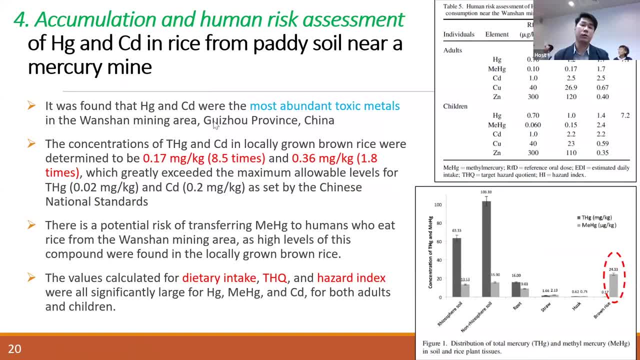 and this one is in guizhou. okay, in guizhou, which is near in mercury and cadmium site, right, a mercury and cadmium site, and unfortunately we found that there are mercury, neva, mercury, cadmium and different kinds of heavy metals, or in the rice. 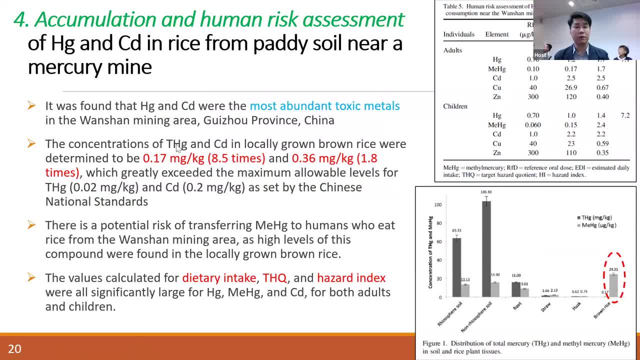 products: okay, for example, for the total mercury, which is 8.5 times exceeding the safety guideline, and for the cadmium, which is talking about 1.8 times exceeding the safety guideline, and we try to put input this data okay and to estimate some human health risk assessment. and for the total hazard portion: okay, normally. 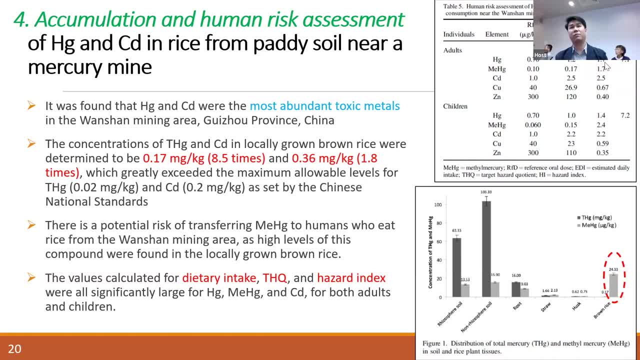 when we take a look on the paper, they will only focus on one: heavy metal. actually, in the real production, i think, in the soil, most of the sites, frankly speaking, they are multi, okay, multi-polluted by various kinds of pollutants and we try to input: okay, only, this is only three. okay, i didn't. 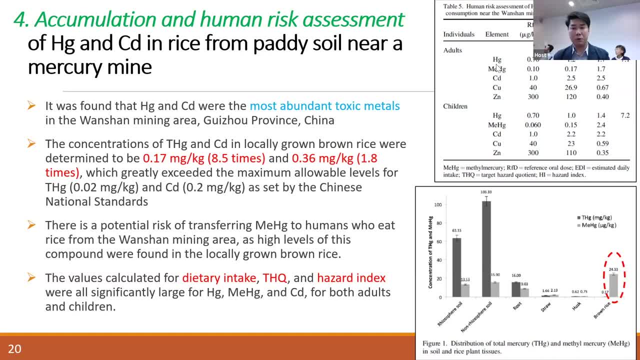 i didn't analyze all, but by just these three: mercury, neva, mercury, neva, mercury, which is the uh, the toxic form, most toxic forms of mercury in the, in the as a mercury type, atmium, and what we found is even just mercury itself is 1.7. what does this? 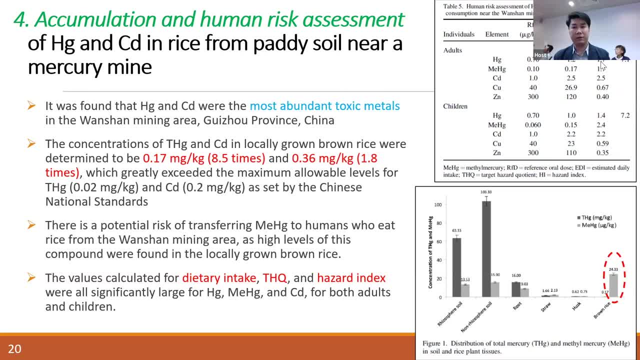 mean if this is higher than one then maybe have a very high risk of some pasta, okay, some hustle. so by mercury is 1.7 neva mercury 1.7 for cadmium 2.5. so hi is a health index which is the accumulative. 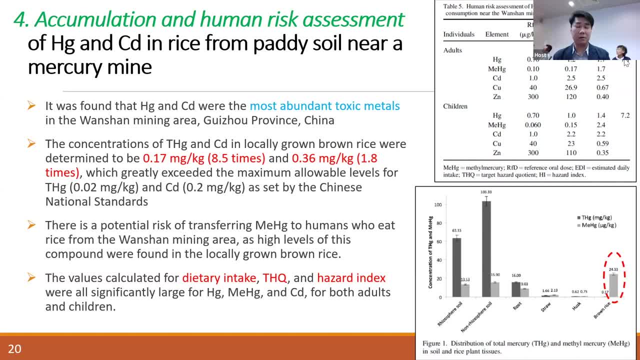 name. if this is higher than one, that means there's also some uh high risk of different classic effects. so by just this one metal, mine, okay, we find that the human, human health risk assessment is actually providing a very alarming result, okay, alarming results in china, and i think there are quite a lot of similar conditions, not just in white job, but also in 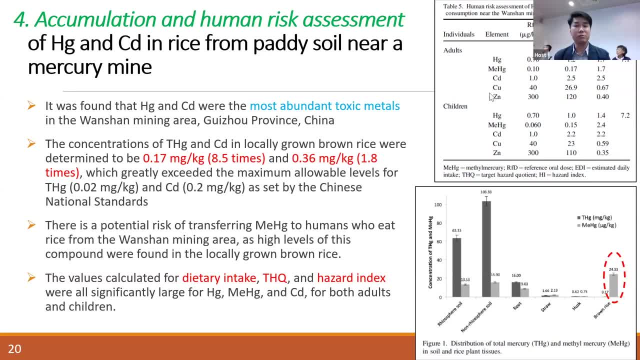 other profits, and not just for adult, but also for children. okay, the condition is very similar, and we also found in the brown rice, okay, most of the mercury that actually exists in the meat, from moving form that is, as what i just mentioned is the most toxic form. so that's why, uh, is this out of our 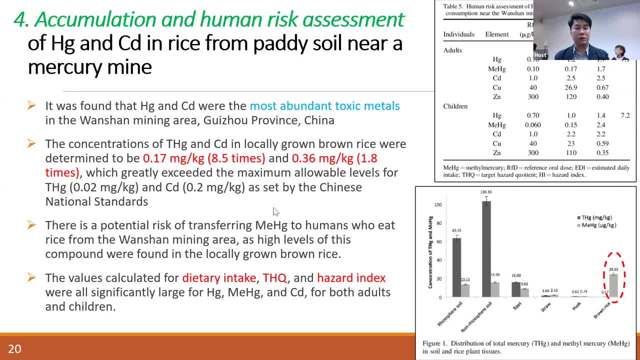 expectation and, of course, uh, we interfere or somehow. if we have a casual chart with the farmer, okay, and we ask them: okay, how would you handle this right? would you consume them? and, frank is speaking, the farmer say they didn't eat. but they will sell them to the other district, not their own district. 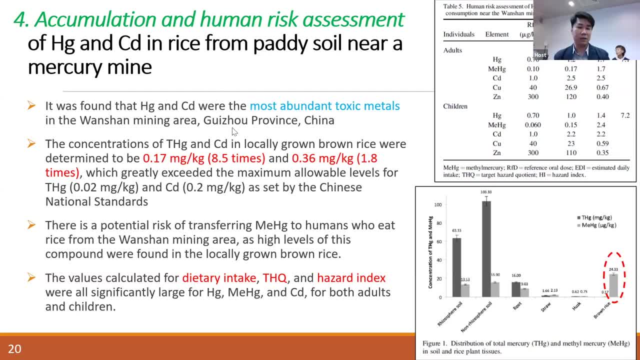 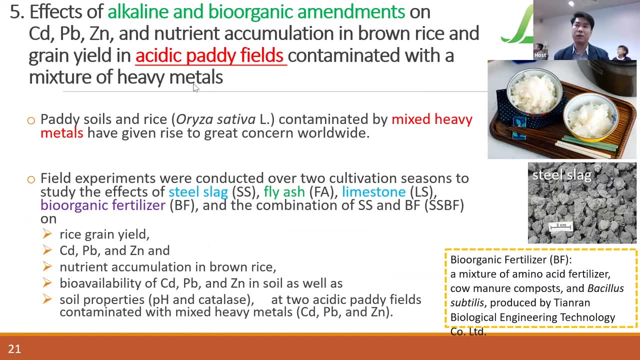 not their own town, because without selling this ride they cannot support their well-being. so i think the farmer should have a certain perception of the quality of the rice, but somehow they can do nothing. they can do nothing in this case. uh, with this concept bearing mind, we're trying to help the farmer. can we allow? 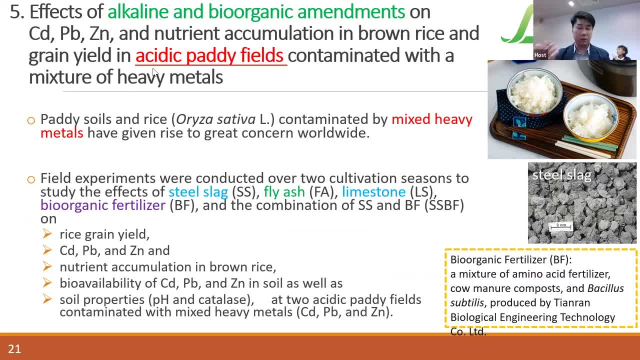 them to grow the rice at the same time, but i mean in a contaminated site. okay, instead of stop all the activity and clean up first, because clean up first is impossible, as i mentioned, they have to wait several years. but now, uh, we tried to locate, identify some, um, acidic battlefield, okay, acid, 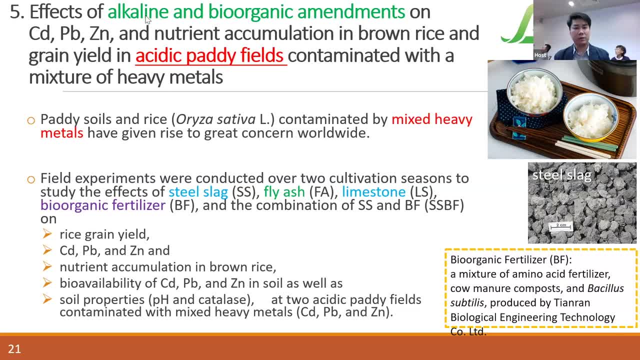 battlefield in china and we found, if it is possible to use some agriculture rescue or some industrial byproduct, just like steel slab, which is a byproduct from the stainless steel factory, uh, five ash, okay, limestone, i think you guys know it very well- and also bio, organic. 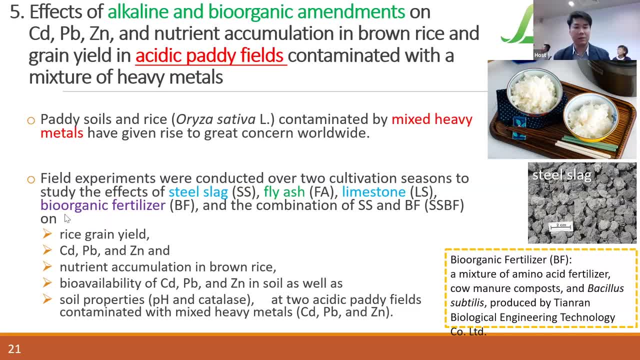 fertilizer which is a very famous and common fertilizer to be adopted by the farmer in china, and i have a check- this kind of bio organic fertilizer which, including some amino acid fertilizer, some cow manure compost, as well as base sitters, bacteria- right, we try to compare. okay, if this kind of alkaline or even bio organic amendment could. 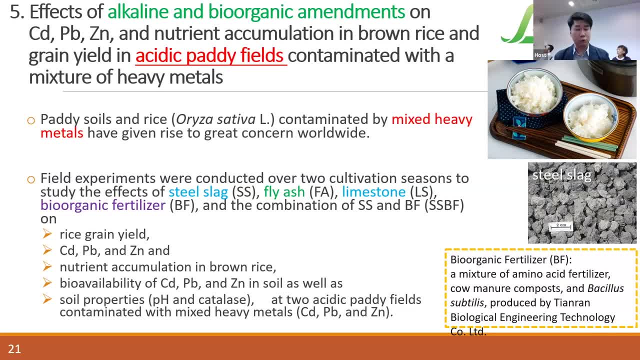 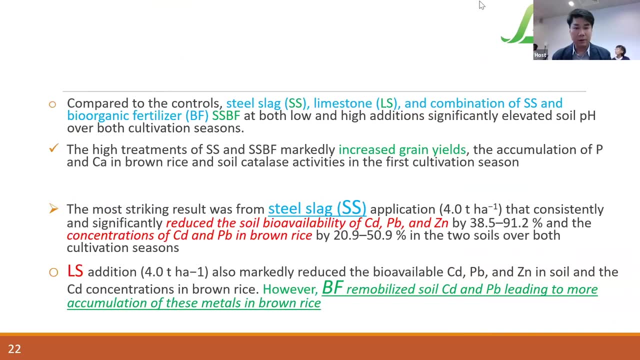 assist, okay, the farmer. of course, the aim is to reduce the uptake, so let's see if they could solve the problem. we focus on cadmium, lead and also zinc and, of course, more important, the rice grain yield and in general, we found that, uh for the- let me see, for this- steel slab, okay. 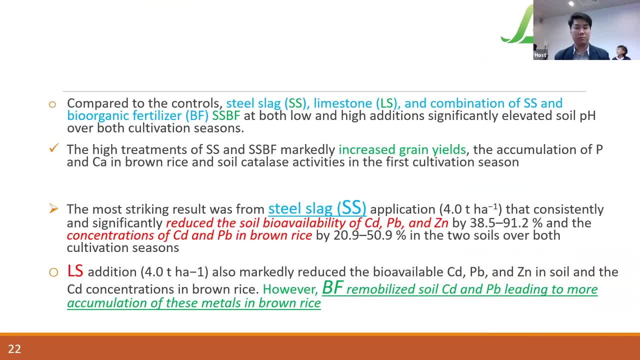 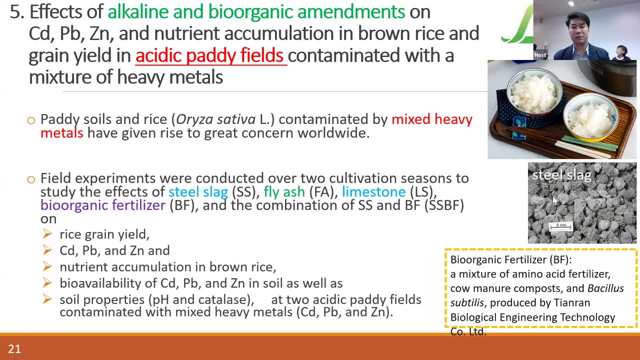 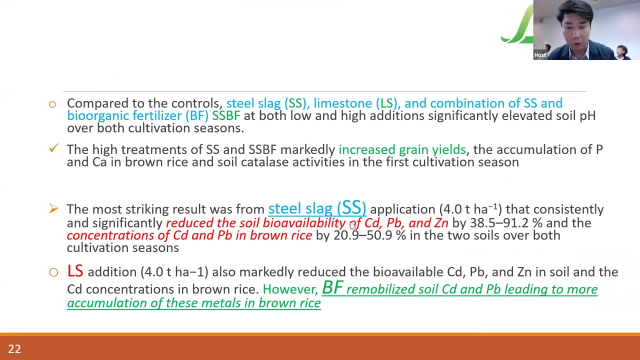 steel slab. they can actually do a very good job. it can reduce the soil bioavailability. because- still slats- most people would think that, oh, they're just a byproduct from a stainless steel, just like stone. okay, we never think that it could do a good job. they could reduce the soil availability- okay, not just for. 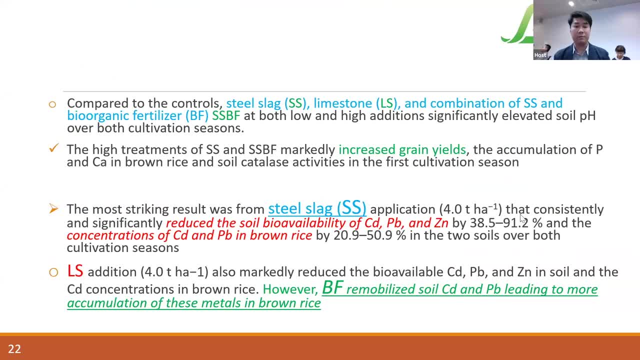 cadmium, but also for other kind up to 90 percent, and not just availability, being reduced in the soil. at the same time, the rice accumulation, okay, also drop for the limestone. i think, uh, undoubtedly could be very nice, because it could affect the ph as well as reduce the bioavailable. 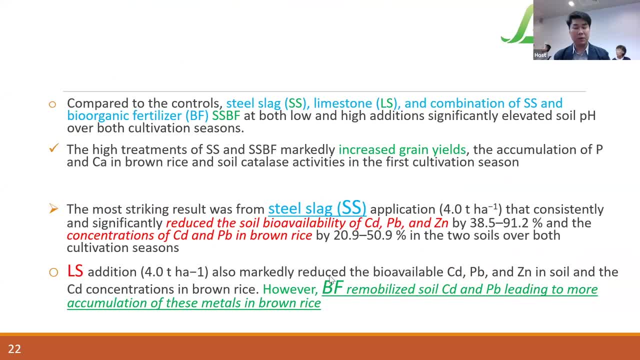 metal in the soil. but what we are somehow being alerted is the bio organic fertilizer. that's most of the pharma we use and we found that. we found that the fertilizer will remobilize. that means it will activate, okay, even further, mobilize- a metal in the soil. 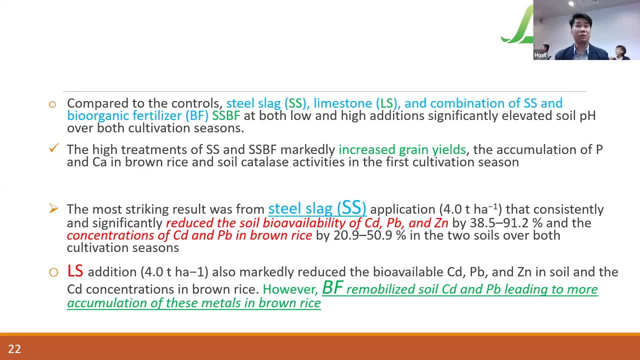 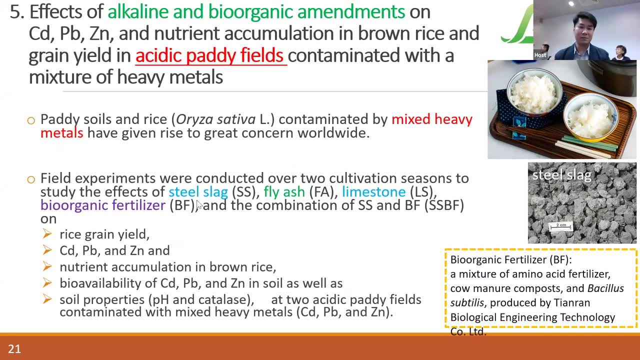 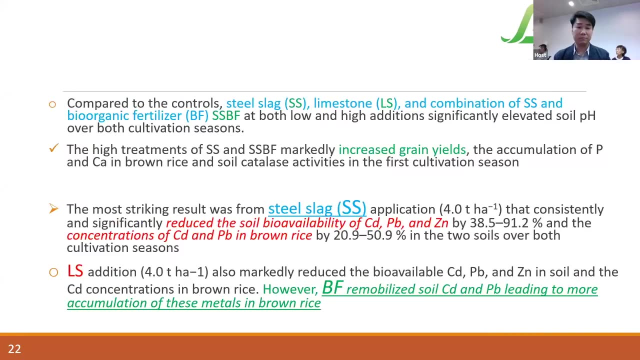 that's is actually an alarming problem for the farmer and of course, we suggest them stop, you want, using this kind of fertilizer because they think it would be good, but rather this case: some rub, some ash- okay, or even some industrial byproduct actually doing a very nice job here. 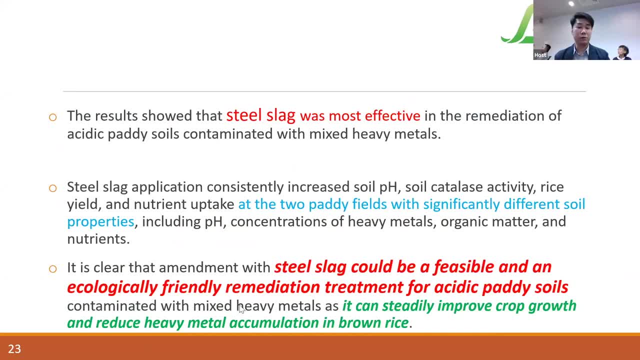 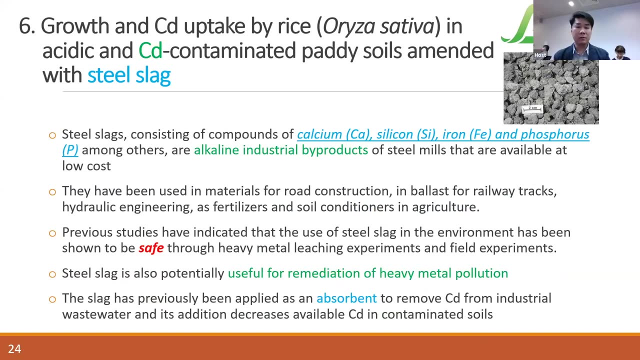 And then this still slap could be a feasible- and also a good friend- remediation treatment for the acidic soil, because it can also control the pH as well and also improve the crop growth as well. And then we try to have a detailed investigation with just the steel slag okay, which is a 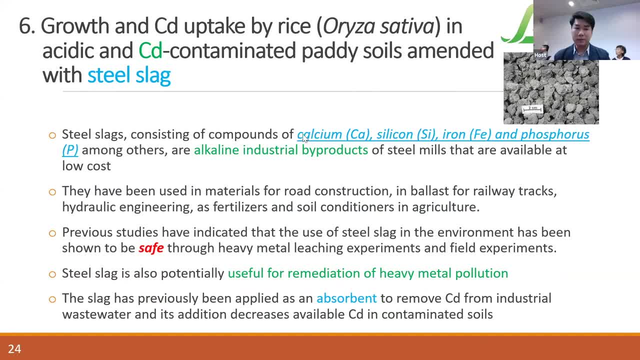 byproduct from the stainless steel factory And we found that the steel slag actually contain calcium, silicon, iron and also phosphorus. That means they are not rubbish. They are not some byproducts. actually, it could be a safe okay or amendment okay. 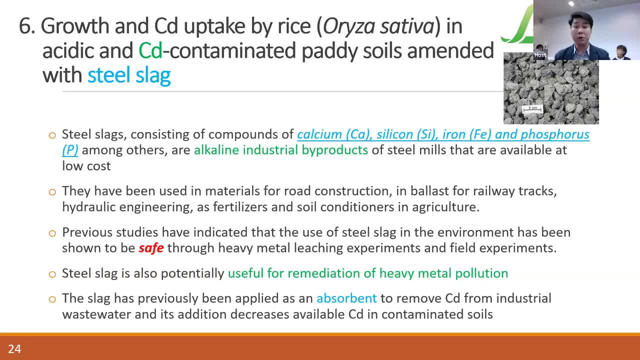 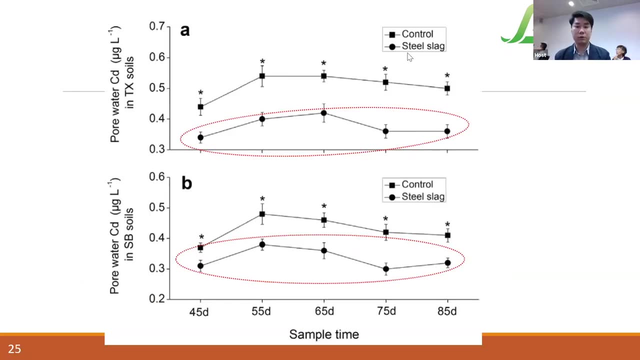 for farmer that's to grow their rice on the contaminated soil. It could be. It could be useful for remediation as well as the agriculture as well. So they could be a solvent. we call it a kind of biosolvents And what we found is: you can see, we try to locate different mine sites on the upper. 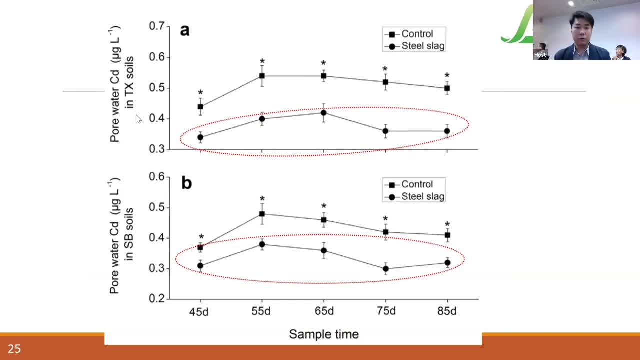 part and also lower part, And what we found is the poor water cadmium. this is available cadmium concentration in two mine in the two mine sites above, significantly lower okay than the control. So that's mean this steel slag did a very good job in stop the mobilization of the. 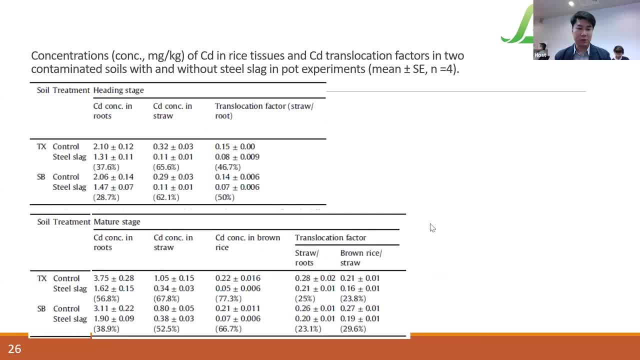 cadmium in the water, And, of course, we're not just talking about the concentration in the water. what we concern is the food that we eat. okay, it's a cadmium concentration. okay, after we add the steel slag in both sites, the concentration dropped significantly. okay, up to 72%, and which? 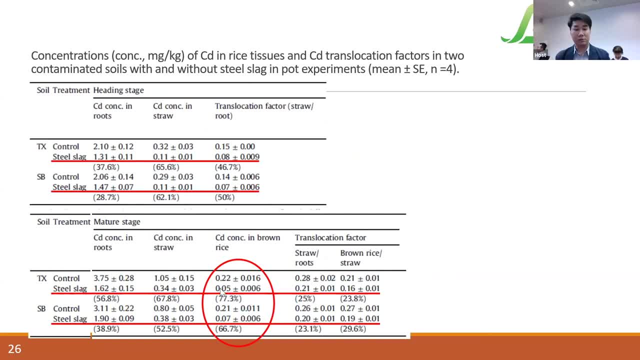 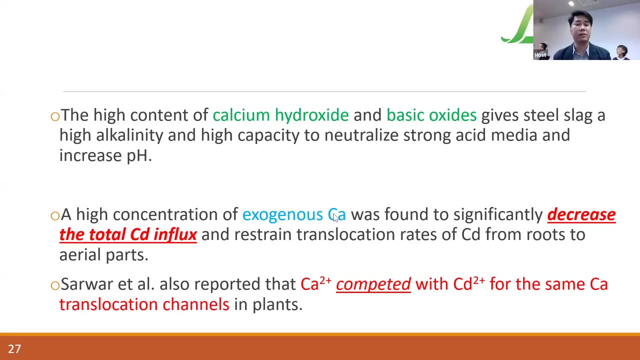 is also safe. okay, now becomes safe. Okay, just 0.0% Okay, Which is actually actually very nice as a safe food, okay for that district, So that we try to find. oh, as I mentioned, it contains very high concentrates of calcium. 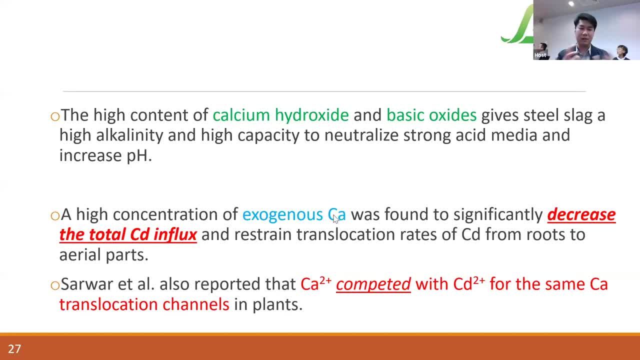 Okay, And if you know that calcium is somehow pretty similar to cadmium, okay, the size, the properties. So that's I always say that cadmium and also calcium, somehow they compete themselves. that's being uptake Okay. 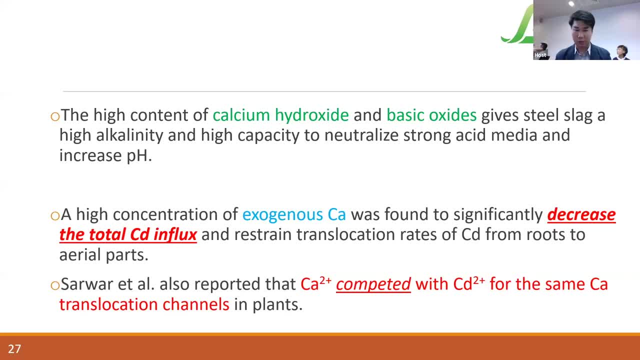 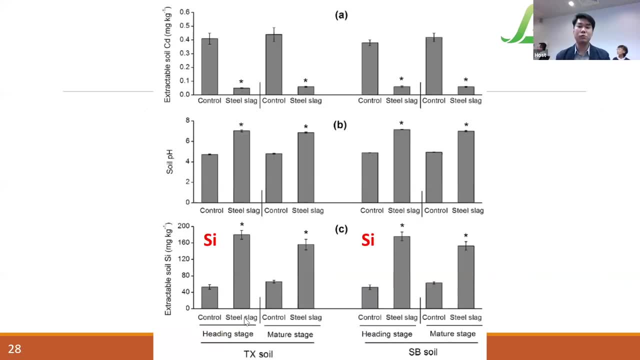 So that the calcium will decrease the total cadmium influx okay in the root to be uptake by the root. At the same time we also found that steel slag also contain very high concentrates of silicon, okay, which is a kind of rare earth material, and the silicon will somehow also 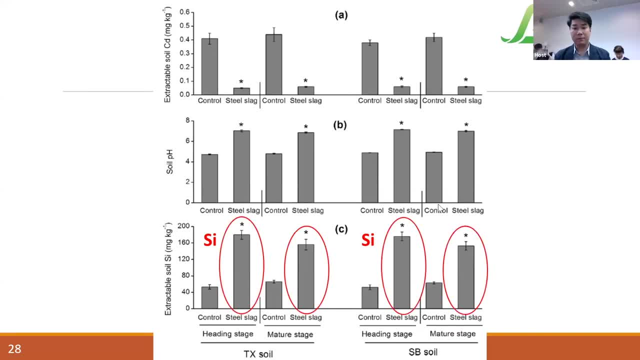 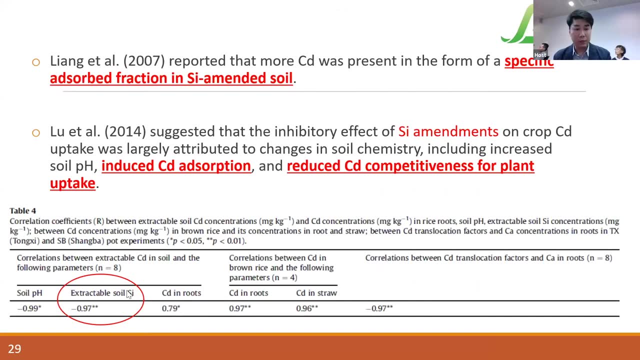 do good as well. okay, So that we also find a very nice negative correlation with the extractable soil, silicon as well as the concentration. So that with these two properties, with the calcium and also with the silicon, that will also support the steel slag to be a very nice absorbent. you know, amendment to be applied. 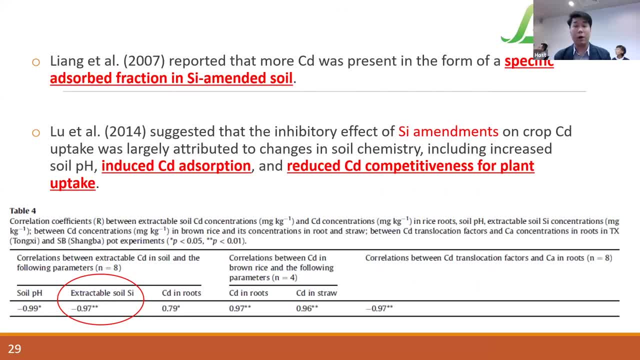 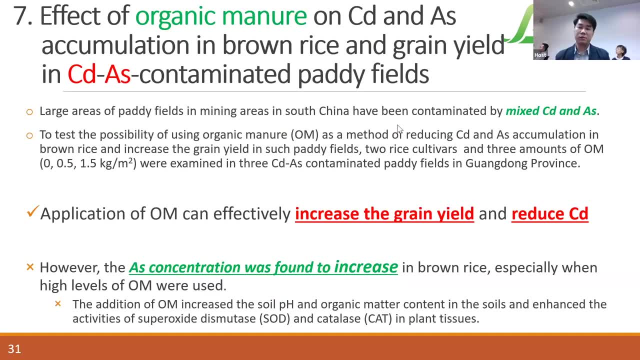 and to be adopted by the farmer in this kind of pollution for rice growth. Okay, So, as I mentioned, in authentic condition we try to see not just the chemical but also the chemical. Okay, Okay, Okay, Okay Okay. 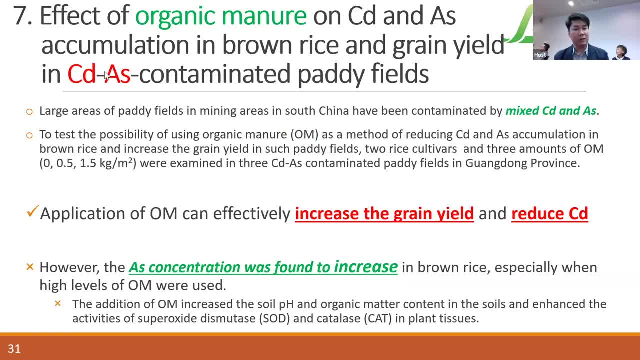 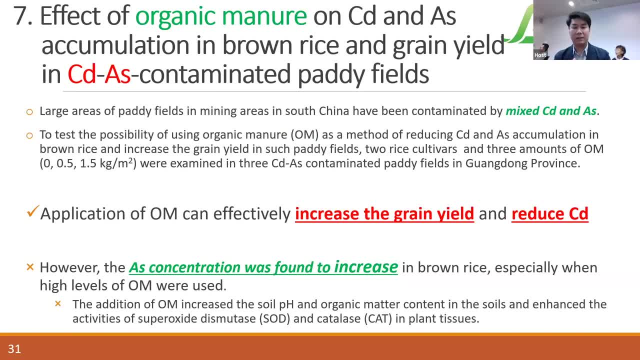 so on and so forth. So we try to see and we luckily identify a site with these two kinds of pollutants and we also try to use a common practice which is applying organic manure. Okay, are in this kind of contaminated site with the plant, with the rice plants cultivation? 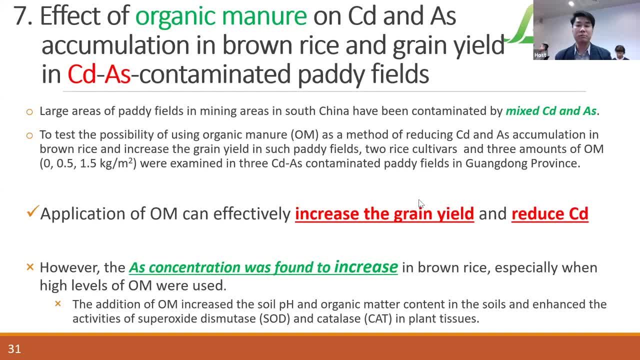 right with this organic manure. of course the grain yield increase okay. at the same time it can reduce the cadmium. but unfortunately we found that we cannot get one stone for two birds because at the same time the arsenic concentration was found to increase. this is also automatic patient. 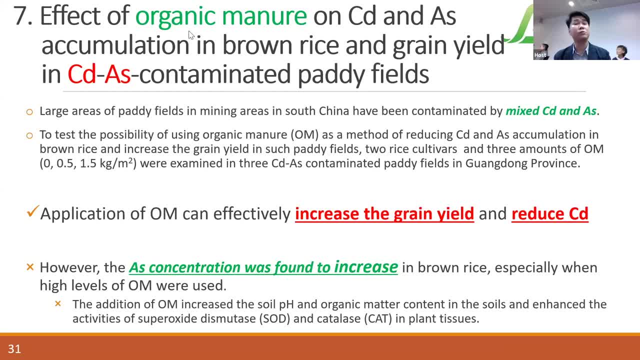 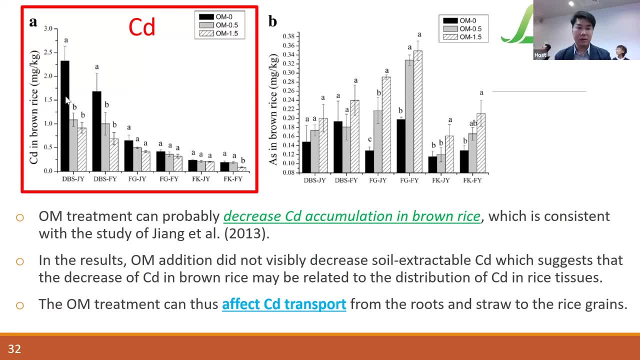 and also, we are sorry to the farmer, we cannot solve the problem by just using organic manure alone. so you can see for the cadmium concentration, cadmium cases, okay, when we apply the organic matter. so black bar, which is, uh, the control. once we add the organic matter you can see which is. 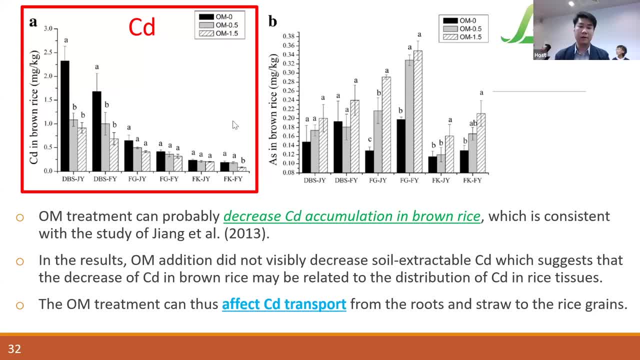 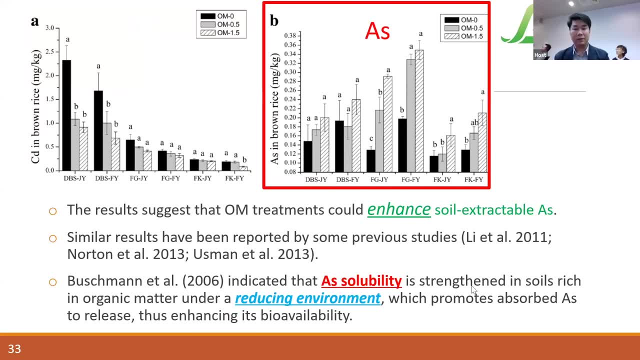 significant drops of cadmium concentration, the rise okay. but for the arsenic, okay, the condition is opposite. once we add the organic matter, the concentration of arsenic rise is significantly increased. and maybe you know when we grow the rice, the condition basically, which is a flooding reducing condition and under this condition, maybe the organic manure somehow. 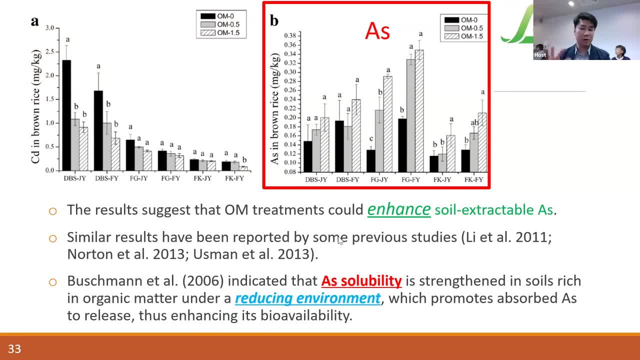 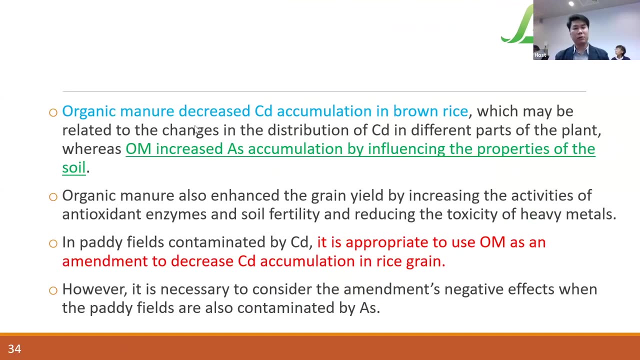 will activate, activate the bacteria and somehow eventually induce the arsenic solubility. the cadmium is opposite. okay, because the reaction is totally opposite, reverse, so that in this case we will say that okay, if we use organic manure, somehow they could do good for cadmium accumulation, but they're not doing. 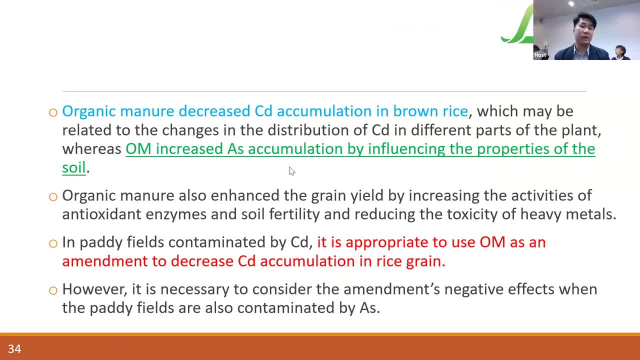 very well for the acid accumulation. that means we can- at least can- let the farmer know if your soil is just cadmium contaminated or some a positive iron contaminated. well, you can use organic matter, you can. you can use organic manure, but if you found your, your soil is polluted by arsenic. 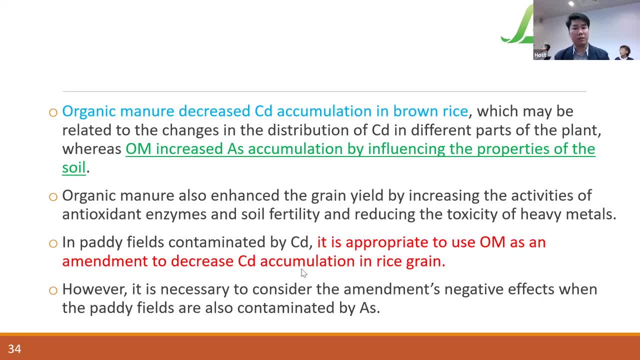 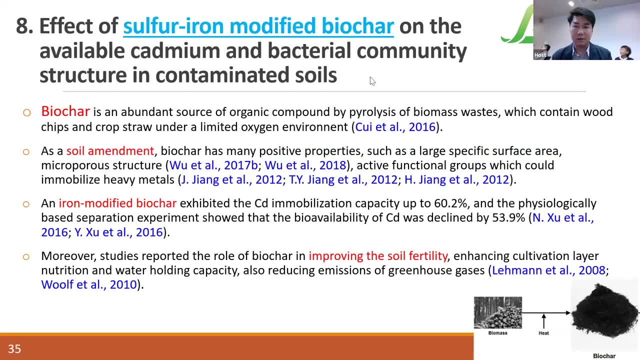 okay, or mercury so and so forth, then you should not use organic material, otherwise you will even obtain okay. so that in this case, uh, it seems organic matter, i mean organic manure, seems not doing very well in this case. and we try in the past few years, we try another technologies which 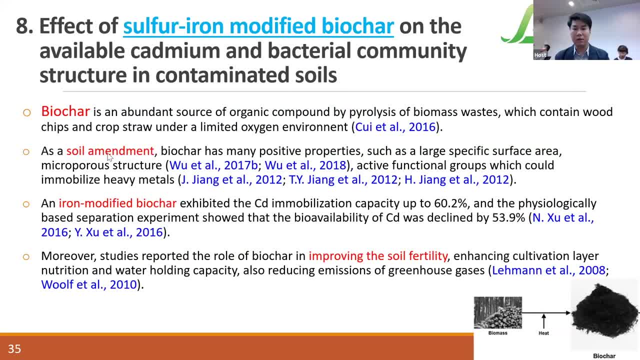 is a bio chart i think all you should know about. just is very popular in the past few years and, of course, this kind of bio chart, in this case, in this research, we're not just using a typical one. we try to amend with, uh, sulfur, okay, and also with the iron. 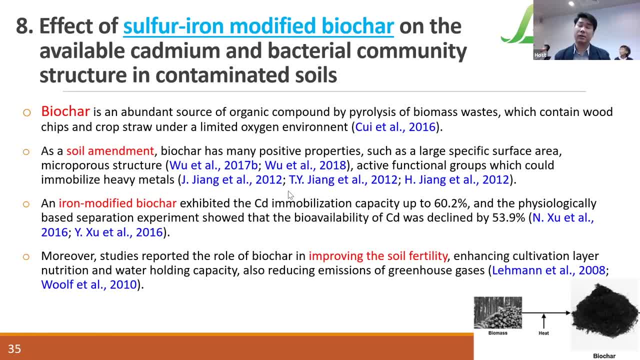 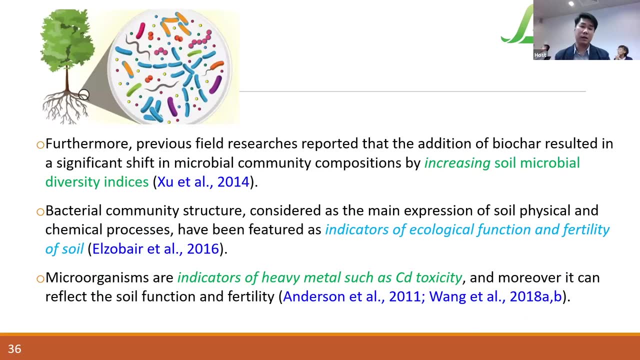 because the bio charge, i think you should know, which contains very high concentration, is carbon okay, or yield seeds and so forth. it could also do good to the soil fertility as well as for the microbial growth, because we found that the microbial growth or microbial index, somehow, is a 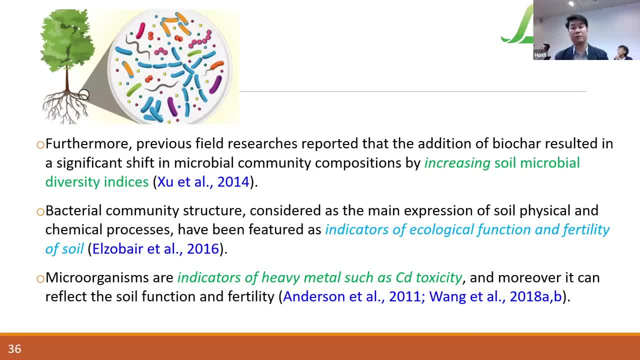 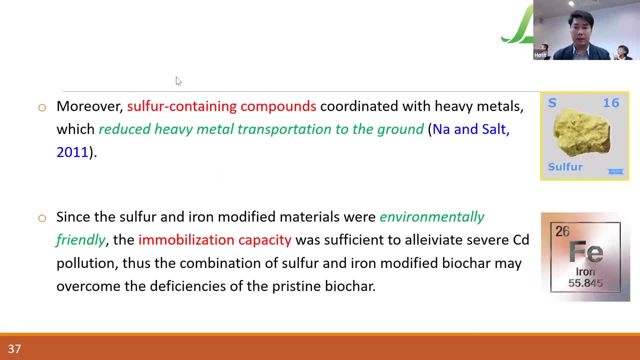 indirect indicator for the soil health or even for the plant health, so that at this time we also consider the soil microbial diversity index in this part- and for the sulfur and iron- i think this is a very well-known okay material that's to reduce the medical transport or medical 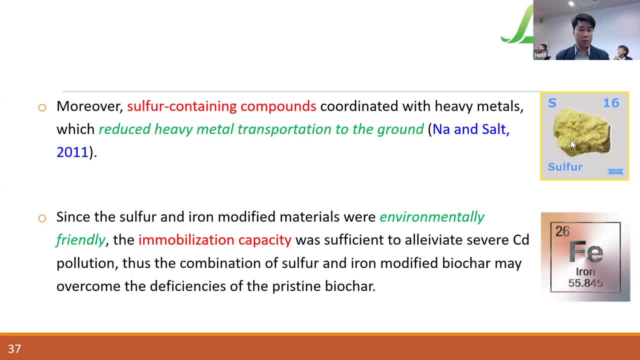 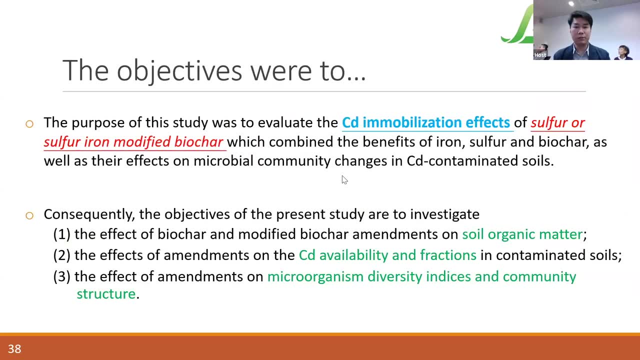 availability in the soil. but that's why we try to incorporate this two kind of mineral with the bio chart production. so the objective is to uh, to investigate. if there's two friends, okay, the sulfur and also- i modify biochar, do good on the chemium immobilization as well as on the microbial community. 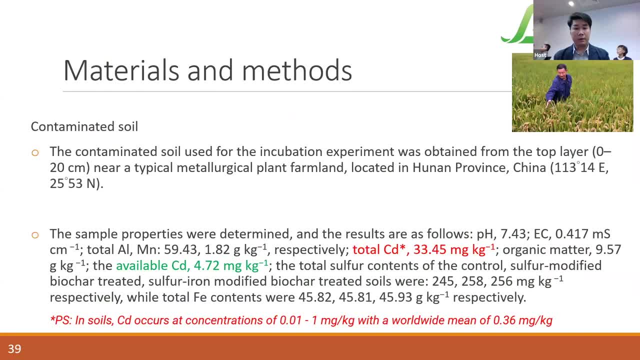 uh, cadmium availability, so and so forth, and we found one site in hunan province, in hunan province. so let's see the normal range of cadmium. okay, which is rather low. okay, 0.01 to 1 ppm. okay, the world means is around 0.36. so if the soil contains around one or a little bit above this is muted. 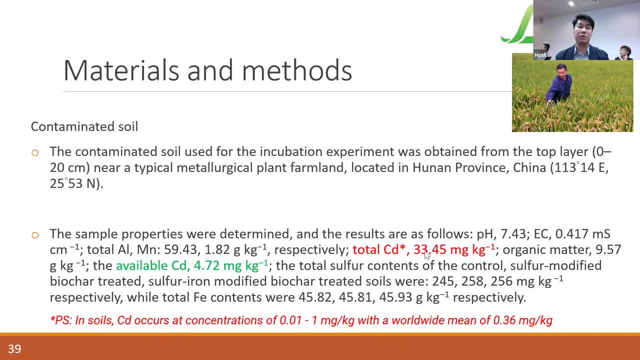 and now we found this site is 33 ppm. this is excellent, extremely high the total and for the availability. it's talking about 4.7- 4.7. so i would say this is a highly polluted site with cadmium and this is our target and we can also use this site to test. 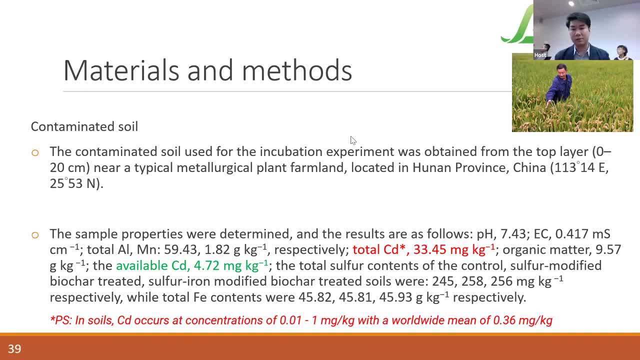 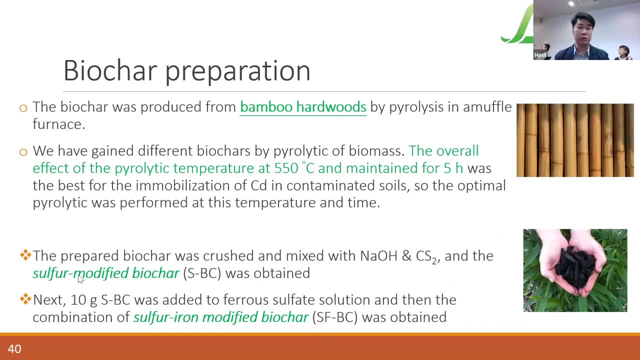 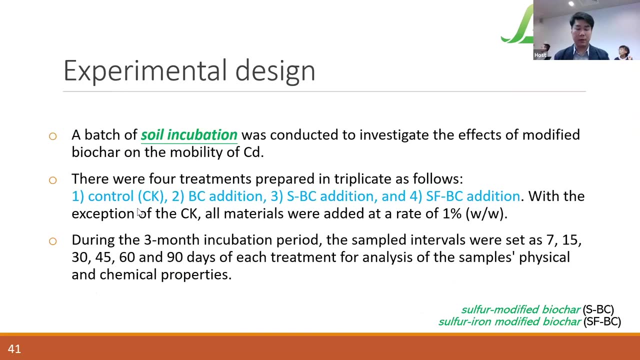 whether our biochar is doing, doing good and in the site and the source of the biochar. we're using some bamboo hardwoods- okay, and of course we add the sulfur and also iron again during the production. okay, we have different uh uh trimming to control the biochar alone and also sulfur with the biochar and also sulfur. 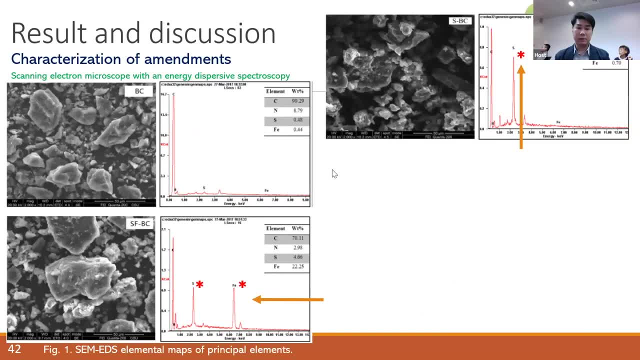 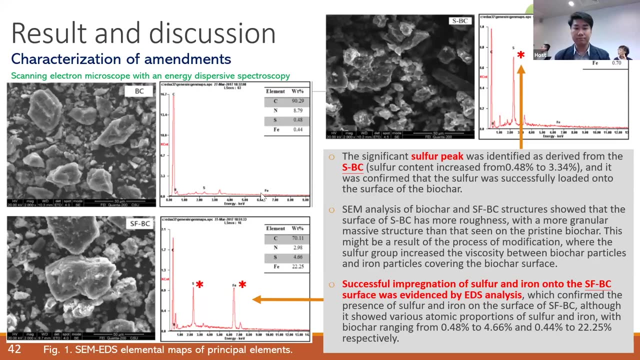 plus the iron with the biochar. so let's see, uh, with the scm, we- at least we- can find that, uh, it contains a very sharp peak for the sulfur and also for the iron is actually proof that this is a successful implementation. okay, and about itself? and then we found that 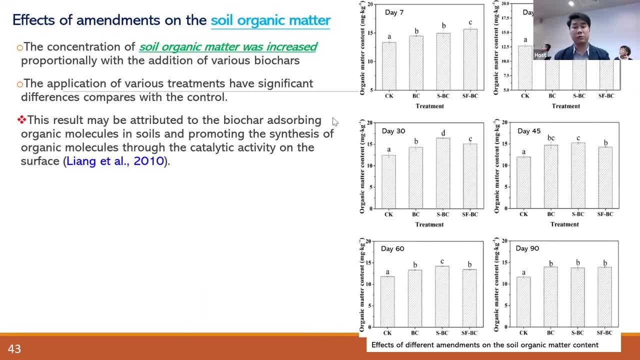 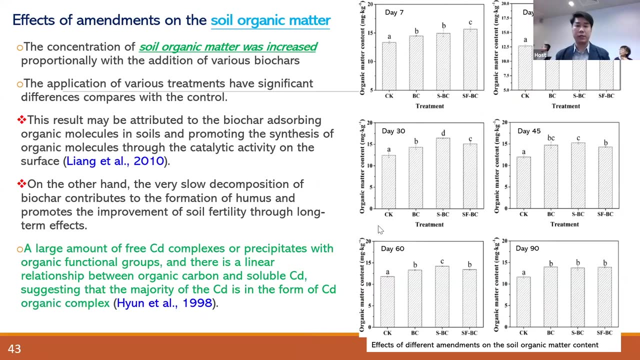 right, the soil organic matter: okay. after a several incubation period, we found this organic matter was increased successfully with the biochart addition. okay, and of course, this biochart, as i mentioned, which is rich in carbon salts, so that it can provide a very good duty. okay, and this duty, of course. 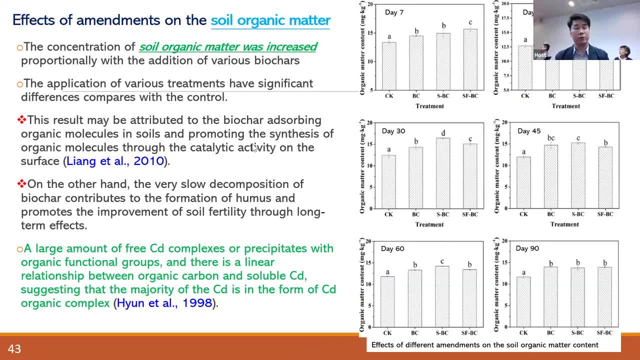 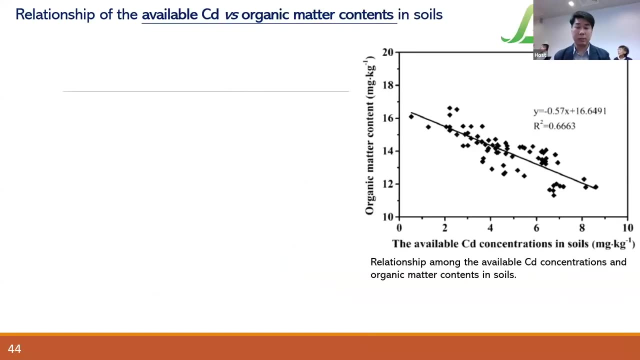 they could somehow immobilize the cadmium, so it's reduced the rise of plate. but as it's carbon, it's not just provide a good source to improve the soil fertility but also control the cadmium availability as well. And here shows the relationships with the DOC, as well as the 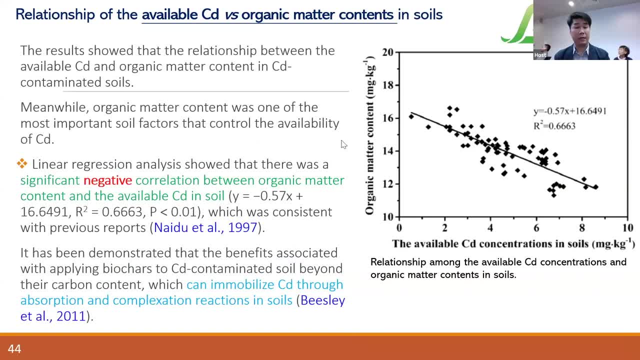 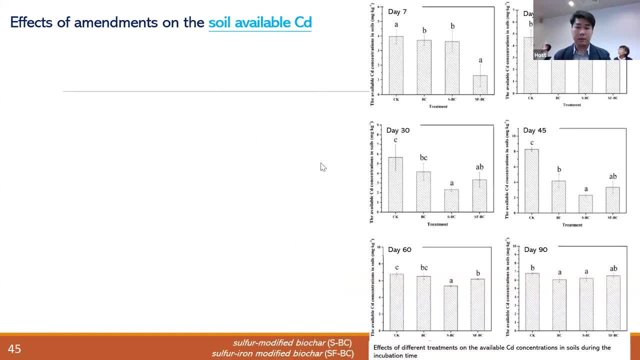 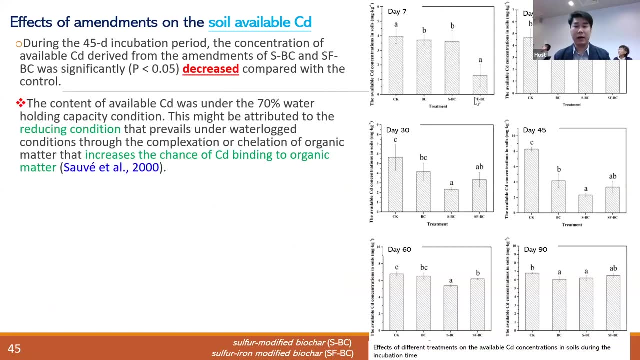 available cadmium concentration in the soil. This is a negative correlation and they can of course immobilize the cadmium. And here shows the soil available cadmium. and what you found is with the sulfur iron addition it can actually significantly decrease the soil available cadmium very. 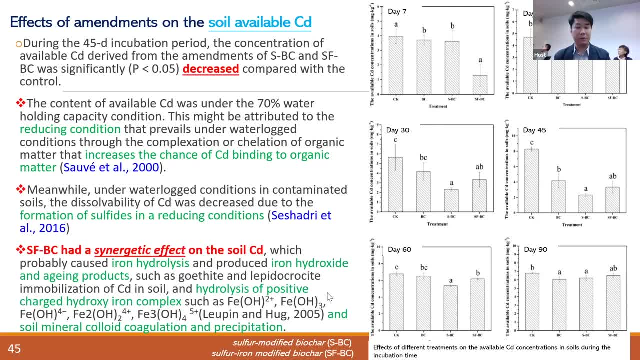 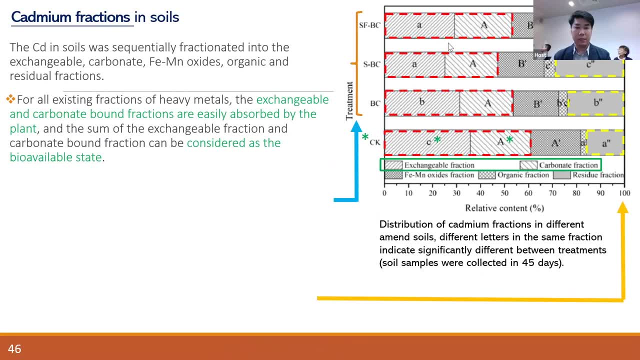 sharp and they also have some synaptic effects on the soil- cadmium as well. Last but not the least, we also found that the residual fraction that's for the biochart treatment- the sulfur at the biochart and sulfur iron at the biochart- 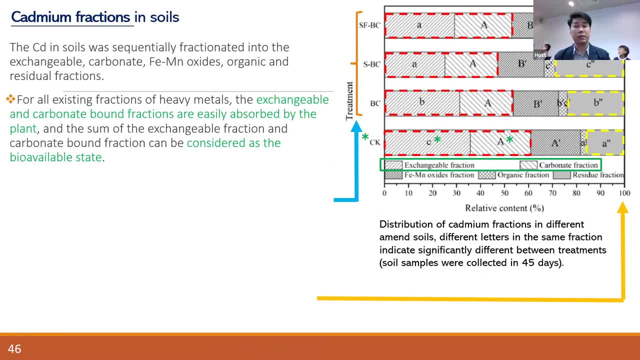 what you found is the residual fraction is increased, while the mobile fraction, exchangeable fraction, carbonate fraction actually decrease significantly, So it's actually improved. the speed section of the heavy metal in different form, of the cadmium in different form, is also being reduced significantly, So that's the immobilization effect is very significant. 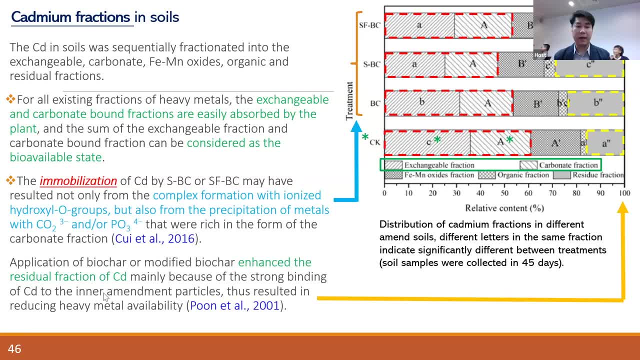 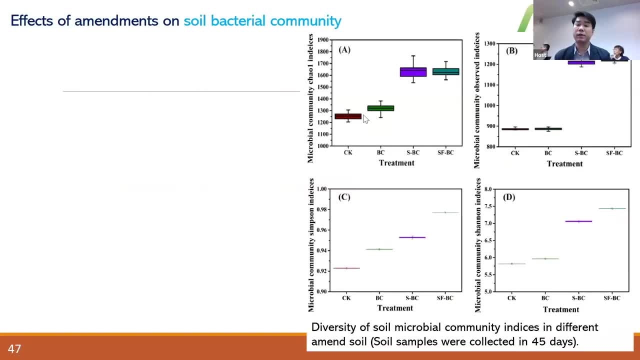 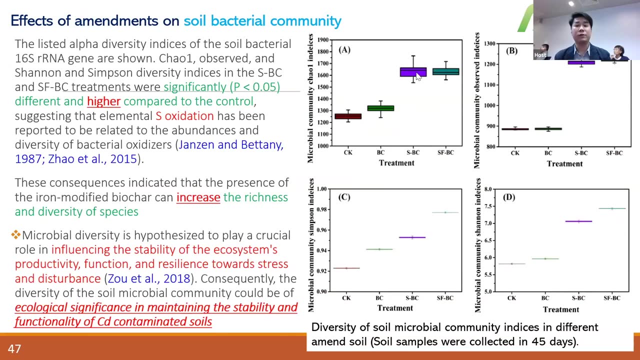 And of course, as I mentioned, enhance the residual fraction of the cadmium. And here shows the soil bacterial community. So on the right hand side you can find we try to use different index, the cow index, so on and so forth. And on the 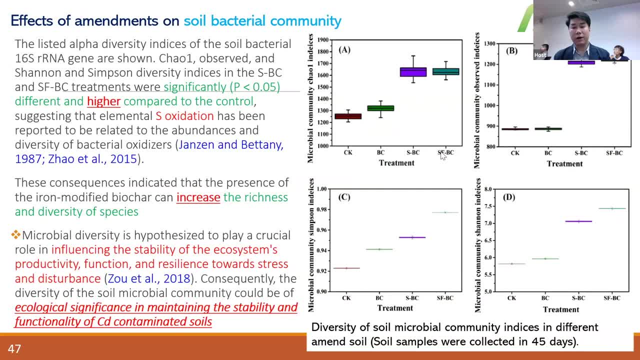 right hand side, the sulfur at the biochart and the sulfur iron at the biochart. they also significantly increased. Okay, so that's whatever the bio community, the abundance, richness, diversity, also improve this. So that's. these kinds of biocharts worked very well in the soil. the 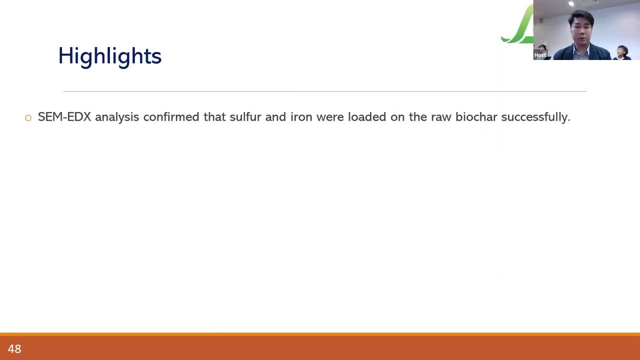 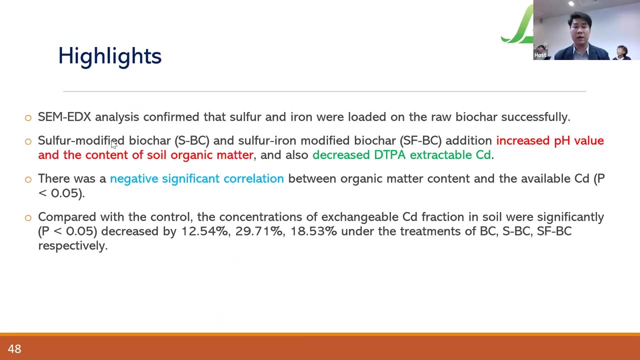 material as well. So this is a quick highlight. this kind of biochart- I mean not the traditional one, what I focus, which is a sulfur modified and also sulfur iron modified. they improve the pH, improve the soil organic matter, as well as decrease the BPA in front of the cadmium. 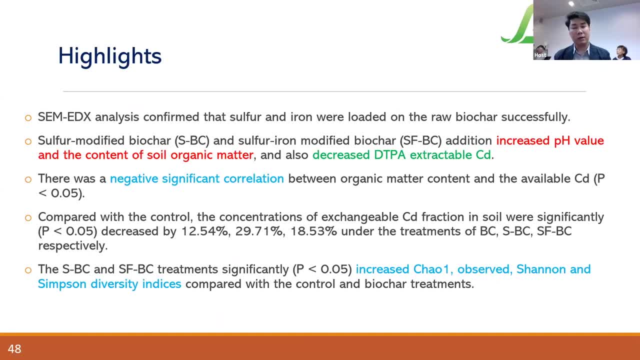 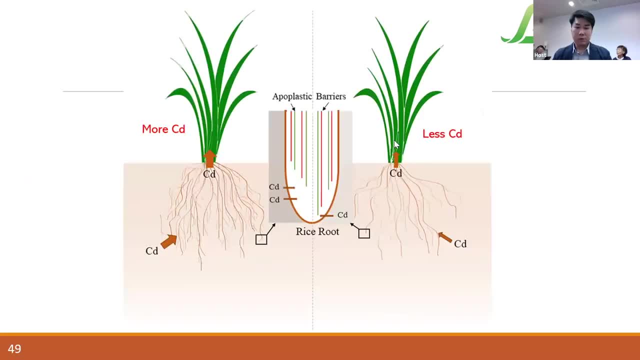 So that would be a very nice potential candidate to apply that okay with the farmer when they are doing the rice cultivation. So I'll try to stop a little bit here because that's a very quick recap. In the first phase we try to clean up the pollutants before we do the farming And in the second phase we try to 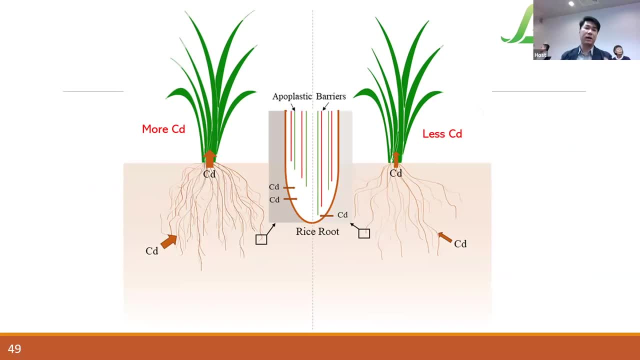 consider about: we try to grow the plant at the same time when we're doing some treatment by adding different types of fertilizers. And then the second phase we try to consider about: we try to grow the plant at the same time when we're doing some treatment by adding different types of fertilizers. 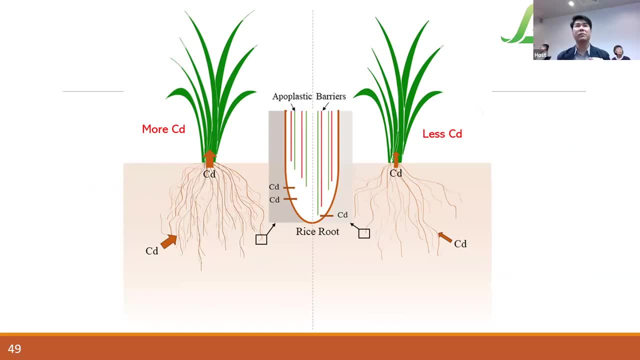 So first of all, we take the airfields, we use them and we start to Jord еen favorites, which we call it The. I mean we talk about Matt, but we have also discussed about- remember, we can't keep asked for your, so weml, they're all over the place. We talk about crops and we think that is something that, because all of a sudden we are at the same time in the country and we are sensations of that, we just don't get out in the field. 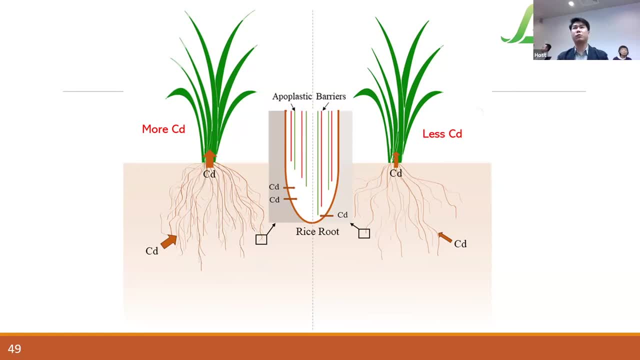 to ask them what people do. I don't, I don't know. it depends on what people do, but, frankly speaking, some farmers that very high, okay. so we think that if we keep using the amendment uh uh when they are doing the uh, 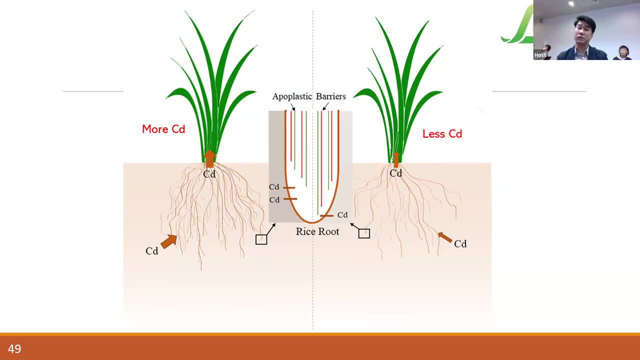 plants or rice cultivation. it seems this is not long lasting. every time they have to add, they have to renew biochar the amendment. so we are thinking: could we somehow not clean up the soil and also not add? amendment is possible and the farmer say, yes, if you can do it, okay, we love to try, we would. 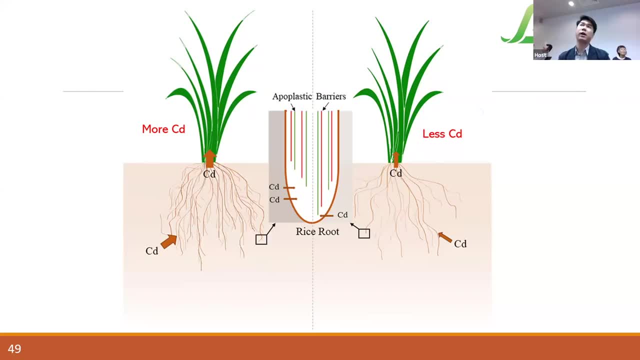 love to try. so, with this concept bearing mind, we try not to touch on the soil. which try not to touch on the soil, or touch on the heavy metal, just leave it. whatever the available form, total form, whatever, we try to focus on the plant itself. okay, so here, as we know, the rice which is accumulating. 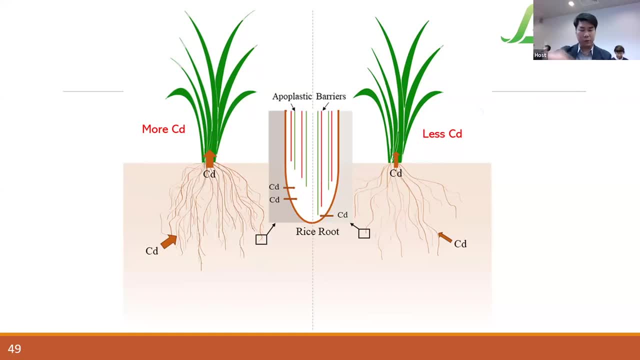 plants. they're not going to grow, they're not going to grow, they're not going to grow, they're not going to accumulate metal from the root to the shirt and also to the grain as soon as it's impossible to touch on the stem to the grain. so we work on the rice, we work on the rice root. so on this, 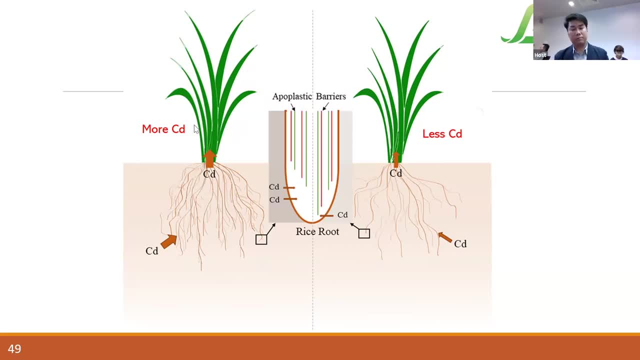 powerpoint. you can see, uh, we found that for some rice cultivar- okay, or some rice string, if they galactic more cap- because we found that the structure, the morphology of the root itself is significantly different. at least you can see the size, the root length, okay. uh, the network of the root itself is totally different for those rice. 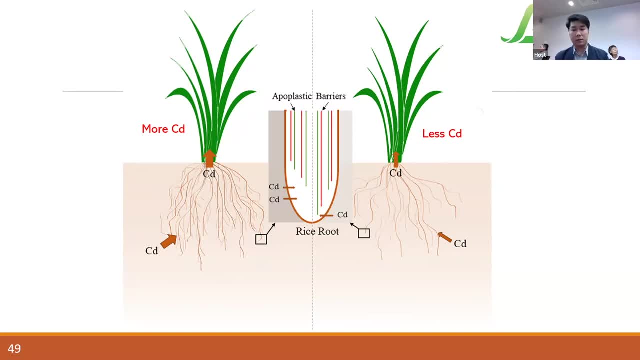 drain will uptake less heavy metal, which is easy, okay, but at the same time, besides um the morphology, okay, the number of number of uh root, i get the diameter. we're trying to take a look on some channel, okay, some channel, some uh uh apoplastic pathway, if a plastic pathway, which is the major. 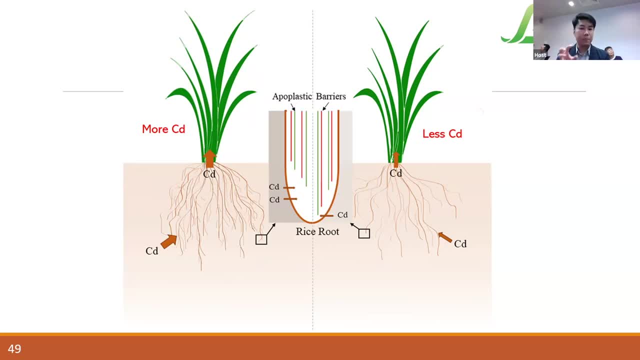 pathway, uh, the root itself uptake the iron, of course, including the heavy metal. so we try to take a deeper look, closer look, how root itself affecting the object, or heavy metal, if we, if we can somehow control or select, um, the rice root, that could somehow, ah okay, hinder the metal uptake from the wood itself. that would be perfect because 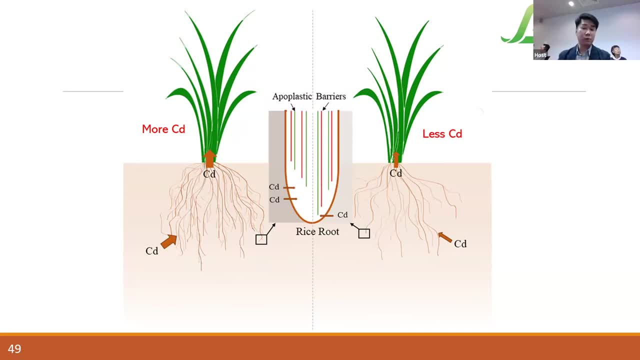 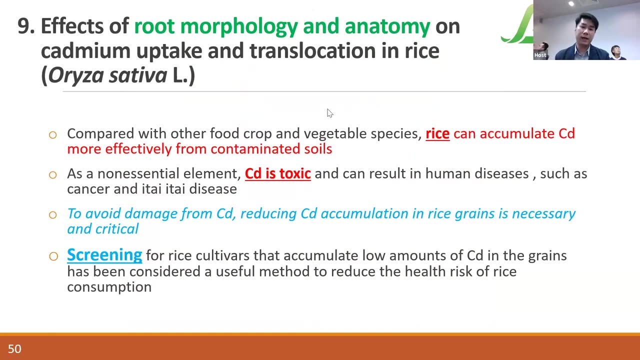 we do not need to, we do not need to do anything in the soil, so let's see, okay, if it's actually working. and again, we, we focus on the root morphology, we focus on the root anatomy, okay and uh, ultimately go, okay. ultimate dream is to screen, screen a nice, acceptable rice. 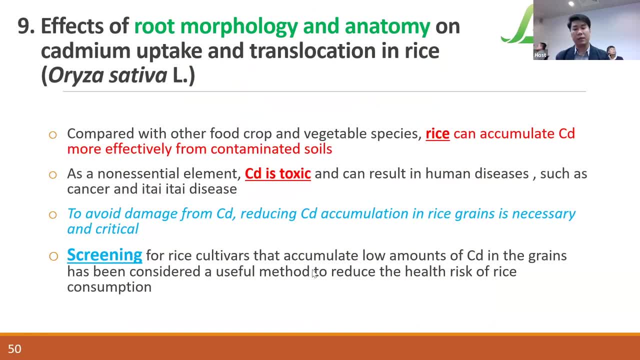 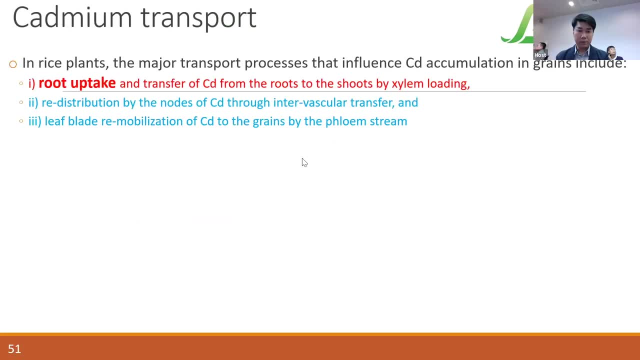 cultivar or rice stream, which could intrinsically accumulate low amounts of cadmium, bring itself okay. so, as i mentioned, the root uptake is the major. it's a key process and also it's the first part, that's a heavy metal interacting with the plant itself. 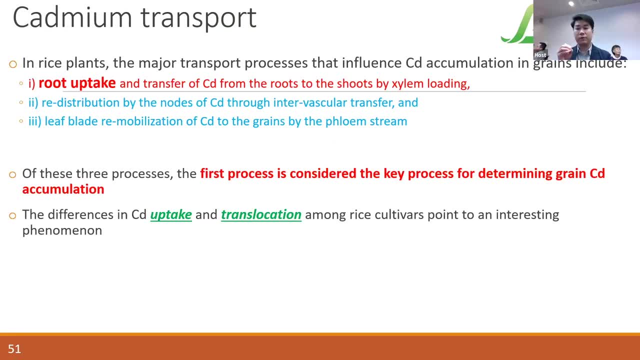 once it plants, what heavy material being updated by the roots? okay, the heavy metal will just transfer. okay, transport being within the whole plant. okay, so that once the heavy metal going inside the root, we can't control. what we can control is to ah, to bar the heavy metal being. 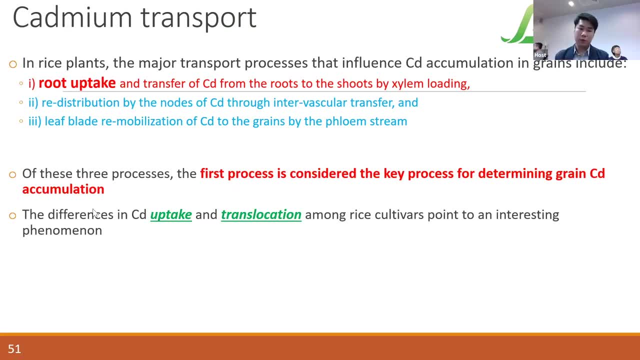 okay, that would be the only thing we could do. so we would like to see how cameo is being updated and what happens when it's not using the root. so we would like to see how cameo is being upgraded. we would like to see how cameo is being updated. 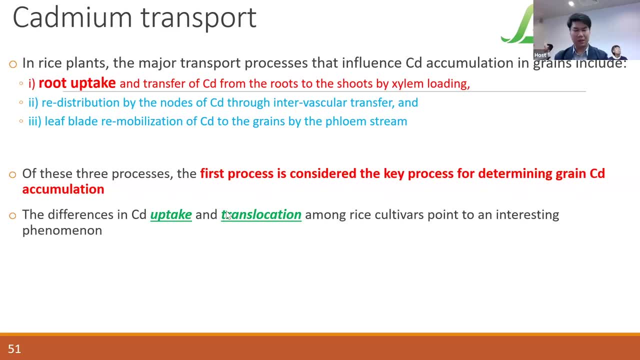 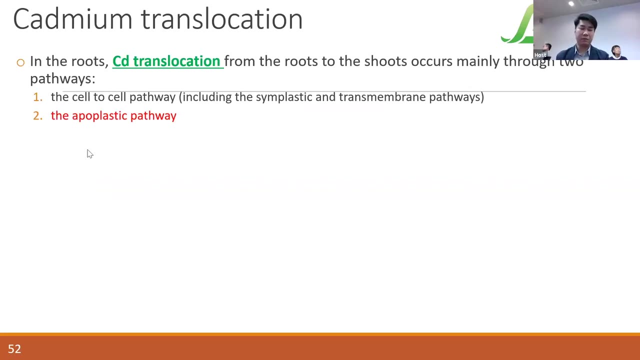 uptake or to compare whether uptake or translocation is more important to the accumulation itself. And for the TACMEM translocation, we found that there are several pathways- cell-to-cell pathway and also apoplastic pathway- And we found that this apoplastic pathway would be. 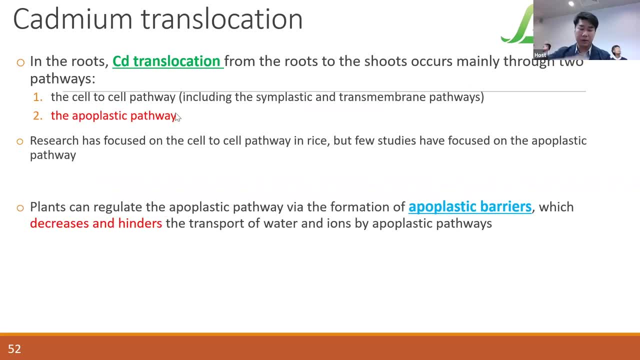 the major pathway, as I mentioned, that controls the ion uptake, ion transport, including heavy metal, And we do believe that there will form some of the plant, some of the cultivar. it will form apoplastic barrier, just like a goat keeper. It will hold the ball, it will. 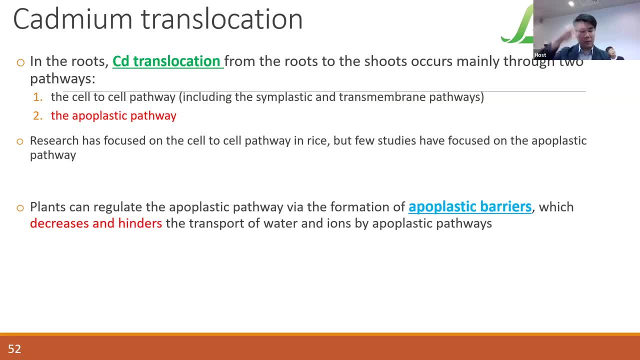 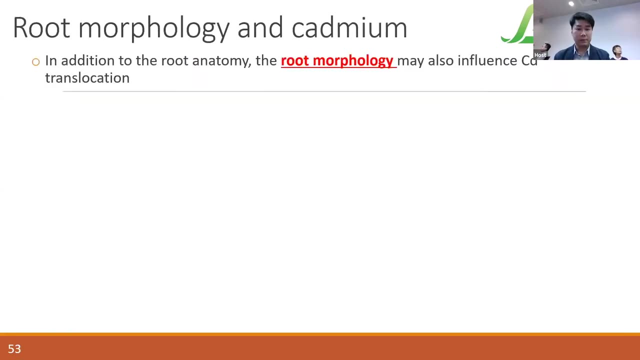 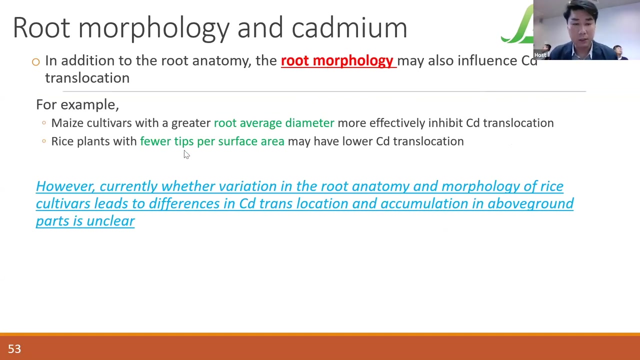 hold the heavy metal. it will trap the heavy metal that's being transported up or even translocated from the root to the shoot. We would love to find this barrier. what could be observed in the root? different rice cultivar, Let's see. okay, besides, we also investigated root morphology, just like the tips, okay. 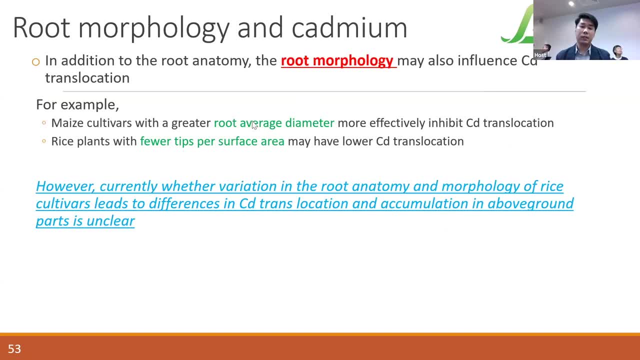 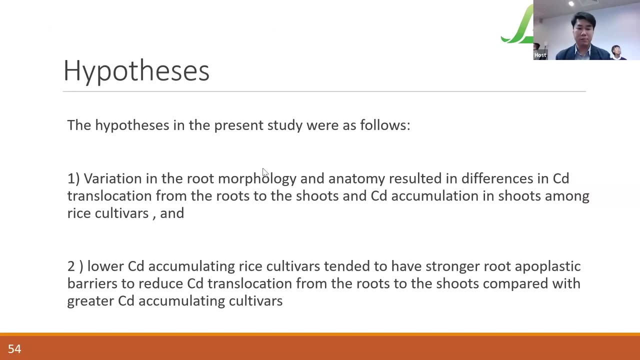 the hair roots. okay, the tips per surface area, the diameter of the roots, so on and so forth, and see whether they're also incorporated. okay, the process of the heavy metal accumulation. So hypothesis, of course we assume that the low accumulating rice cultivar they should. 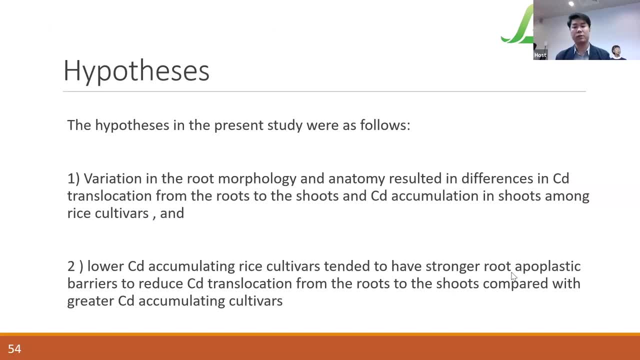 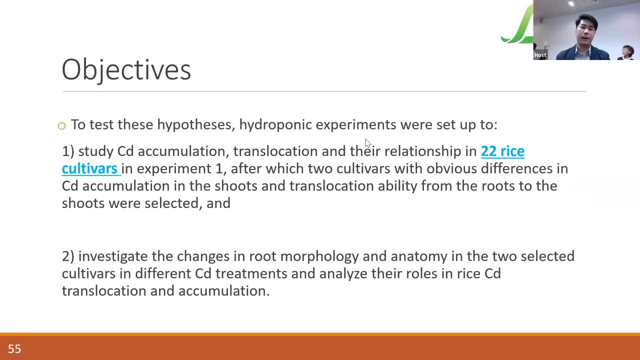 have a stronger- okay, powerful- root apoplastic barrier, Then they also possess different morphology, okay, and also anatomy towards the heavy metal uptake. okay, And we try to select 22 rice cultivars in Guangdong. They are very popular, okay, very. 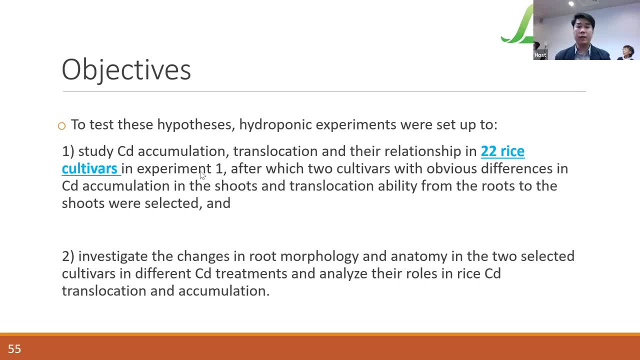 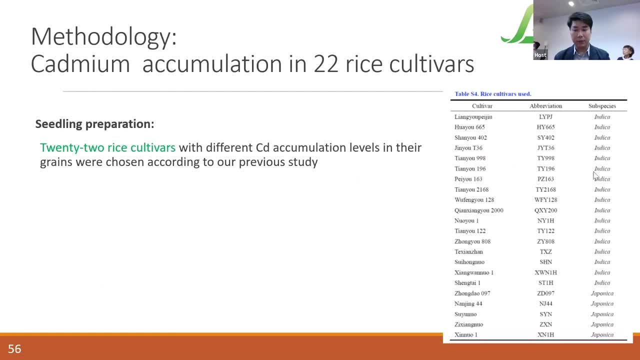 popular and they're also suitable for the weather in Guangdong, so that we use them, we select them And these are the rice cultivar name. okay, some of them are indica, some of them are japonica, and we grow them in the nutrient solution with the cadmium 0.1 ppm for a certain period. 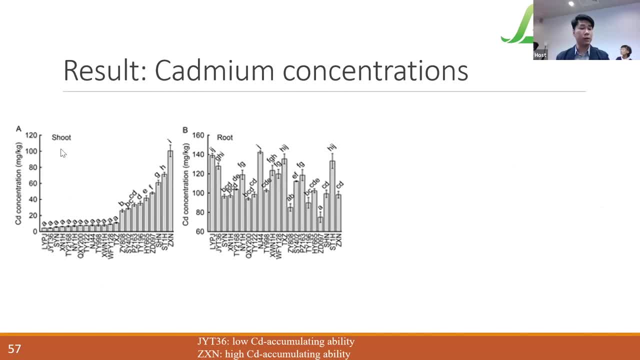 of time And here shows the cadmium concentration in the shoot. okay, and you can see there's a trend, okay, from the lower to the high concentration and the root as well. okay, it does mean different strain. they may have different ability in accumulating the cadmium. okay. 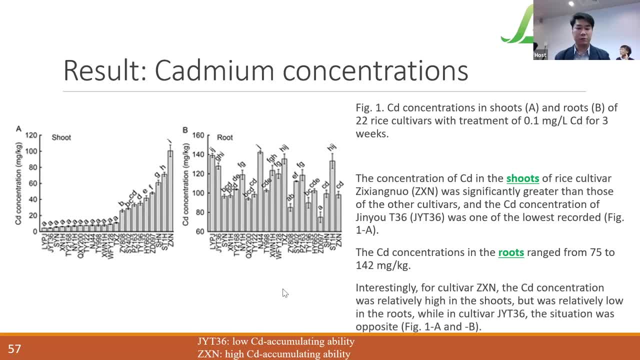 Everything is shoot and root, So we try to identify- okay, we try to identify- the ones with low cadmium accumulating ability and also one with high cadmium accumulating ability, so that this J-Y-T and that X-N is our target. 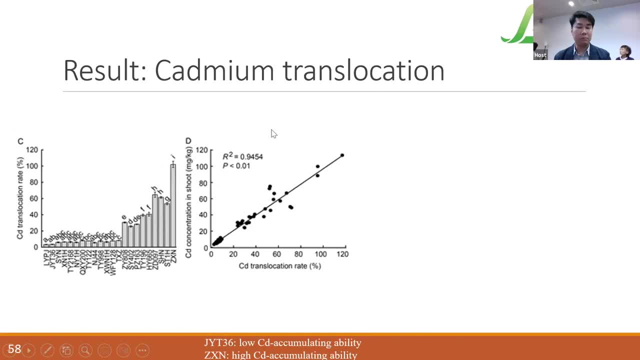 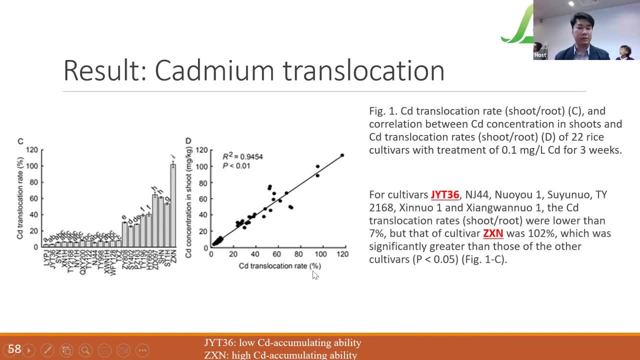 For the cadmium concentration. we also calculate the translocation, okay, and we also find that this J-Y-T and that X-N On top of that. they are myself in here, so we can see the difference, okay. Okay. so if we look at the above here, we can see that they're not the same, They're aqui. 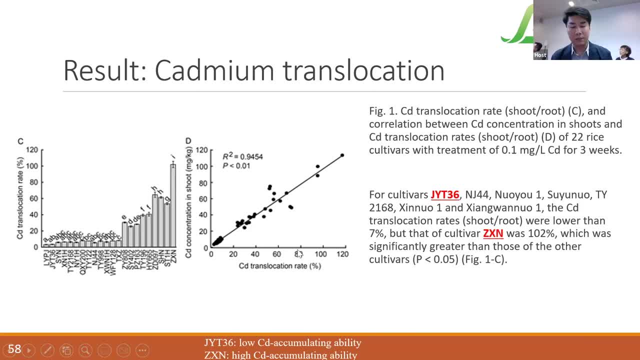 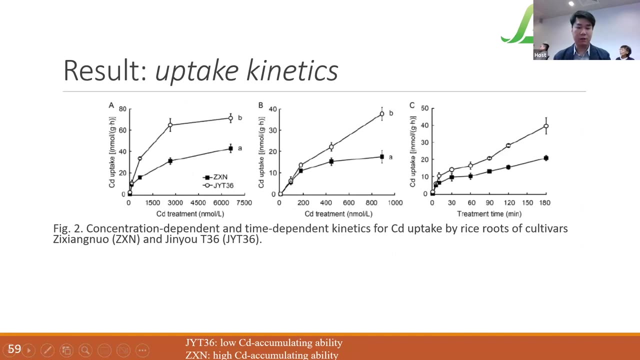 our good candidate to be test as a low accumulating string and also high accumulating string to see if they have any difference in uptake the pollutants, right, okay, so if you still remember, jyt is a low accumulating string, but in the uptake kinetics, uptake kinetics, this open circle, open circle- is jyt. okay, this also surprised us. this is a low. 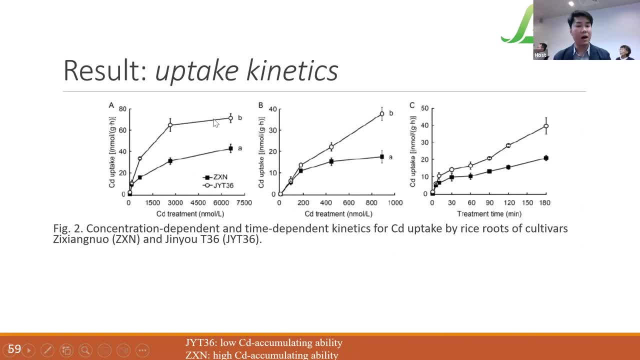 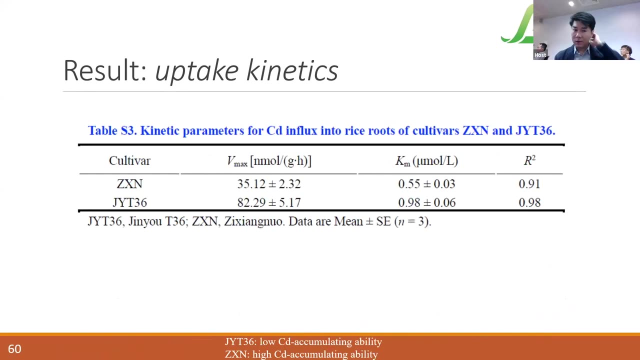 accumulating string, but the other kinetic is higher than the high accumulating strength. okay, suppose we think low accumulating ability should have low uptake kinetics. so in this case is somehow not following our plan. okay, and by different modeling we also found this low accumulator. they got a very high v max. okay, when compared to the high accumulating plants. 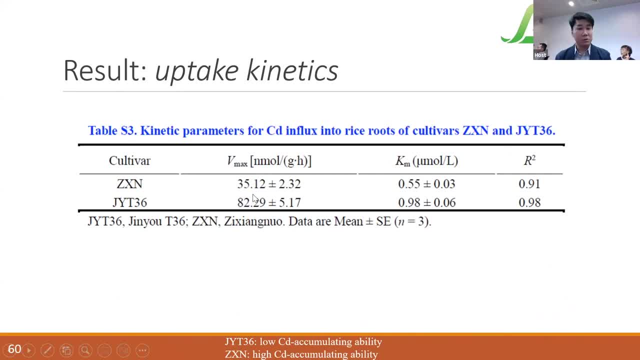 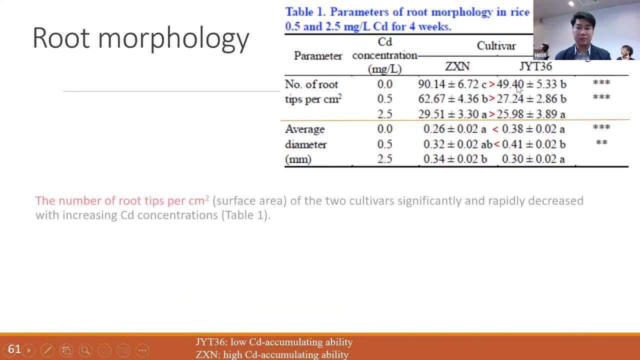 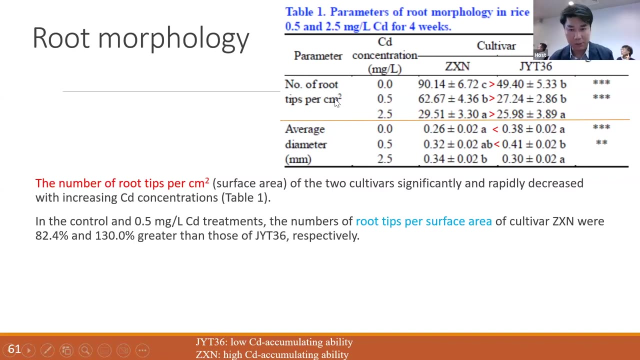 high accumulating strength. so this is very interesting. okay, besides, we also, uh, do some morphology analysis. okay, for the jyt low accumulator string, they should have a less okay number of roots- 10 percent quick, but with a larger average diameter. so it seems that somehow we cannot get a good conclusion. okay, we cannot. 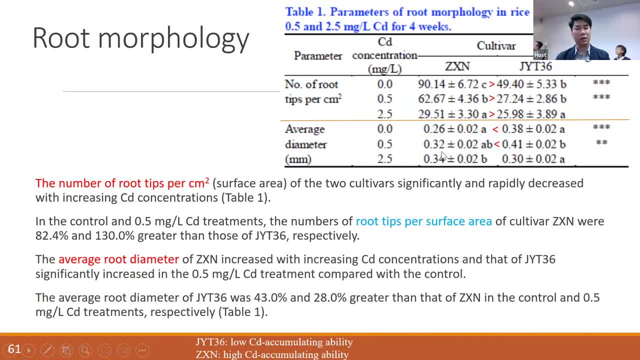 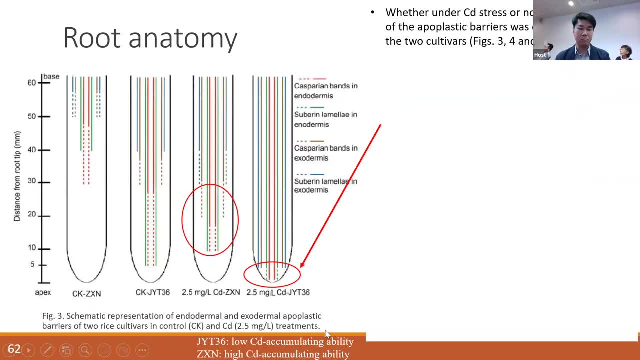 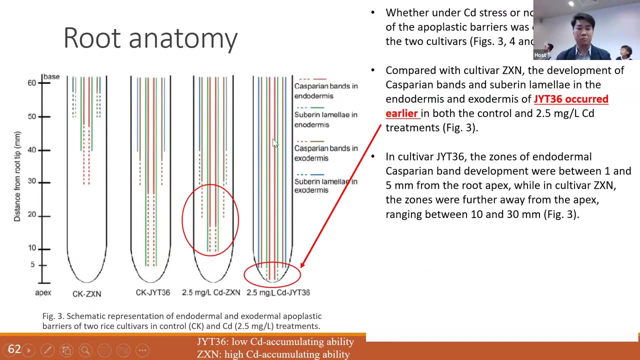 get a good conclusion. but okay, when we take a closer and deeper look, okay, two years ago we found that this jyt, okay, low accumulating string. oh, we found this some colorful line: the blue, the red, the green, the brown. these are the apoplastics barrier, apple plastic barrier. these are the gold. 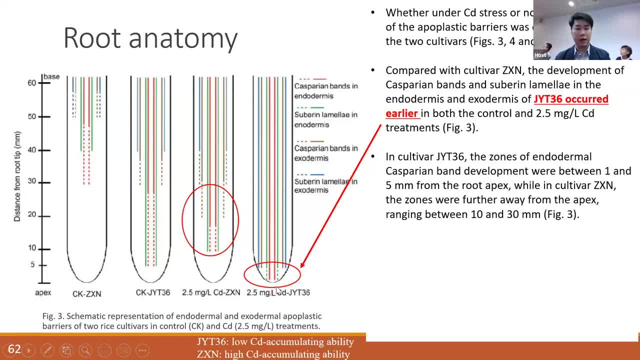 okay and in particular, when the low accumulating string okay under uh uh cad cadmium concentration condition. these barrier very, very early, especially around the apex. around the apex because during the apex, which is a very nice convection, a nice place for metal, for the water being uptake. 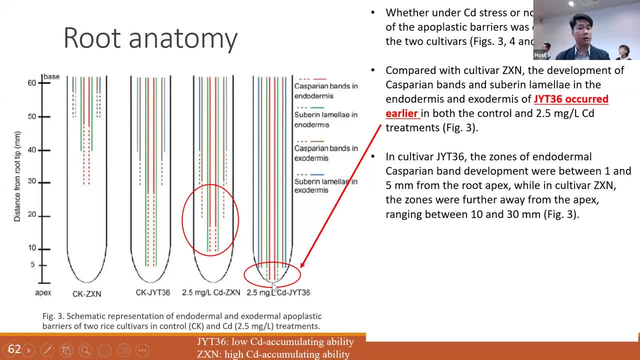 but these low accumulator, they start to develop this barrier. When compared to the high accumulator, this barrier actually somehow exceed. okay occurred in a later period, So we found this barrier actually working very well and also put a very significant role in bar. 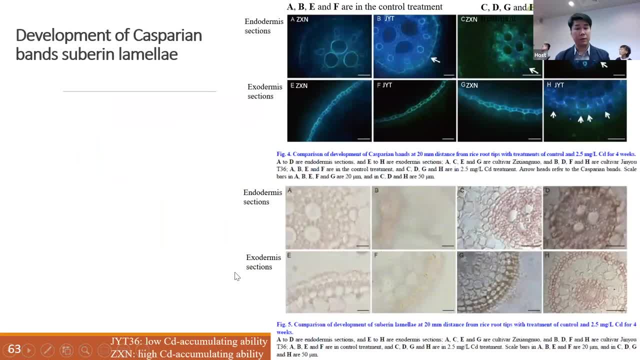 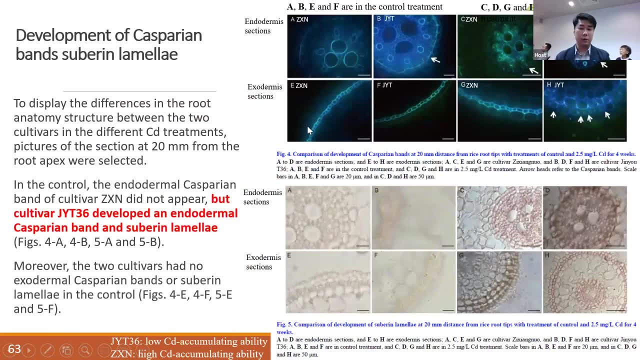 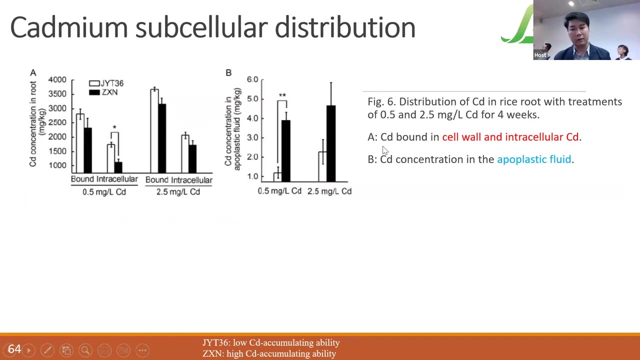 in hinder the metal uptake actually, or the translocation, And with different staining. okay, we also can found this apoplastic barrier is actually working here. Besides, we also tried to trace here: did those heavy metal go? Okay for the JYT, which is the white bar. 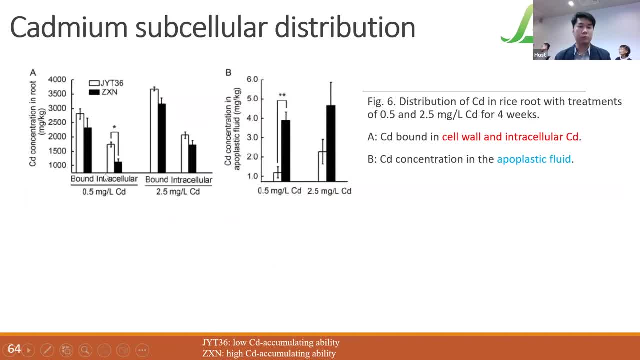 most of the cadmium actually are bound intracellularly. okay for the JYT, So we can find the lower accumulator strain. But for the high accumulator strain, which is, which are the black bar, which are in a apoplastic fluid? 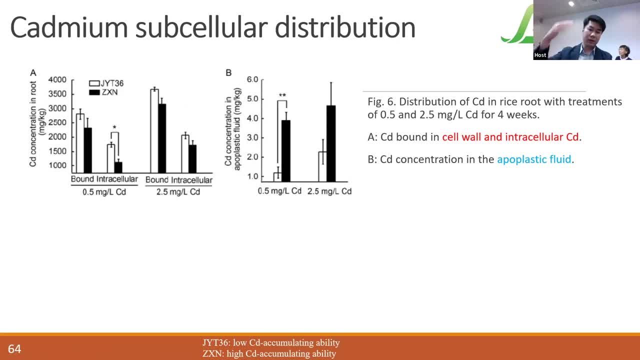 Apoplastic fluid, that's mean in available form- is being uptake- okay by the plant and eventually translocate and accumulate to the grain. So that's why translocation here is also a very important part. If we can bar the metal uptake by the apoplastic barrier. 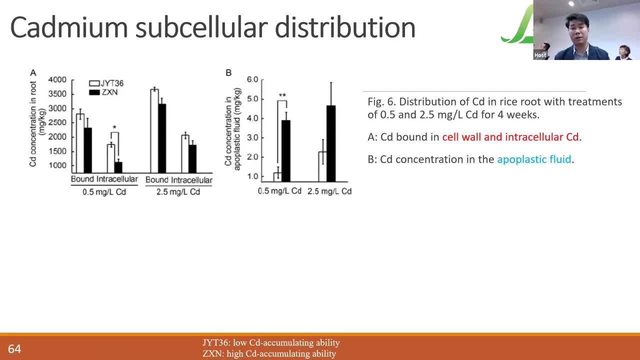 but if we cannot control okay to be uptake or to be bound by the agent, okay, so we can't control okay to be uptake or to be bound by the agent. If we can't control the intercellular component, that is useless. 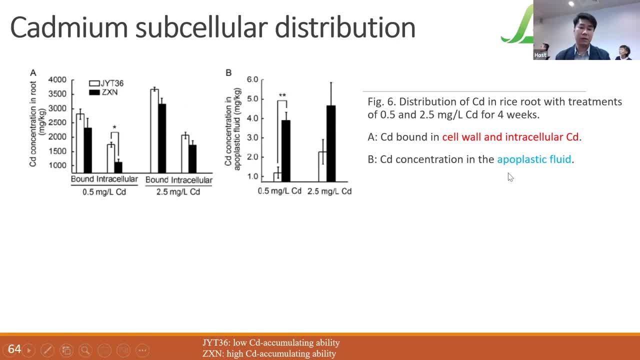 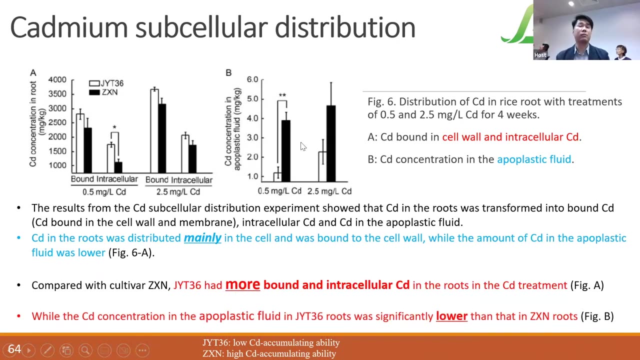 do that without the cadmium concentration actually in apoplastic barrier is much higher for the XN: high accumulating strain prediction. Okay, so that's this JYT. They had more bound and intracellular. That's why it would not translocate further. 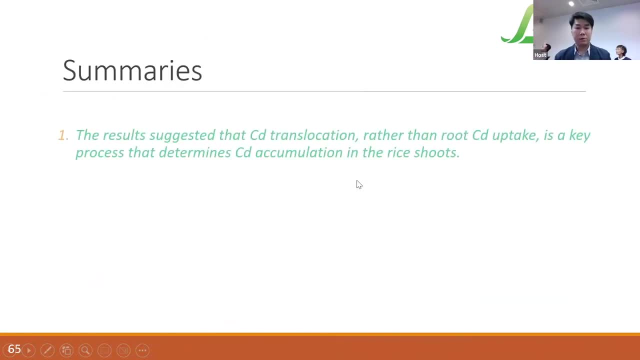 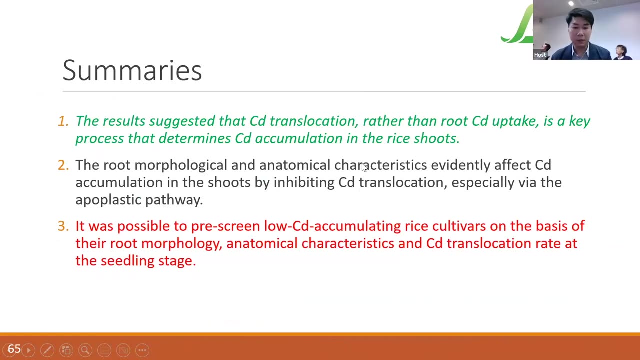 to the grain itself. Oops, the summary. we will say, okay, the Z-zone is at the bottom, that the cadmium, the root morphology and also anatomy would be a very nice characterization for us to screen a suitable rice cultivar. Instead of we have to clean up the soil, we have to add. 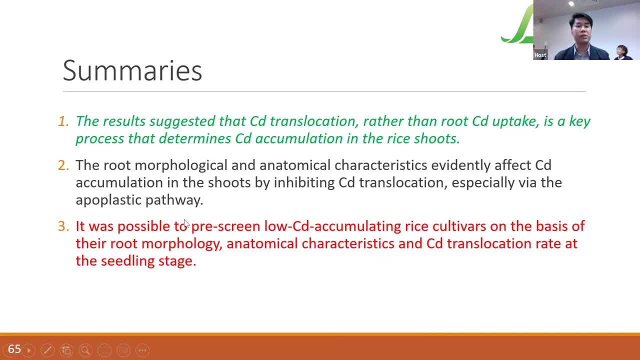 a different amendment, but instead, if we can pre-screen select a suitable, good, low cadmium accumulating string or cultivar, that would be nice enough for a farmer to adopt it, when even they found some pollutants in the soil. Of course, with the time limitation, I think I cannot talk. 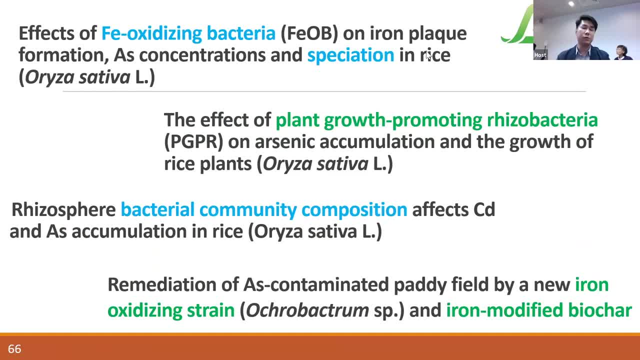 too much, but here just share with you that we also try to consider different kind of microbes, just like the ion oxidizing bacteria. how exactly working with the arginine speciation, with the organic arginine, inorganic arginine, so on and so forth. 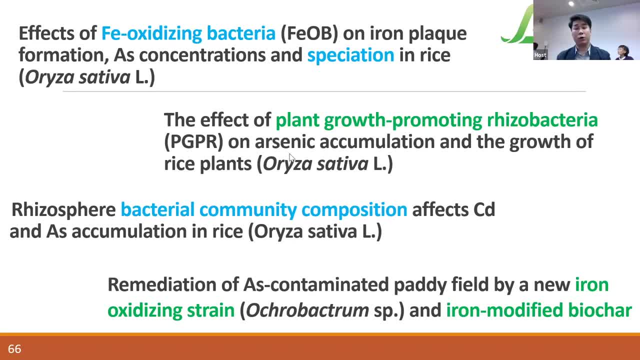 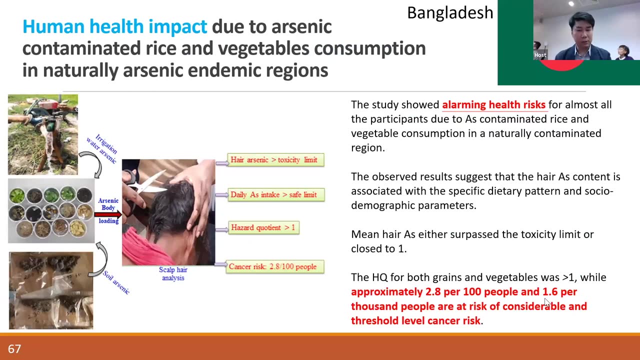 As well as the plant growth from eating rice, bacteria or the arsenic accumulation of plant growth, so on and so forth. So all these are some related research topics that you may find on the internet done by our research group, And recently we try not to just work in China. My PhD student. 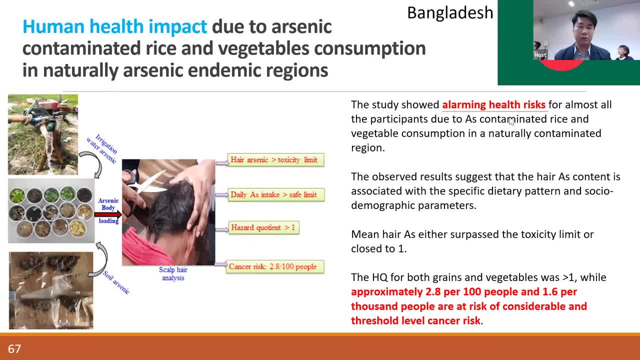 actually comes from Bangladesh. and then you know, Bangladesh is a country with quite a lot of arsenic contamination, especially underground water, And this contamination is actually not done by human activity, not by industrialization, urbanization, which is natural, natural in the groundwater. And they are colorless, taste less, whatever you boil, you cook. 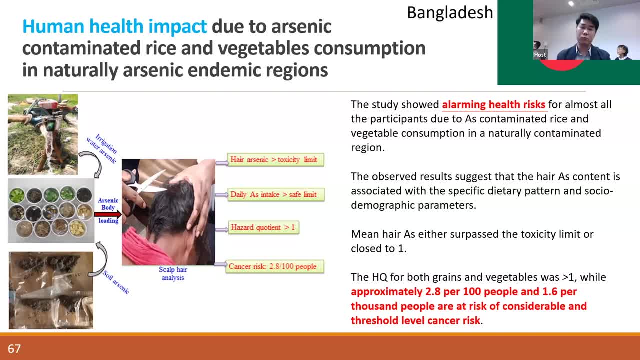 it, you fry it. okay, the arsenic is still in the food, in the water. So that's my PhD student actually, he graduated already. And then one of one part of research is to do a risk assessment And then he found, okay, the health quotient for the farmers, for the citizens. 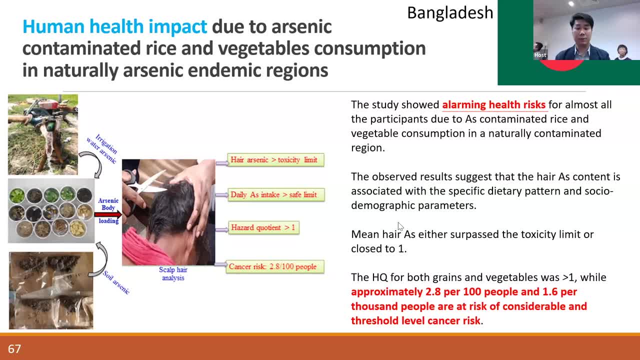 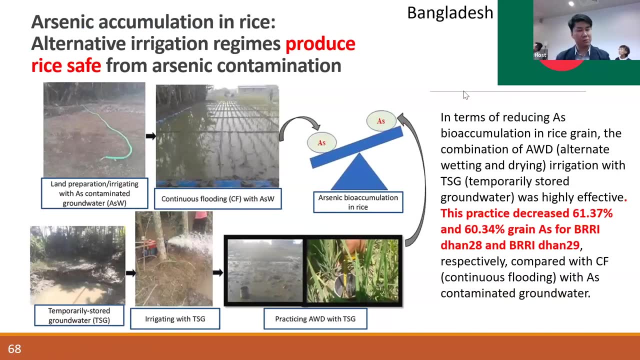 in the Bangladesh is pretty high, which is talking about 2.8 to 100 people, and those 1.6 per thousand people are at risk, so that this is actually an alarming health effect in the Bangladesh. Of course, we are not just finding a problem. we're trying to use some simple. 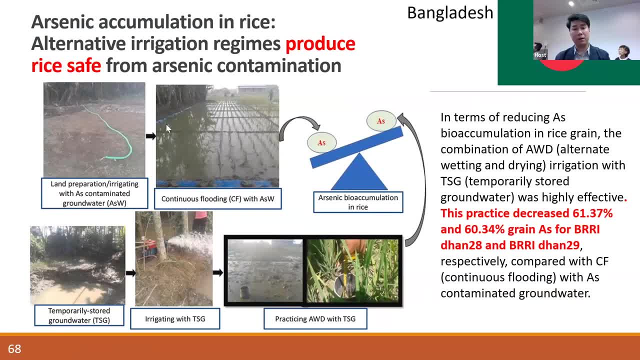 way to solve it. okay, and discuss with the farmer. Of course they don't want to apply different amendments because it needs some code, some, some, some operating, operating of course, So that we try to work with the water. okay, we have some treatment. we've got temporary. 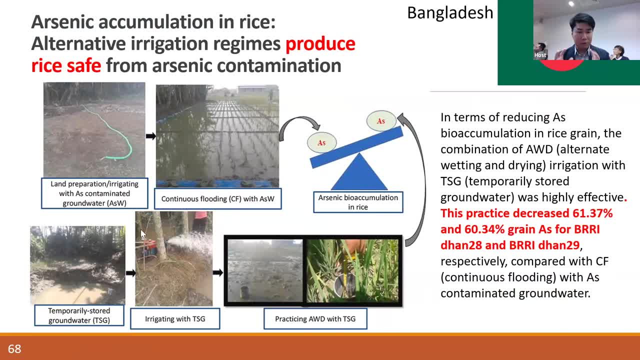 store the groundwater. we we just a simple: simply treat it, just store for over one night after those arsenic being oxidized. basically it can reduce availability And eventually we found that with this practice the arsenic being upticked by the right could reduce up to 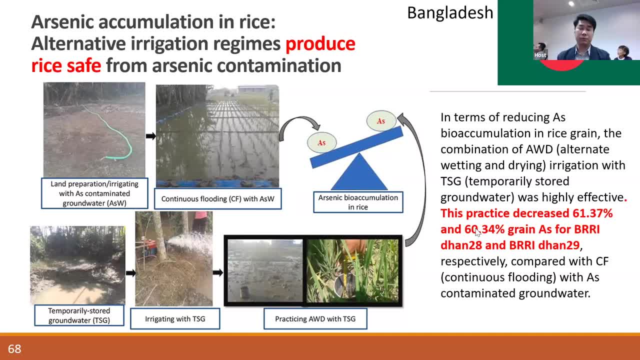 60% okay, which is also safe for the, for the consumer. So that's why it's well, well welcome, okay, well received us by the farmer in Bangladesh. Of course, nowadays we also keep working with Bangladesh and to see if there are any further. 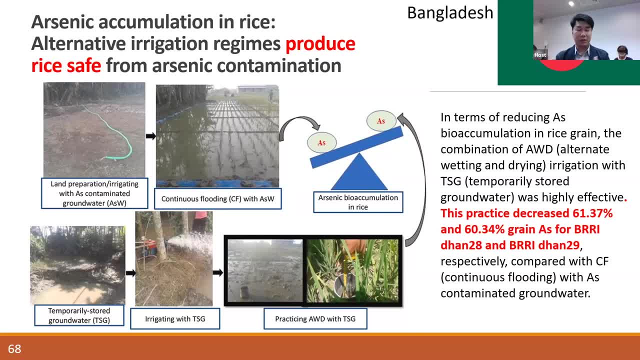 way to assist them to to come back with the arsenic contamination in the groundwater and soil or even in the rice itself. Okay, so, thank you so much and welcome for some quick questions or sharing. Thank you, Okay, so now we open for questions. 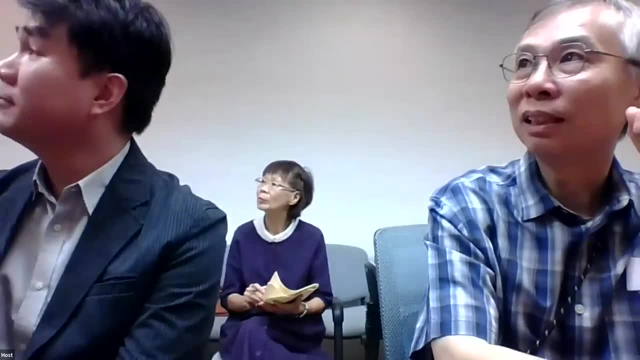 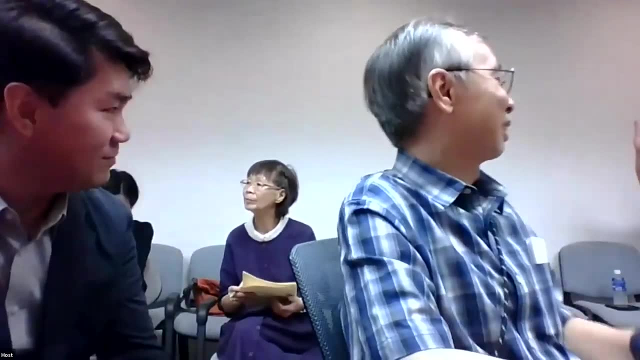 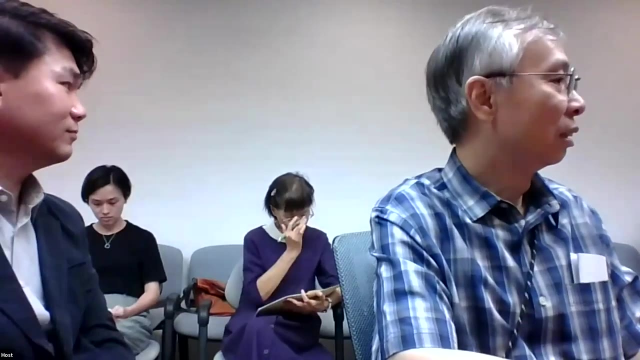 From the forum and also from the internet. So who would like to ask the first question? First of all, thank you for your presentation. it's very helpful. I just wonder how long is the period of function? for example, still select in the soil? 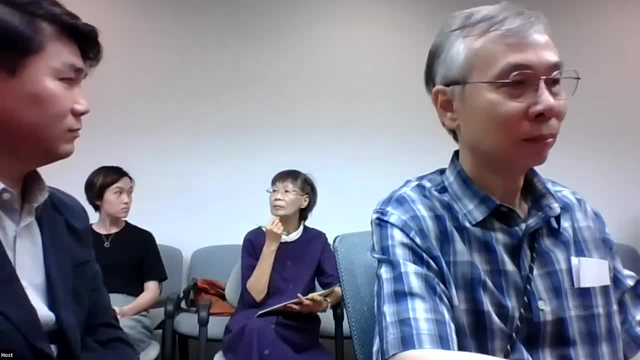 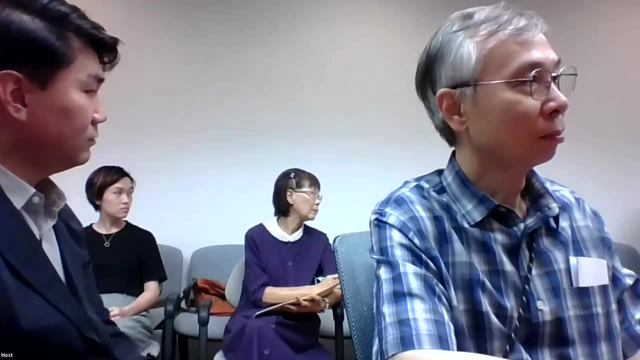 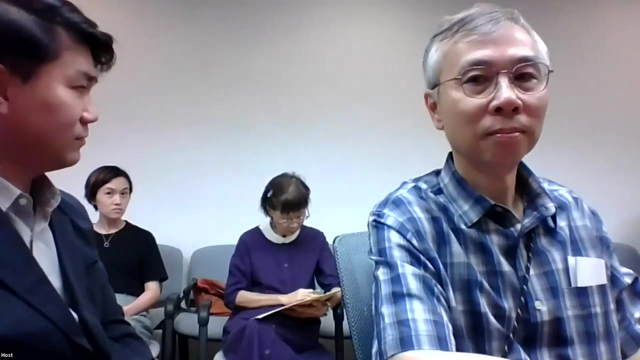 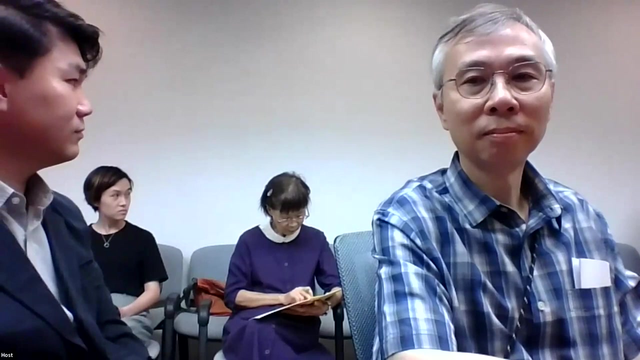 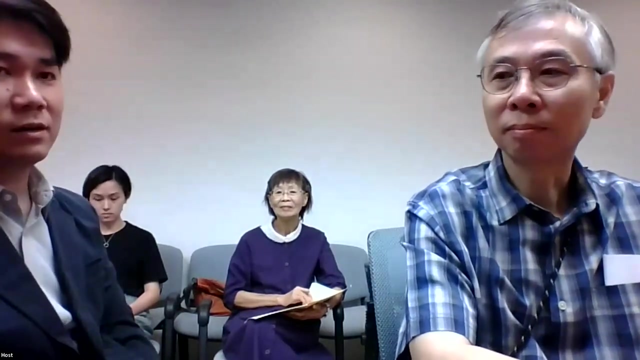 If I want to restore agricultural land which is contaminated by, for example, if we place this material in the field repeatedly, how many times do we need to restore the agricultural soil? or we actively remove that and remove this material? I see, Yeah, this is a very practical practice Normally at this moment. 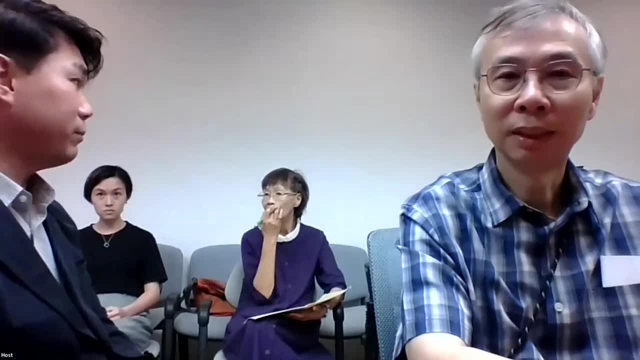 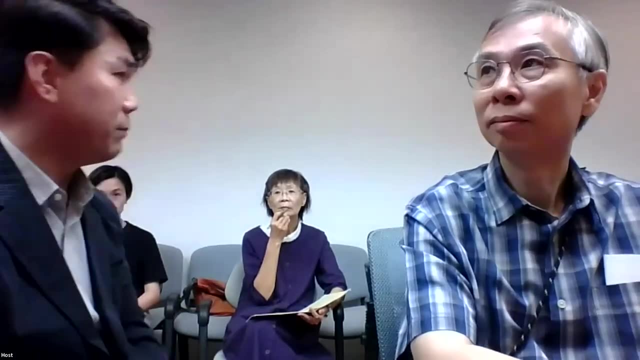 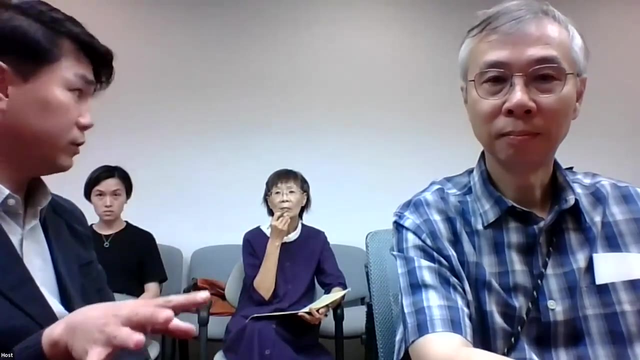 for our research. we try to apply the biochart with the rice cultivation and we normally use two seasons: Growing season and basically after. within the two growing season, the performance of the biochart or this amendment is pretty nice, but for longer seasons we didn't. 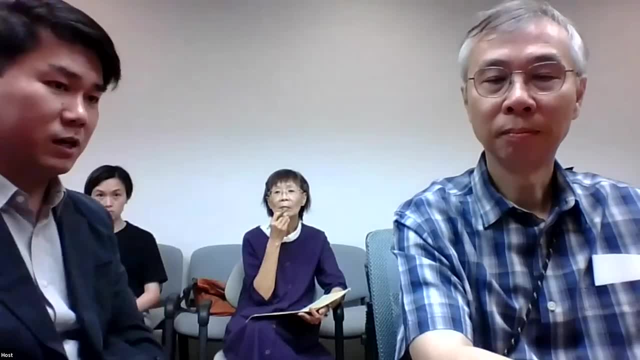 try, but for my PhD student- actually he would become a postdoc- he would consider to use four or even five in Chancellery and Gold vientia. Até 4 genocide. portalkão fica cinco. The limit there is even less than that. so because of that, all the será cada vez lebih barã. even 5, in the future of age. it doesn't need the researchers that will do the evaluation plus for some reason, and the performance of the bio chart it Dubai work is quite good, For the survey fromizes around the state. the efficiency of the biochar. but of course, if you want to ensure that you add a little bit, because one day the biochar will be somehow sick, they're using the absorption and something, but at least for two seasons it's normally okay. for the growing season of price you mean three months or 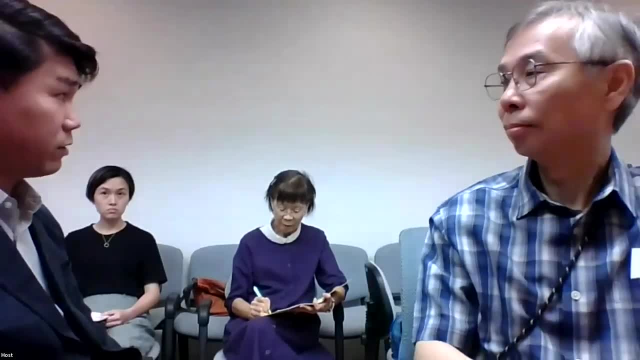 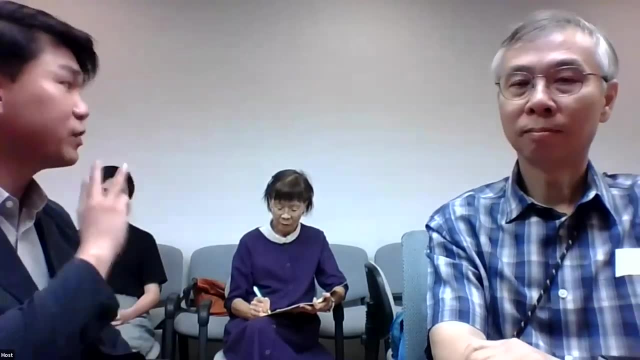 normally for for hong kong. uh, the growing season is talking about three months. yeah, in hong kong we've got two harvest per year, but in in Bangladesh or in some southeast asian country, they may have three, three, three houses. but of course, in china, just like in the northeastern part, 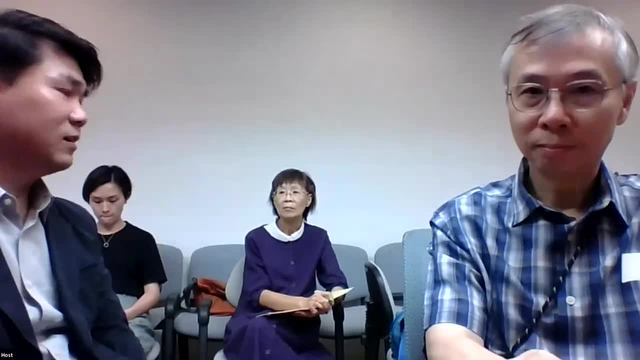 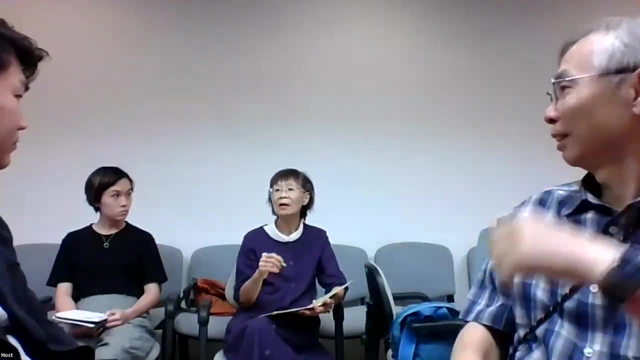 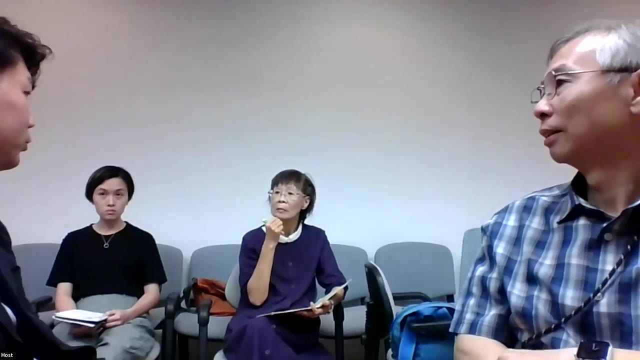 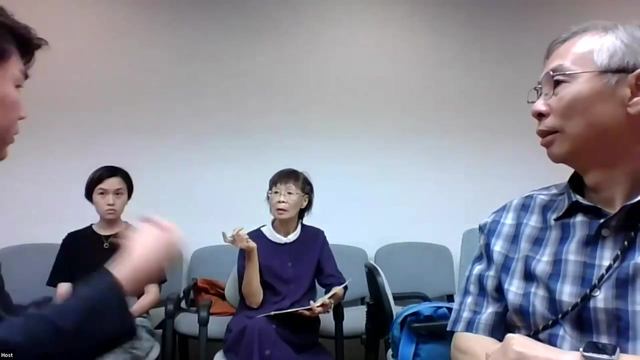 you only got one season because of the weather. okay, yes, please, yes, please, speak louder. basically, uh, we do not need to work at it. you don't need to have a gel at the same time if you want to ensure the fish, and a new one, because the biochar itself is also kind of carbon source. 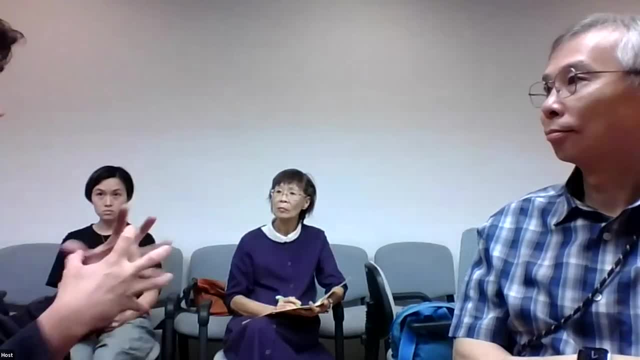 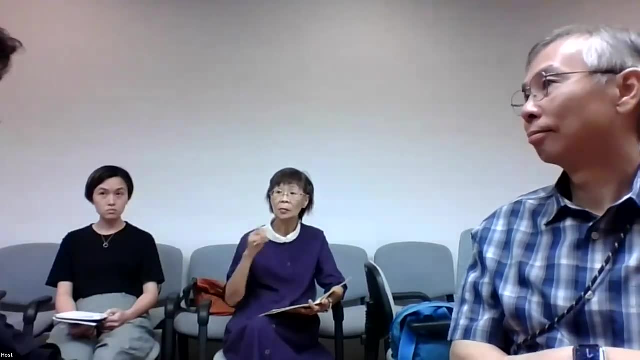 that once it's saturated, basically the metal will just lock up in the biochar and we don't need to take it out. but i know, yeah, no requirement because they are very stable. but i know there are some techniques. they will add some properties to your biochar. 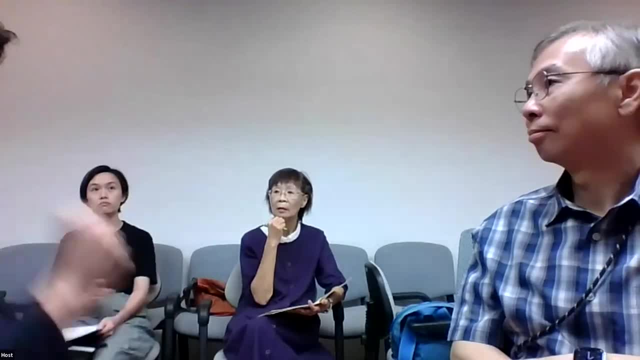 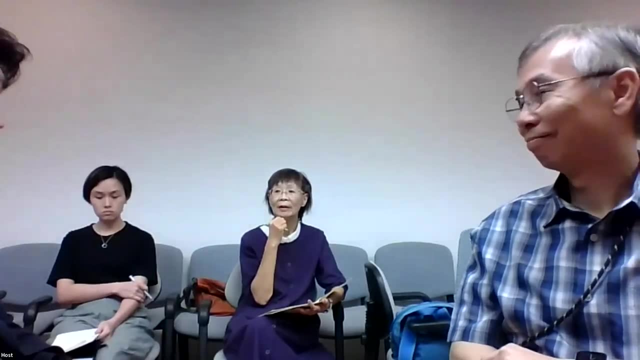 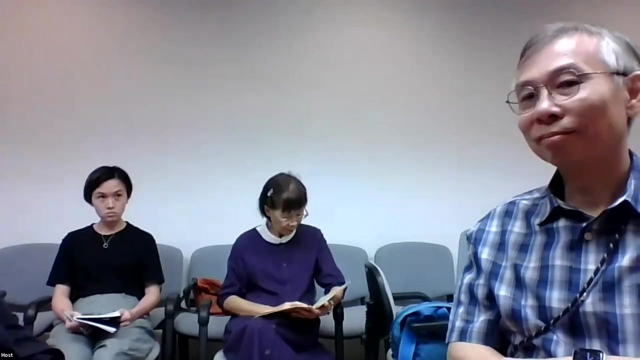 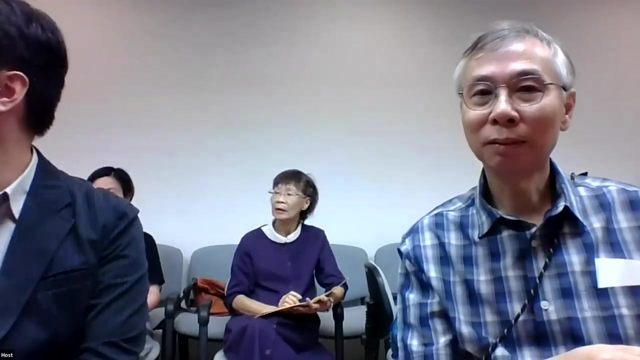 that they need some iron to just to get it out, but at this moment, for pharma, i think they don't like this kind of fertilization as far, as just leaving the soil will not further release, causing any other secondary. okay, so any more questions from the or from the over the internet? 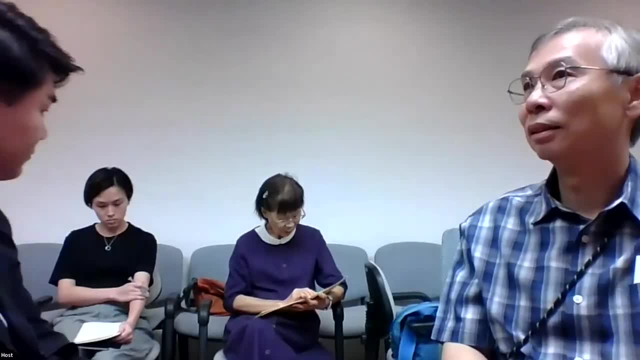 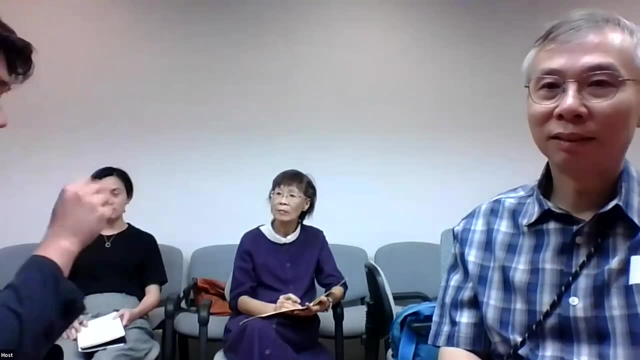 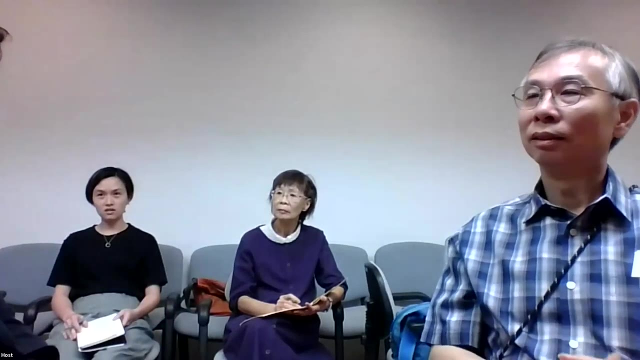 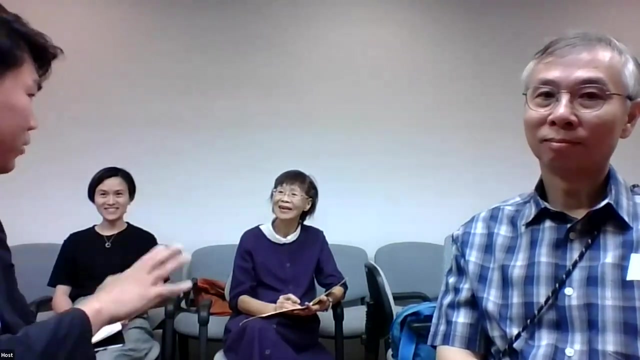 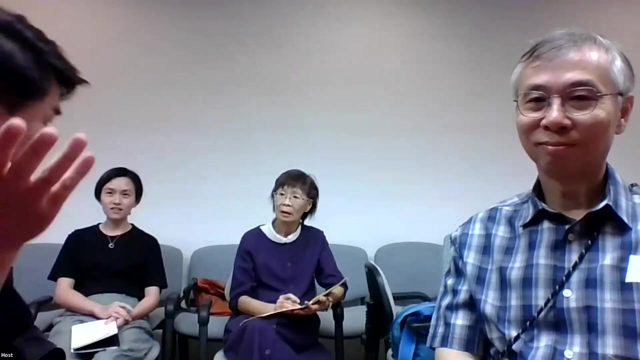 yes, yes, yes, oh yeah, just set it by friday, you know you might see the menu guys. anyway, you're kidding me. you will regret reading that, because normally when you finish studying after this- i am not talking about the other topics- we will talk about covering iron transformation, sometimes just simple пер lignan tarot books. 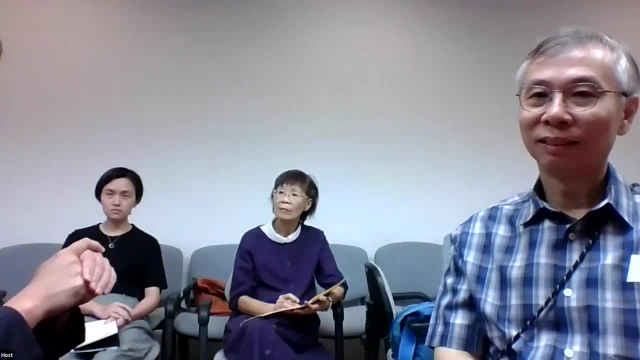 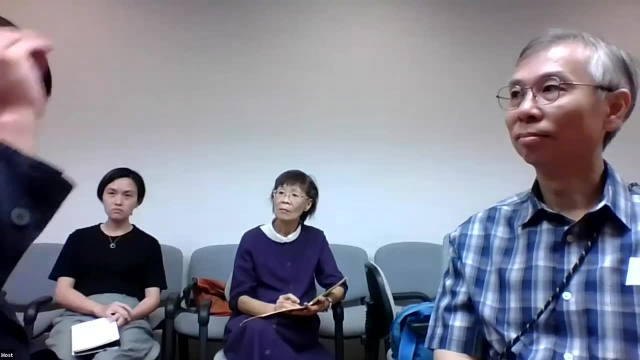 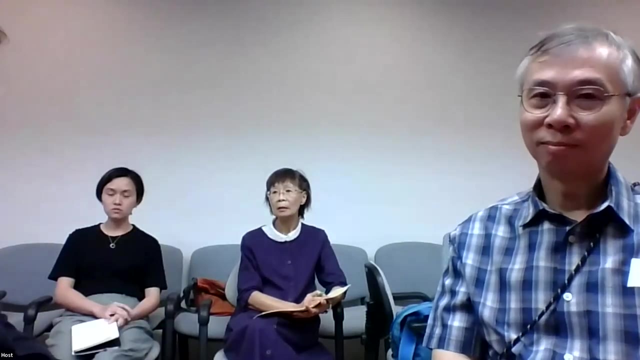 very high. uh, you can see those soil are a kind of barely no grass, no flowers. but for these plants we find something green in the soil that maybe they have some potential as a tolerance or even hyper accumulation. that will be easy, something green. okay, with the biomonic you're using, just 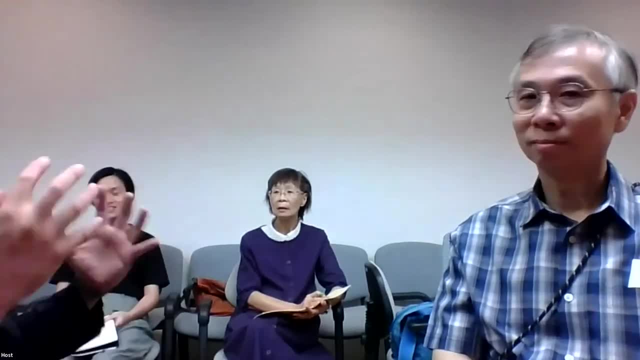 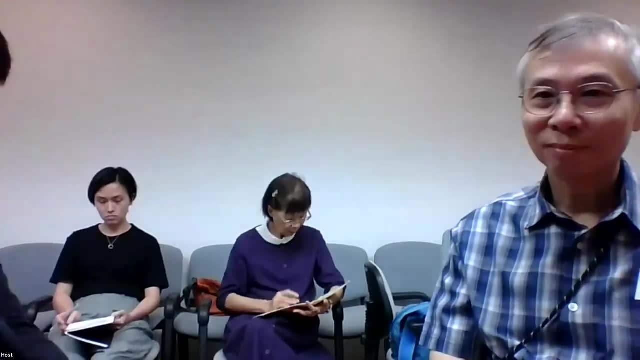 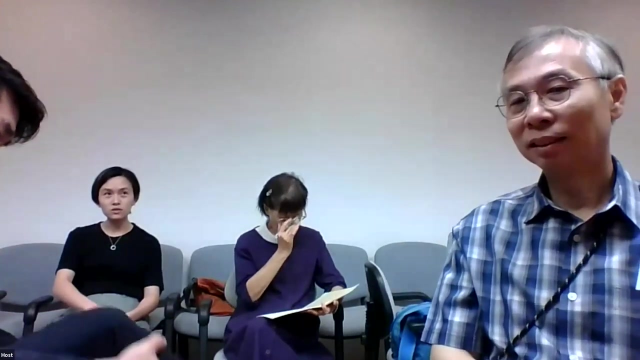 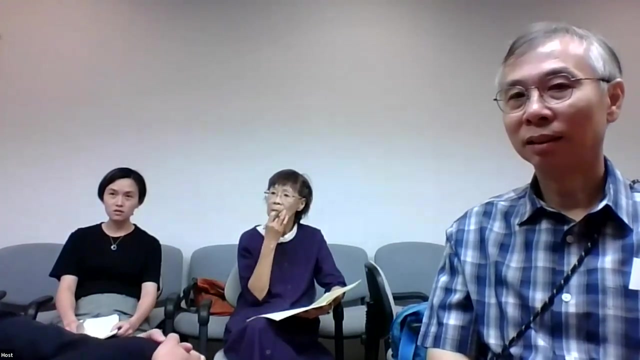 a monocular. you can find that easily so that we keep finding them for, say, one month okay, and we gather, okay, yes, please, uh, it shows like how high the tank normally it will use around 500, 550 pp celsius, uh, and they burn it in the furnace to kind of paralyzes the oxygen. 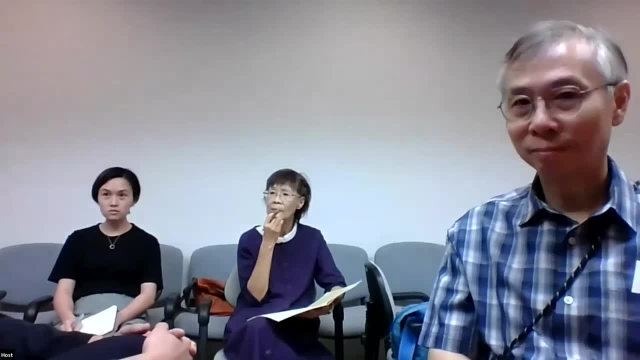 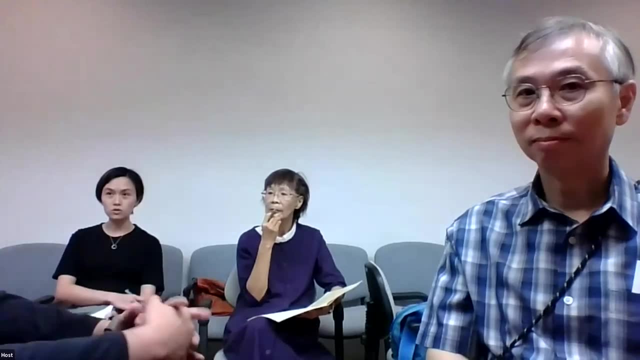 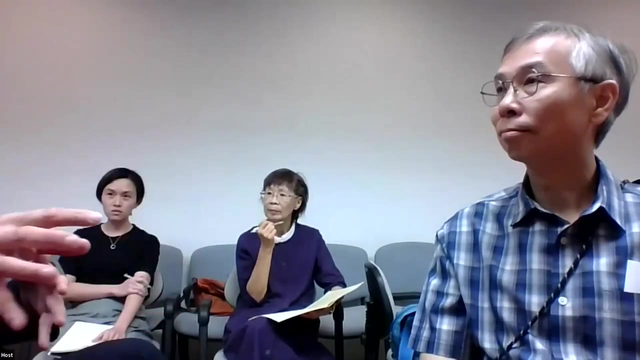 this is very pretty common, available even for some, some, for example, kfb june. of course you can also compare by 400, 400 degrees celsius, 500, 600 degree celsius. they may have different performance to characterizing, but five, five, four, okay, five hundred five inches and fifty. 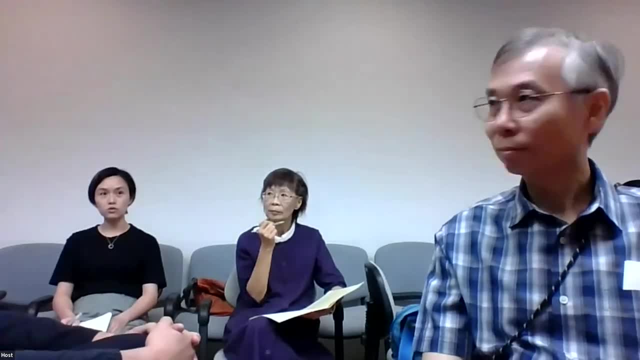 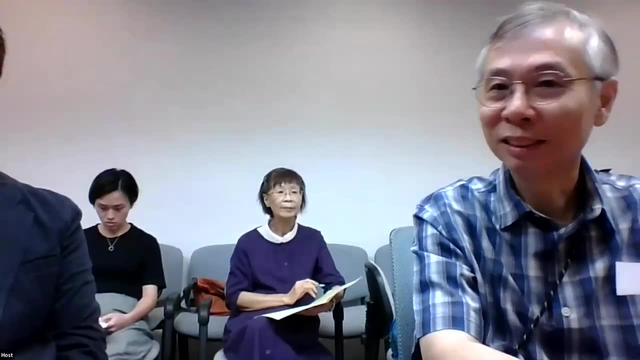 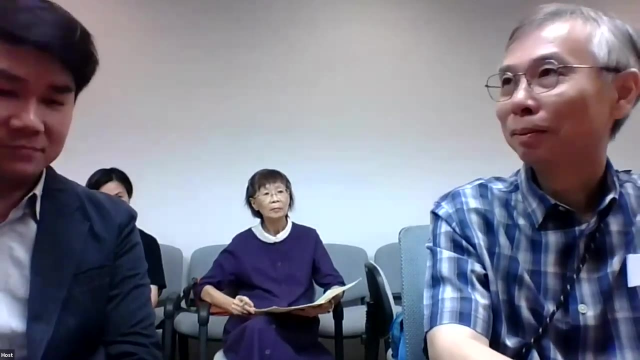 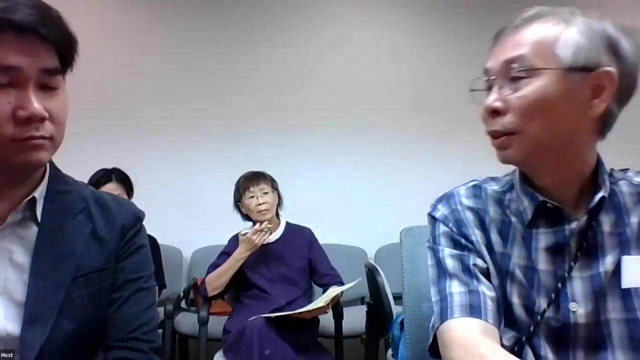 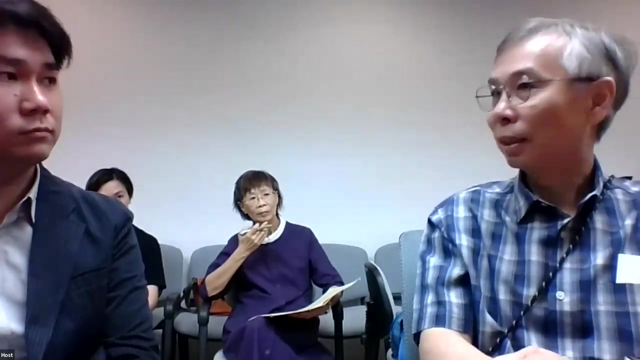 degrees celsius with the back, okay, and any questions from the internet. i want to share some of my opinion because, um heavy metal contaminations, um, some are due to industrial pollution, right, such as cadmium. some are literally occur, like, for example, aluminium right, so there are the most abundant elements in the earth. 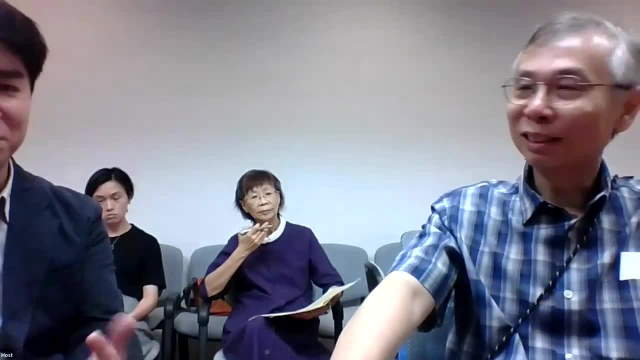 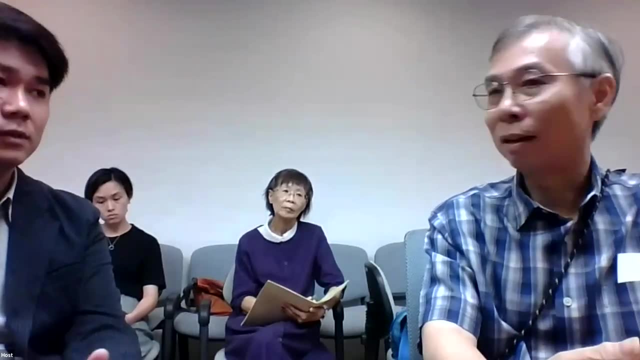 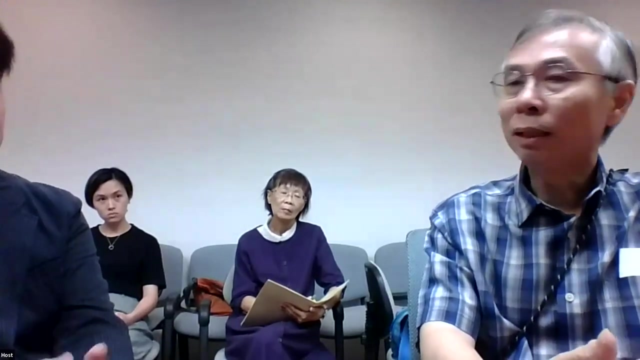 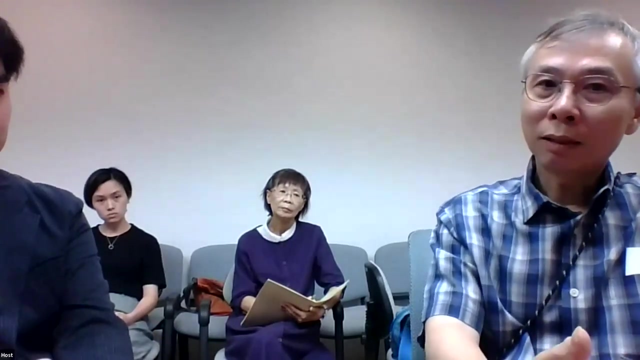 but they are not available most of the time because they oxide, yeah, but in acidic soil the heavy metal become more active and available, right. so when we, when you talk about the rise uh contamination, it's mainly in the southern part, southern provinces. right, the why says this uh, this problem? right, but i think there is a lot of um controversial approach. 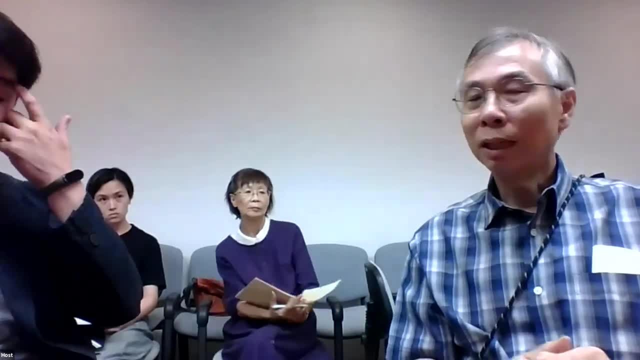 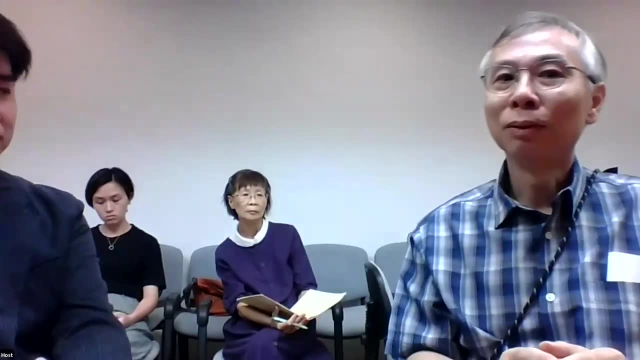 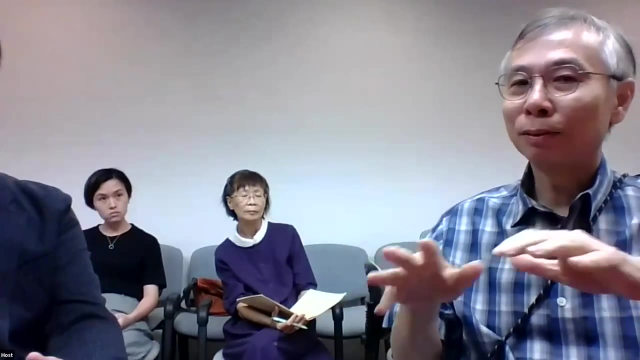 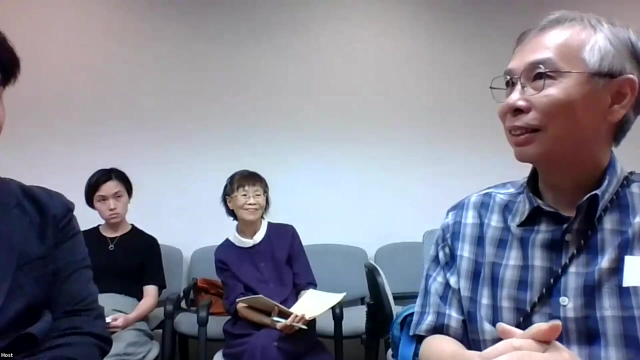 because cadmium uptake is also related to other central mineral. yeah, this thing is important, right so. so when you're trying to manipulate those to make it uh less the roots, is less uh available for metals and water, whatever? well, on one hand, you cannot achieve uh reducing heavy metal, but on the 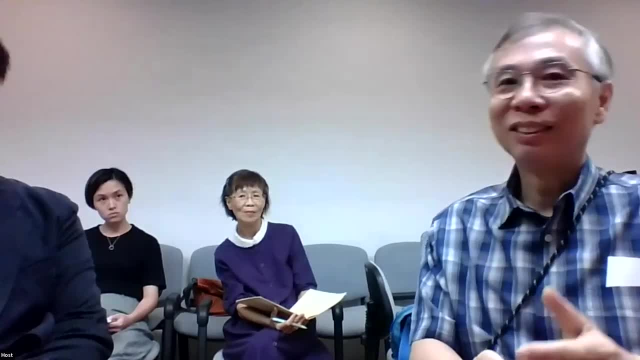 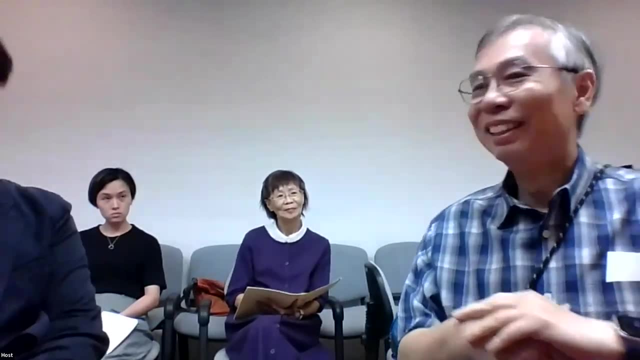 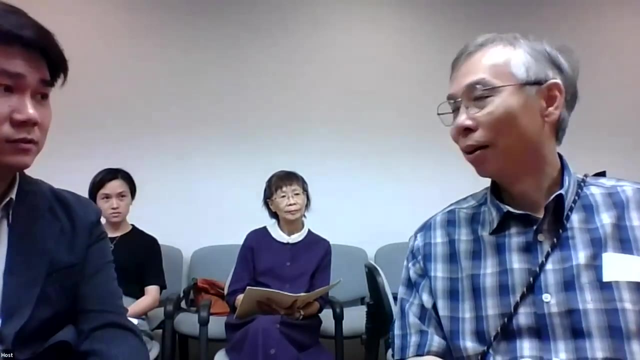 other hand, you may also reduce the use, right? yeah, so i, i there's, i work on heavy metal when i'm a master student, so at that time i started to work on heavy metals and i'm a master student, so at that time i i found a different mechanism from from a glass, of a stupor block, okay, which is a grass grown. 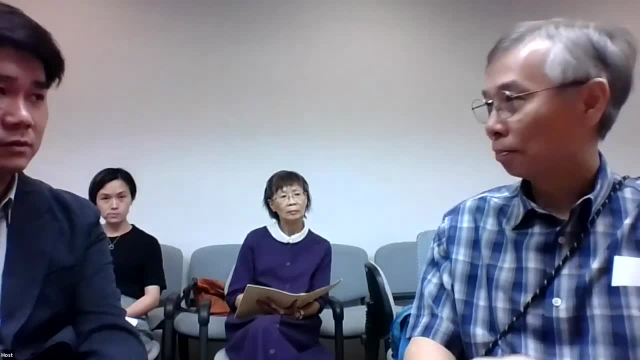 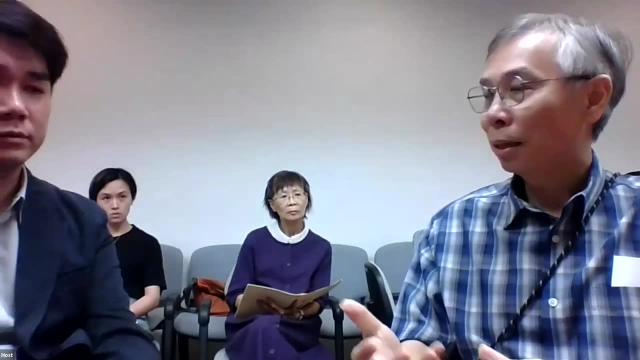 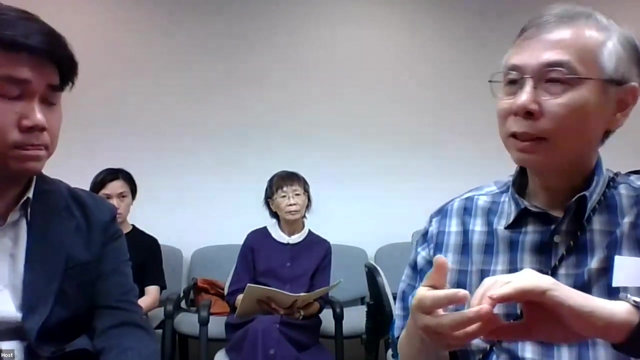 in the in the metal mine region in the uk. so they're also hyper accumulators, but they are accumulated in the roots. oh okay, you know, i hit the alphabet's tissue without transporting up to the upper parts, and i have some um evidence showing that they have some phytokinesis. 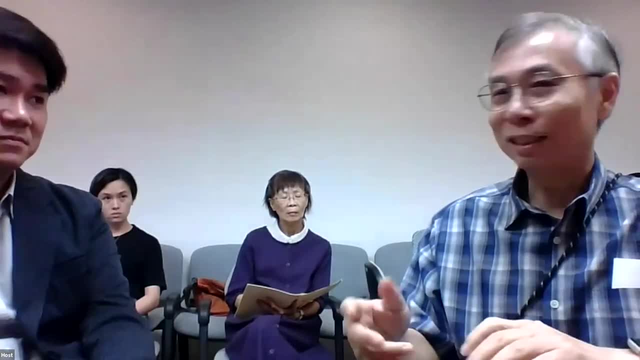 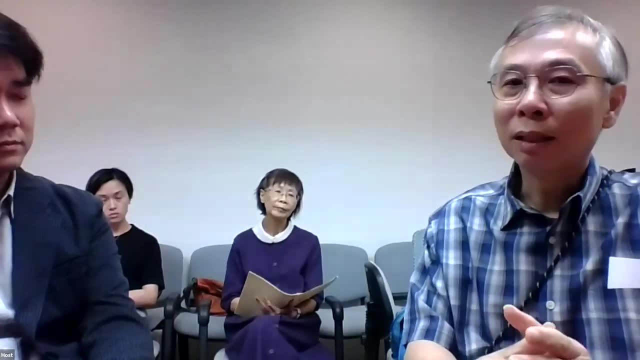 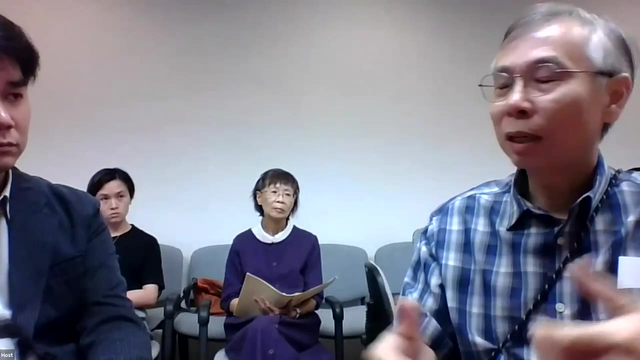 which that that the trap everything in the lower part and then that the other part is going heavy. yes, so, so there are some mechanisms like that, and also maybe a mechanism like the, the roots morphology that you mentioned. right, but what? how about? um, if you just want to help? 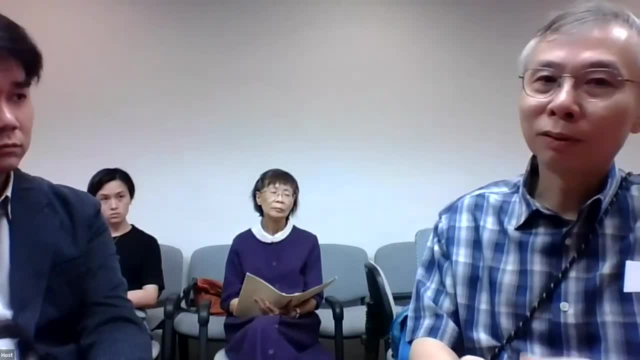 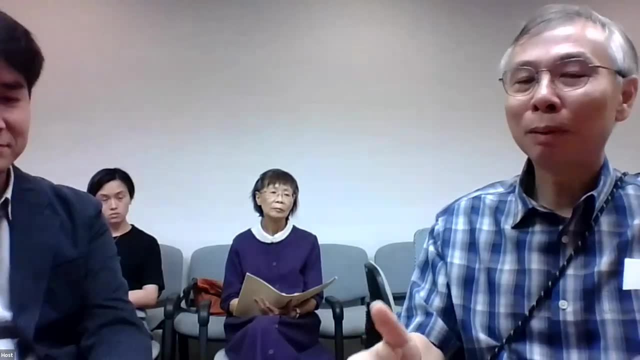 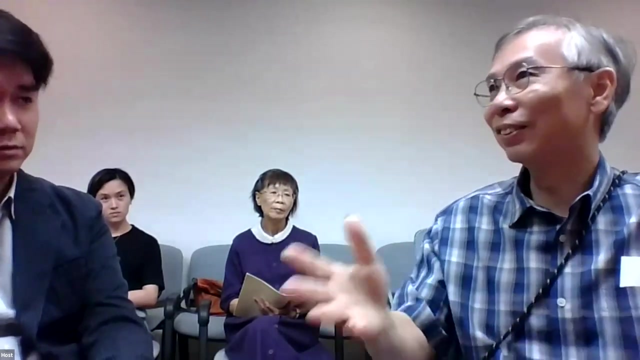 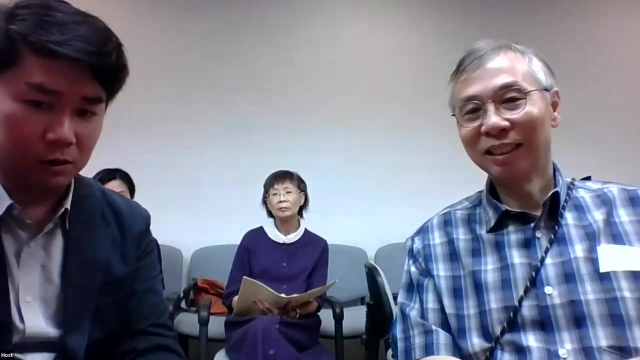 the farmer. so how about just screening for the rise that accumulate least? yeah, heavy metal, and growing the best right, because there may be multiple um mechanisms. so if more practical right, just go to the field and using a germism to screen will be more practical for the farmer. yes, of course this would be the most easiest way. just screen those. 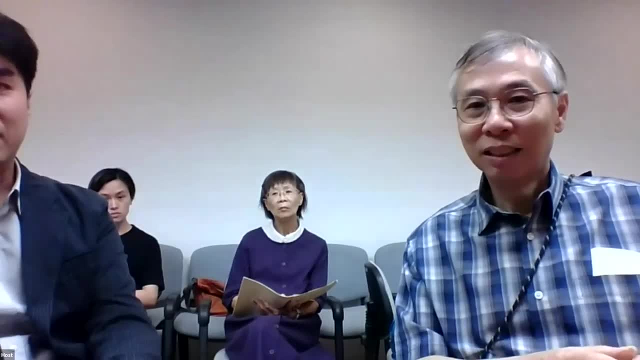 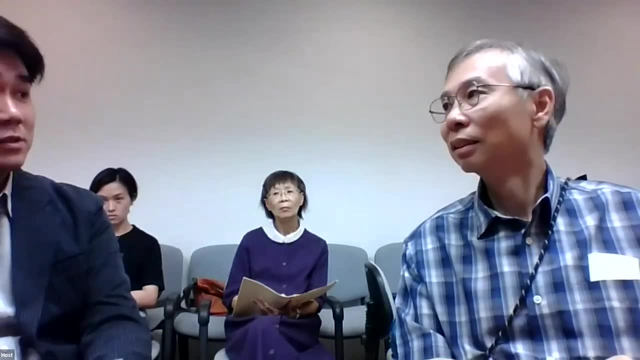 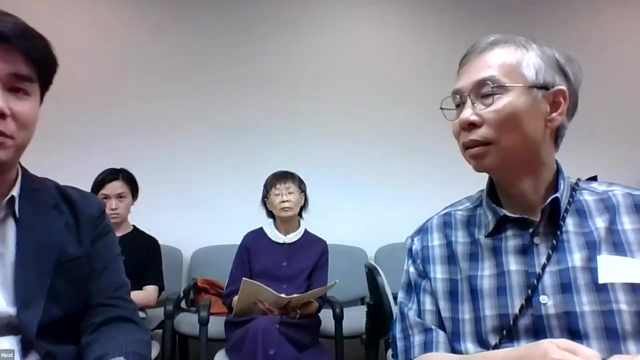 rice cultivars with no accumulating. but of course there is a dynamic: no accumulation versus the yield. let's see how the farmer will consider. they prefer to provide a safe rise by high yield rise and the same type of contamination. because nowadays when we talk about human health, 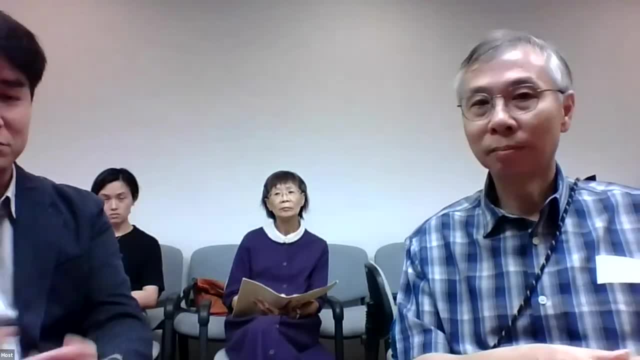 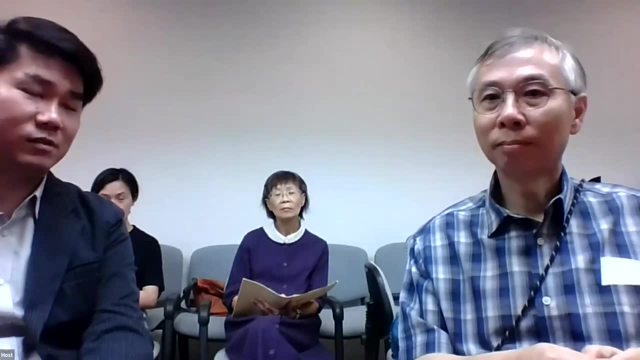 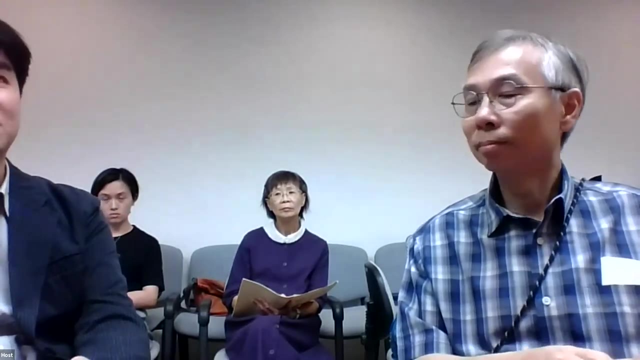 we are not just talking about the yield, because they cannot be degraded in the human body. so we will somehow consider having a concentrated. just let me be. i know in hong kong that we have some brand, five users and so forth. if we can also do some screening to see if i use a? 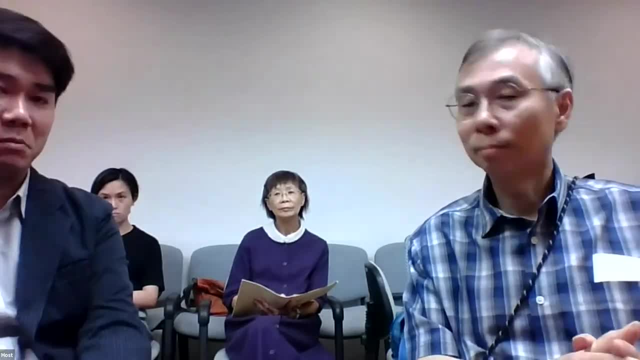 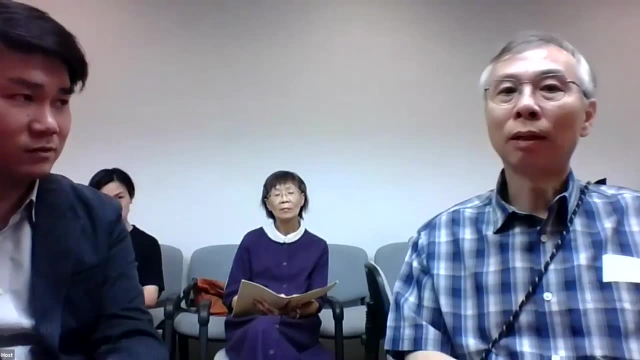 low, okay, or even high, accumulator. we are doing different from hong kong, or even not. you go to, uh, Australia, so, as we went, there is some open space, so i'm just showing what we can do, so that's, that's okay. whatever you want to do, i think we would just go and read about it. 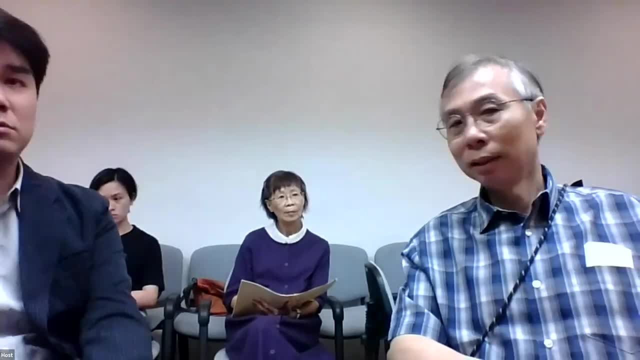 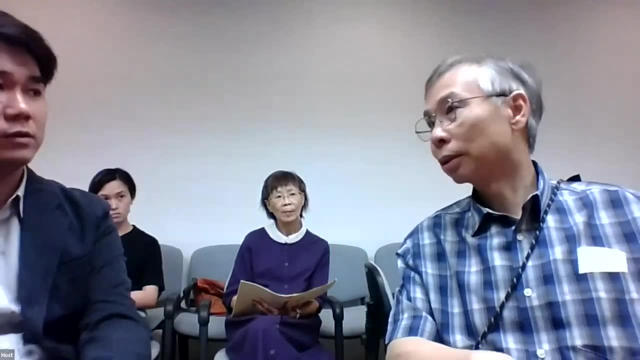 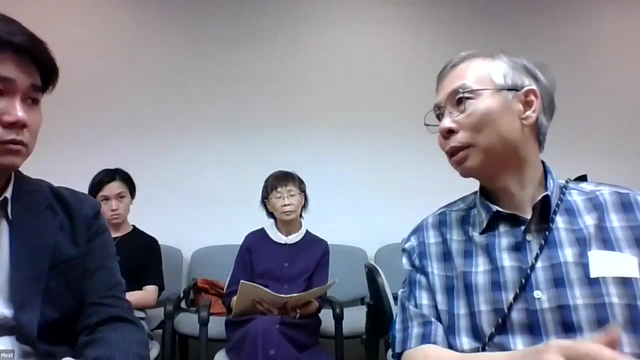 it's also important to map the contaminated sites, because if we can map it into our assessment of any metal, then we can have a better plan of agriculture. right, okay, map it. yeah, because, uh you, But some crops accumulate much less than this. Well, first, of course, I think, growing rice in the metal mine. 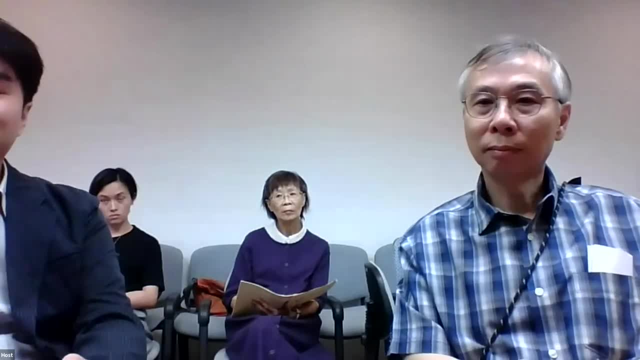 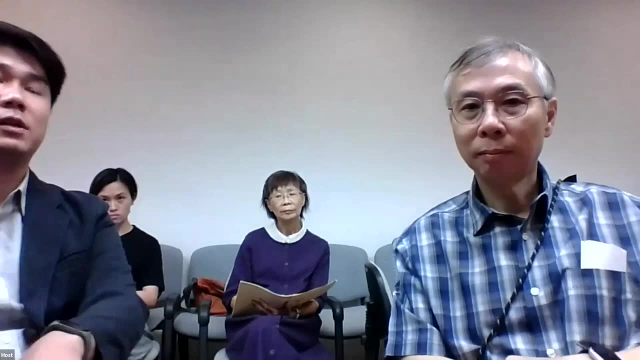 is not our first choice, right? Because this is somehow impossible. But somehow, you know the rice, I mean the farmland in my research. basically, they are not in the middle of metal mine, They are just around the metal mine, especially the first part. 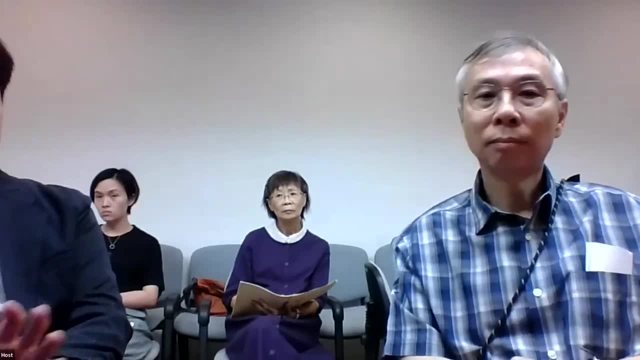 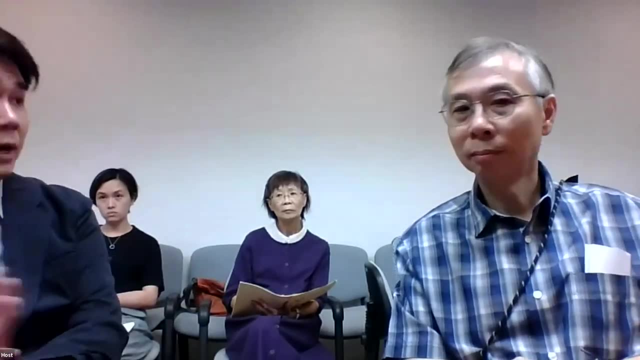 the Guizhou metal mine containing cadmium and mercury, which is talking actually about one kilometer away from the metal mine. So that's, I think, yes, we have to do a soil map, okay, For example, to see the metal concentration. 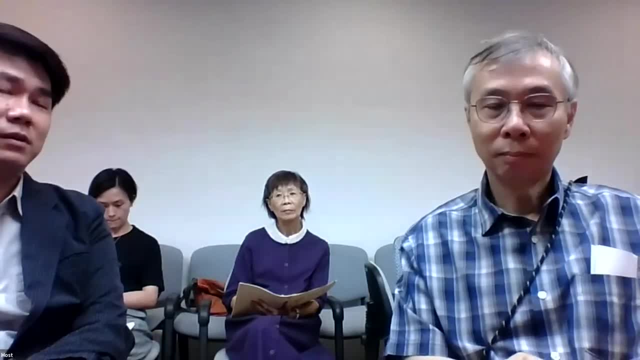 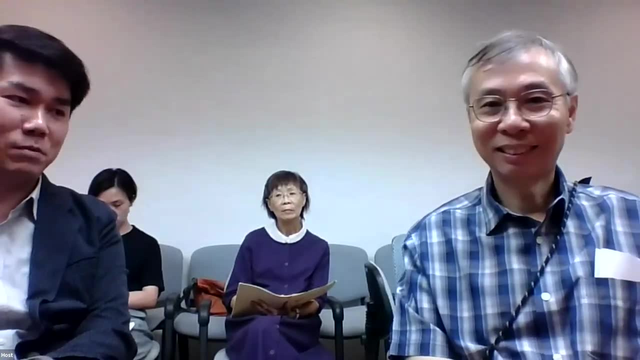 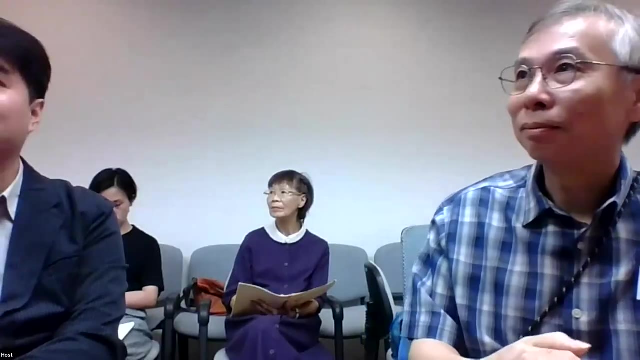 in order to find a good place for the plantings. But first I think we should not grow the rice in the metal mine, I think. even if we grow it, I think no people would like to buy it Any further questions. I do have a question. 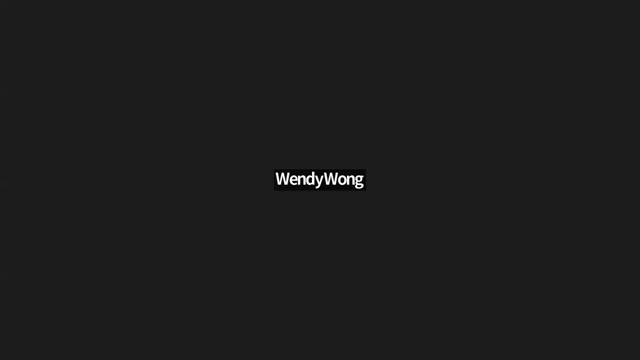 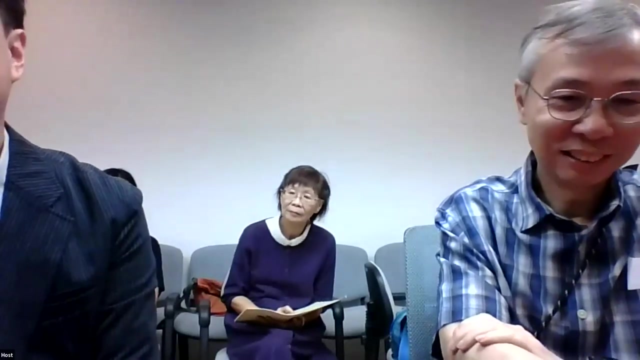 Yes, Mandy. Yeah, Is it possible to grow hyper-accumulating, you know, the cadmium plants with the rice together, so that one plant will actually soak up the cadmium while you can grow the rice as well? Right, This is a very nice idea. 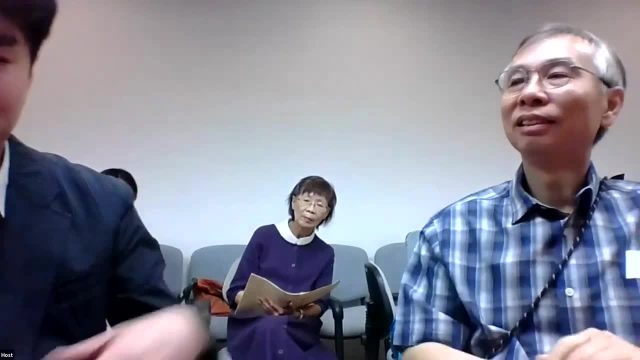 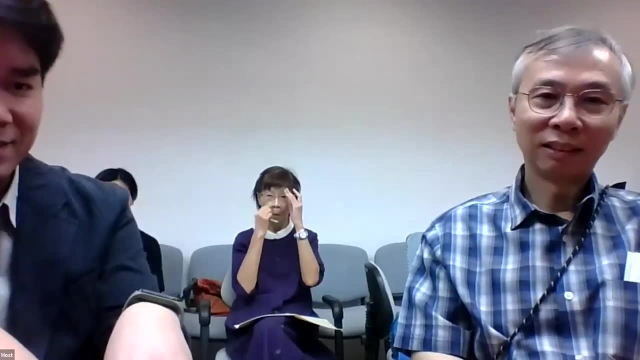 In old days we have similar concept. That means hyper-accumulating rice. hyper-accumulating plants grow with the rice. Let's see how they're competing. okay, Competing and uptake, But it seems not easy because for rice, 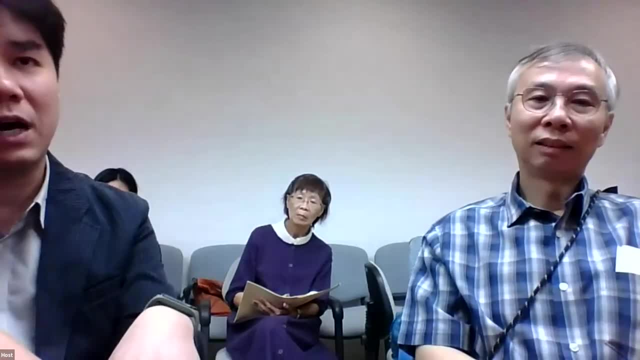 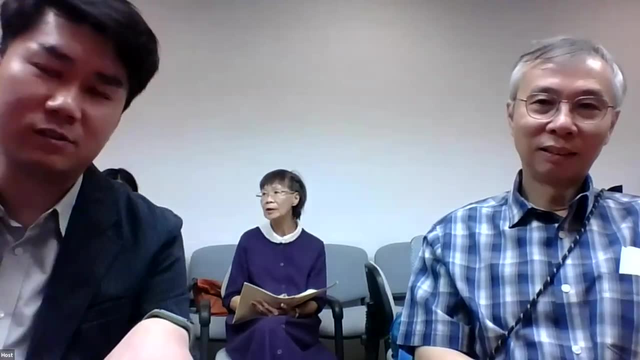 the growing condition is flooding. It's flooding And most of the hyper-accumulator- so far we know they somehow not growing well in that flooding condition, So that rice is a kind of a loner. okay, They can't grow well. 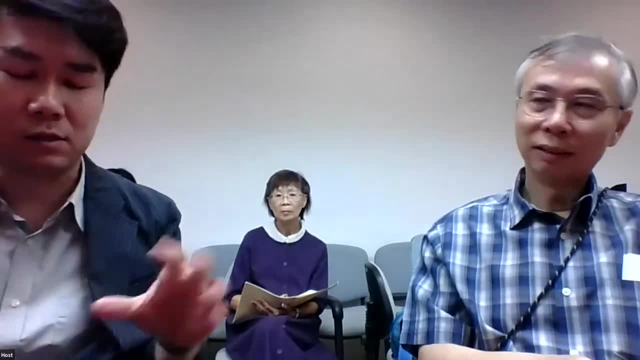 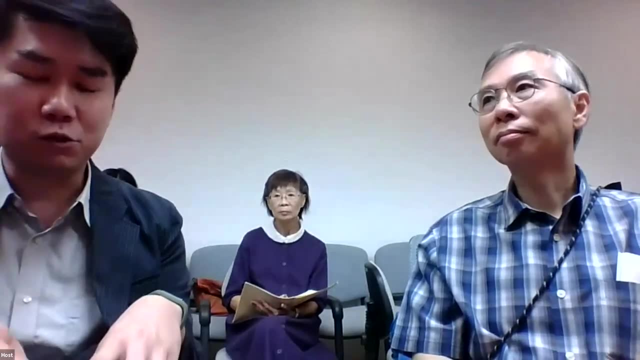 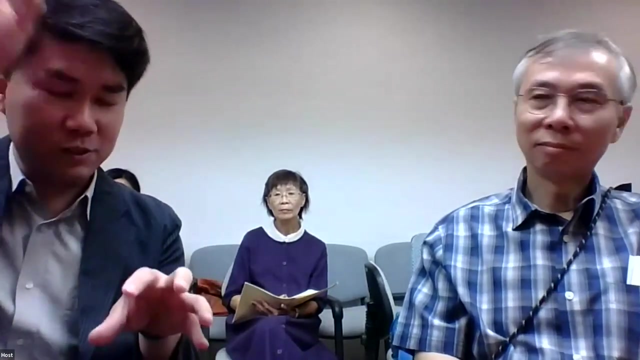 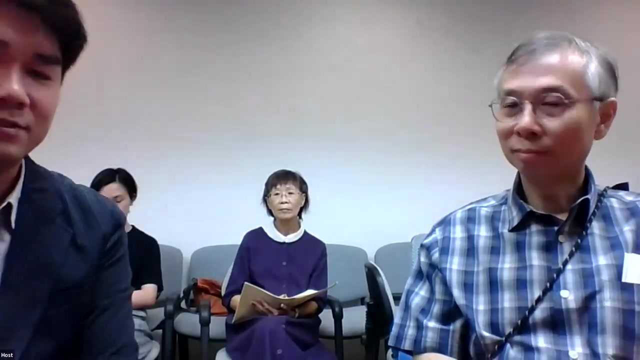 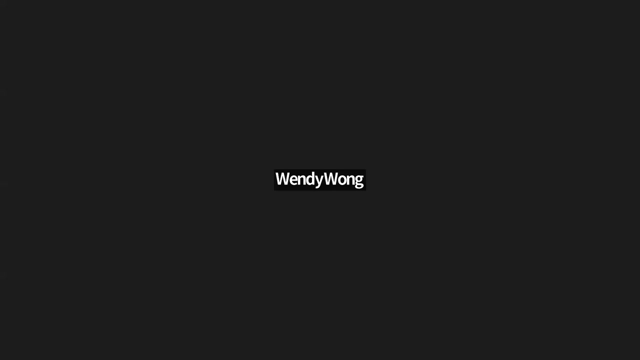 They can't grow well in the. This is nice for maize, but not for rice, basically, Okay. So one more question is that after you keep growing all these hyperaccumulating plants, it actually will help you to clean up the soil, correct? 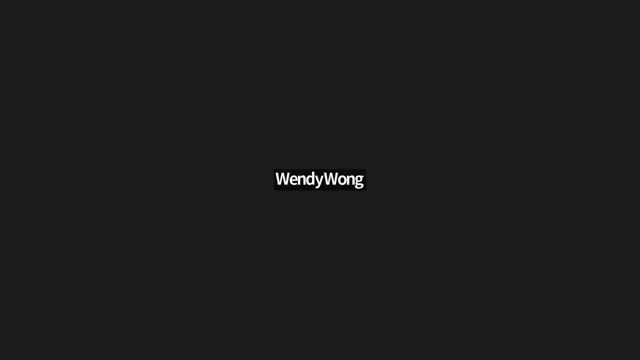 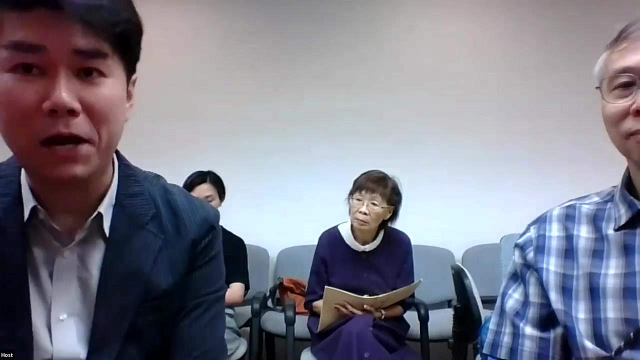 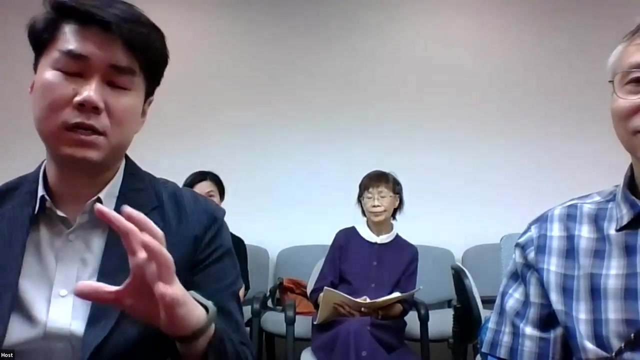 Right, Okay, so eventually the soil will be good for any. you know any crops, Right, but you know there are some limitations. It takes a long time, talking about five to ten years, and we have to remember that if the rice, I mean if the hyperaccumulating plants, especially the root, 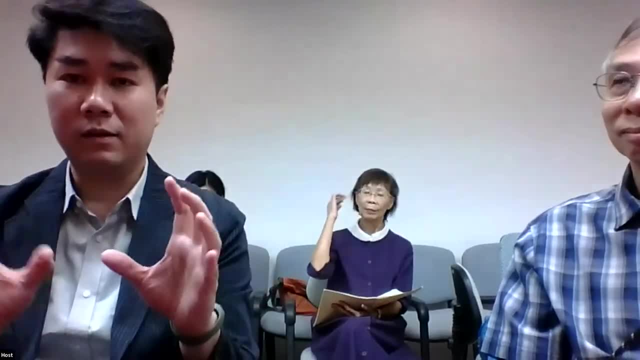 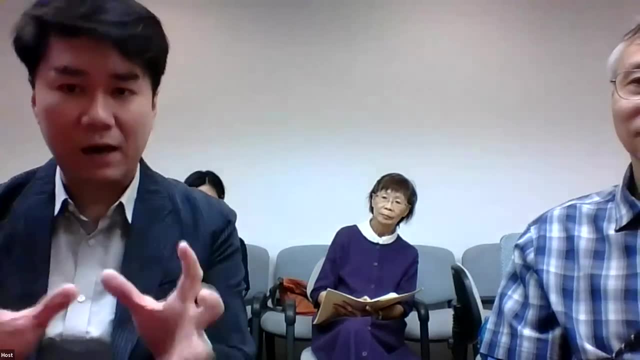 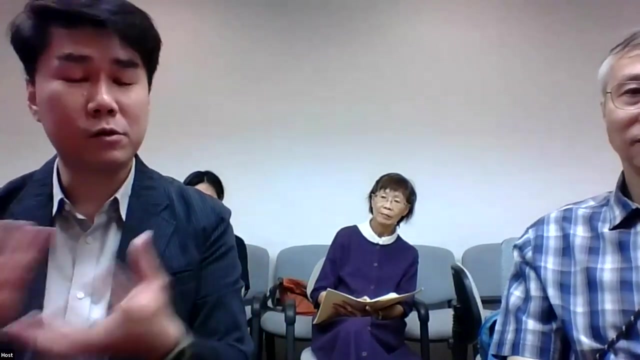 if the area of the soil that is not being contacted by that plant, then the gluten somehow could not be easily being uptake, so that it also depends on the plant size. That's why we have to use a long time to do for the, for the, for the cleanup, and also in the middle we have to mix. 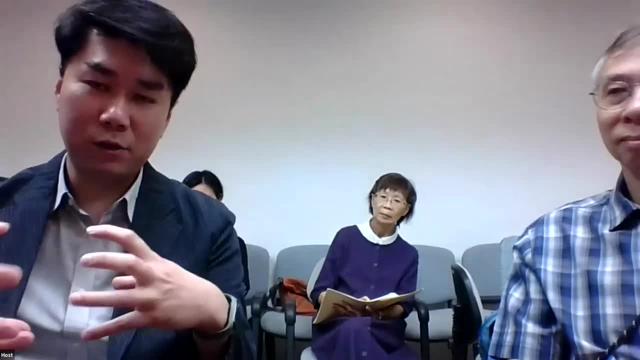 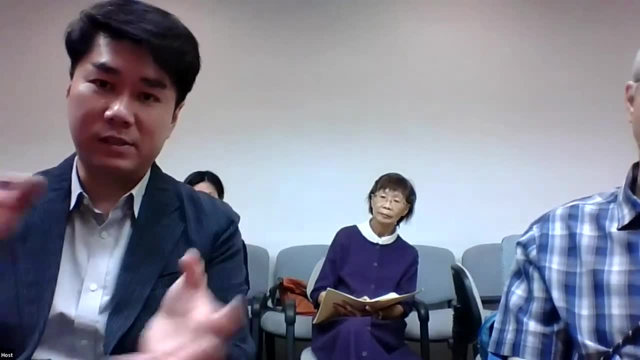 the soil, okay to ensure. okay, the metal is well okay. it's in a good condition. okay instead of you know it's in a bad condition. it's in a good condition, okay, instead of you know. 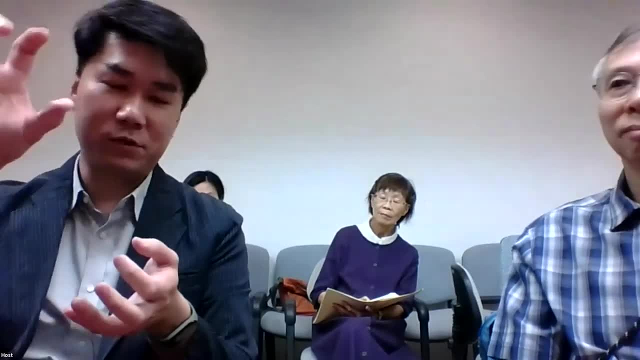 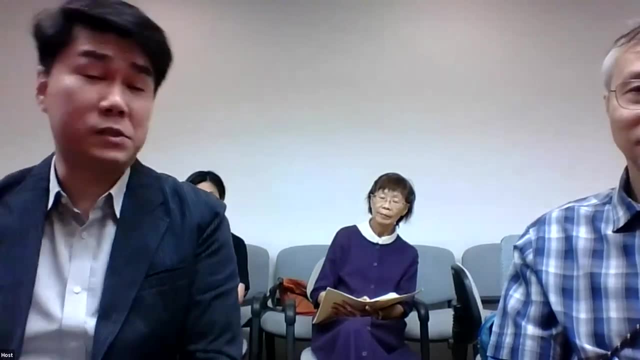 instead of just: oh, the shallow depth is being cleaned up, but most of the heavy metal is actually in the bottom, so we have to make it uptake down and also be uptake again. so it's also a manpower issue and at the same time we cannot do anything. no, aquaculture. so that's why this phytoremediation- 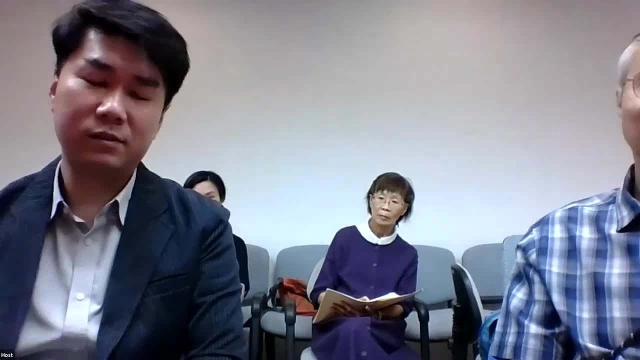 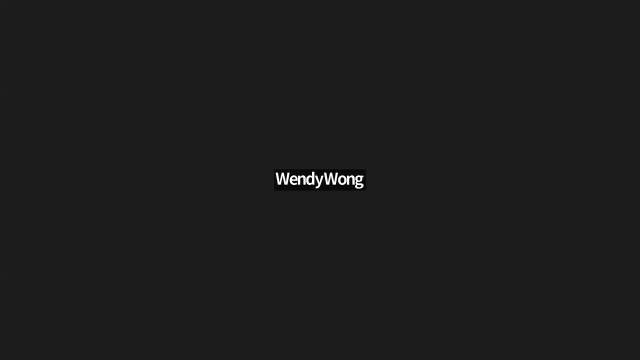 somehow I would not encourage for the farmer. But now you did mention something about the hyperaccumulating plants. is that once they accumulate the heavy metals, you can actually mine the plants for the metal? am I correct? Right, right, it's vital mining. 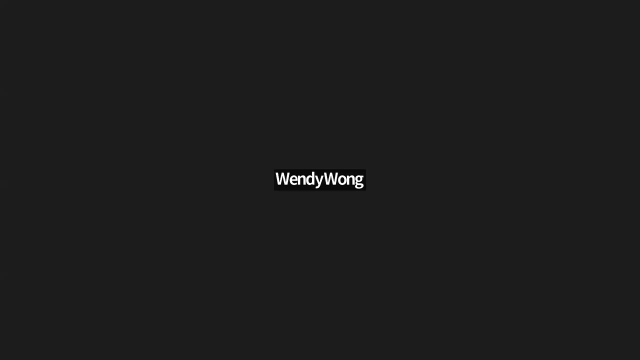 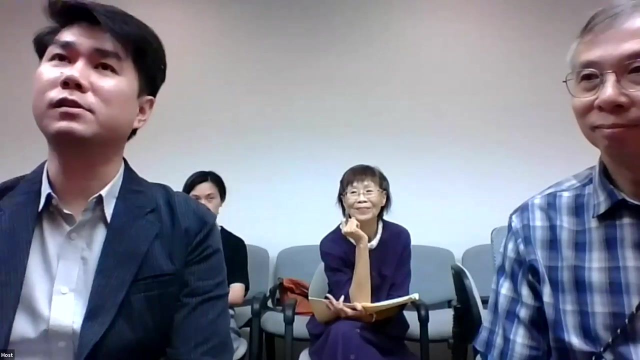 So is it possible that you know, instead of the farmer growing that, and if they can work with some kind of mining corporations, then they could have a good livelihood instead of going in and at the same time clean up the land? Oh, this is a nice idea. I never thought about it, but well. 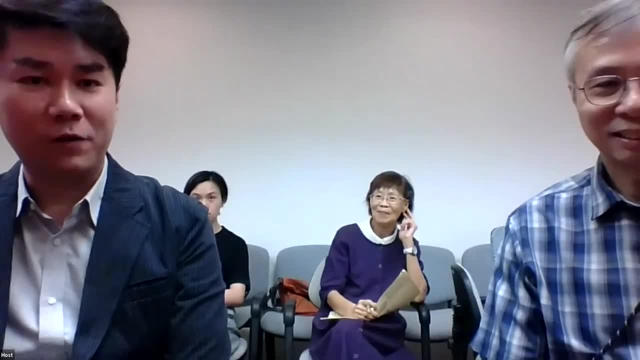 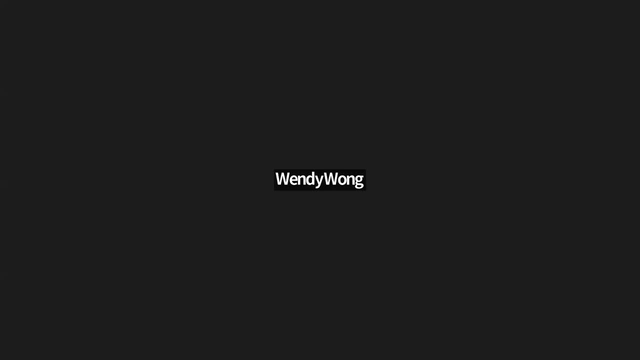 they could somehow get money, but they have to wait for five to ten years. Yeah, but five to ten years is actually not too long. when you talk about you know it is long in short term because you know when you're looking about money and income, but then in the long term, for any business, five to 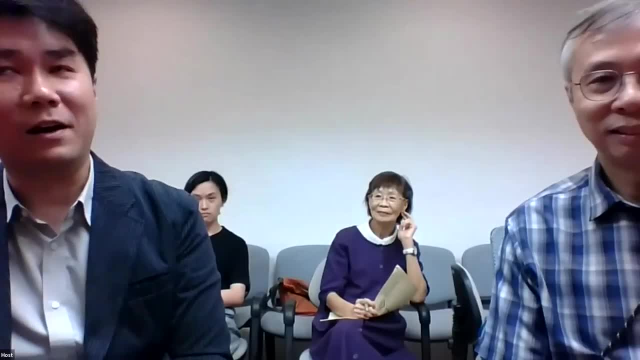 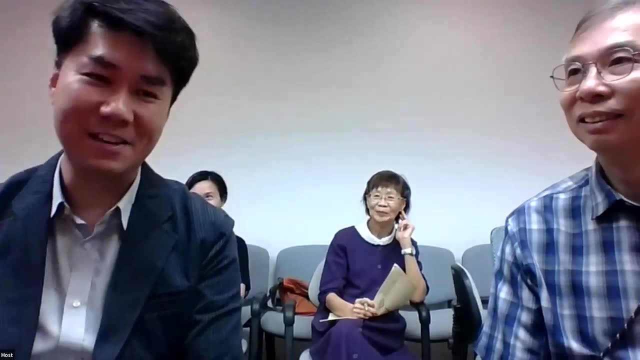 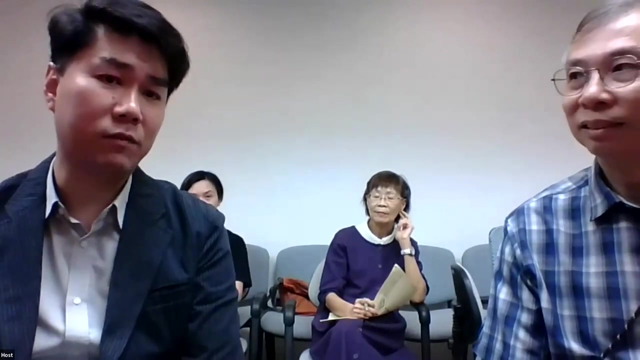 ten years is not long at all. Right, right, I think in an economical perspective they might be feasible. I didn't think about it. I think it's a good idea. maybe we can. we can think about it by estimating the amount being uptake and also calculate the efficiency. 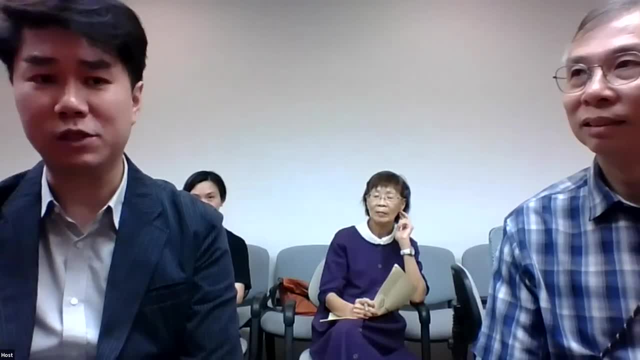 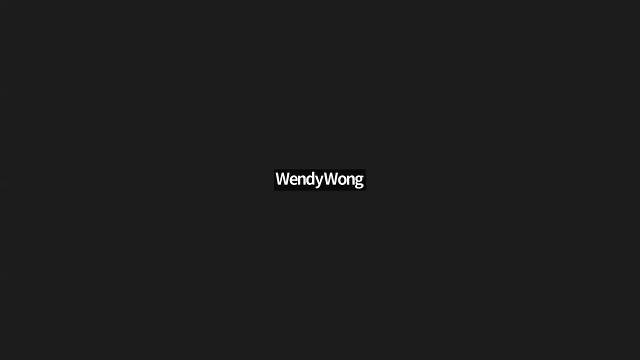 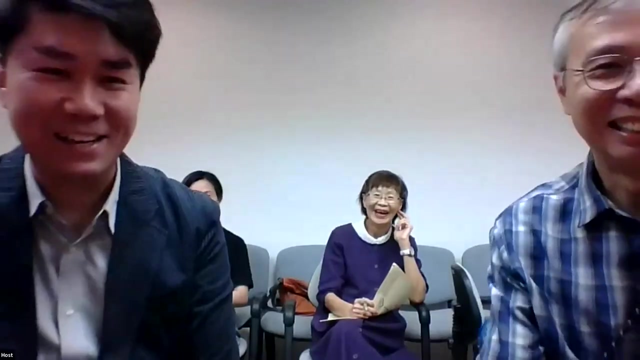 whether it is feasible to get the money instead of just farm, instead of just. I think that would be a you know for your research, for your PhD students to look into it. All right, thank you. thank you, nice, Maybe you get money, Yeah, yeah, yeah, I can get some money. 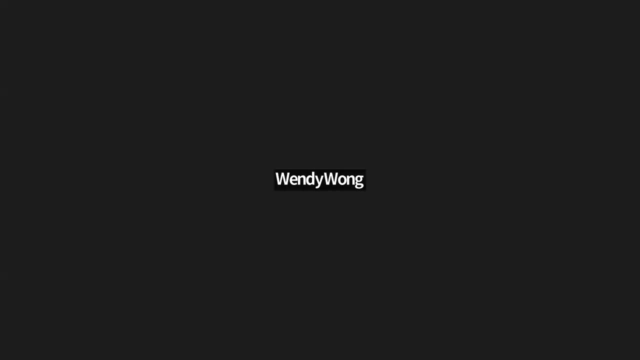 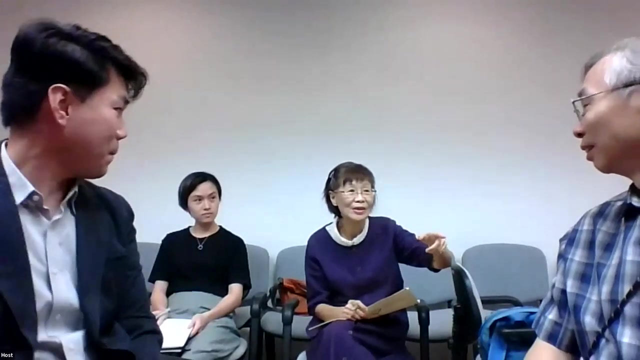 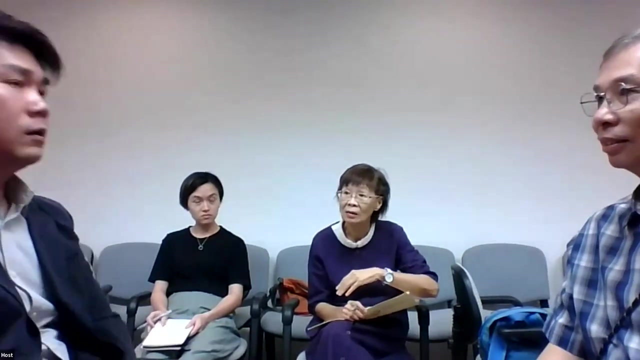 Some rare earth? yeah, Thank you. Okay, any more questions? Yes, Can I ask a question about the heavy and heavy research on how much yield is the factor? Oh, let me see, because for those heavy metal, mine, okay, I mean the soil with heavy metal. 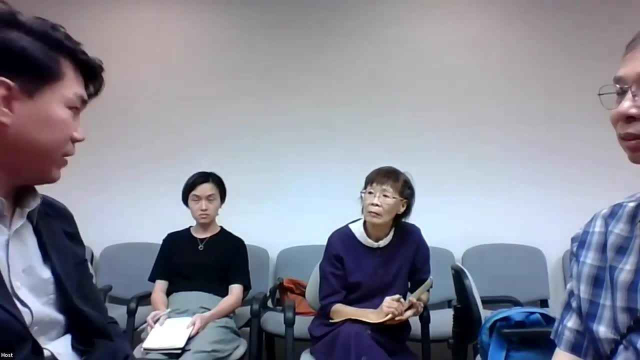 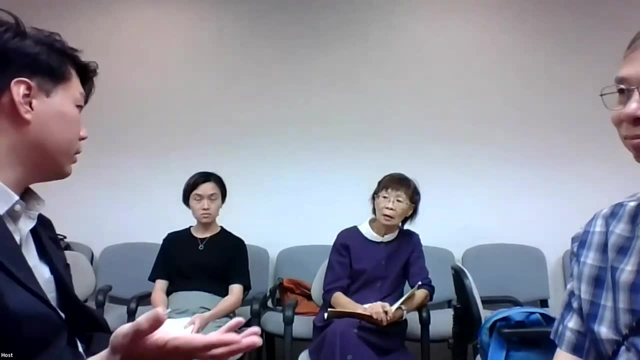 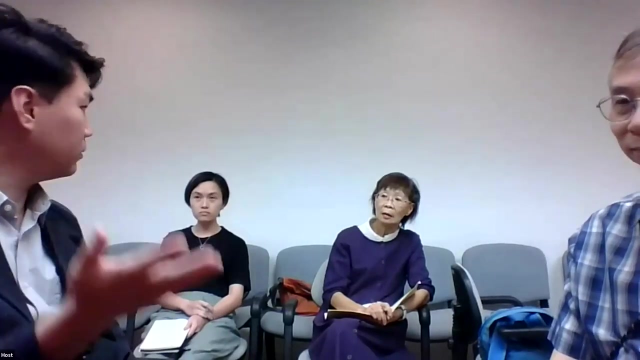 contamination, the yield is significantly being affected when compared to natural, basically. but once we add the biochar or the bacteria, we found that the yield didn't increase very, very much, not talking about first of all, but at least maybe 20 percent, 20 percent at least. but at the same time we are mainly concerned on the